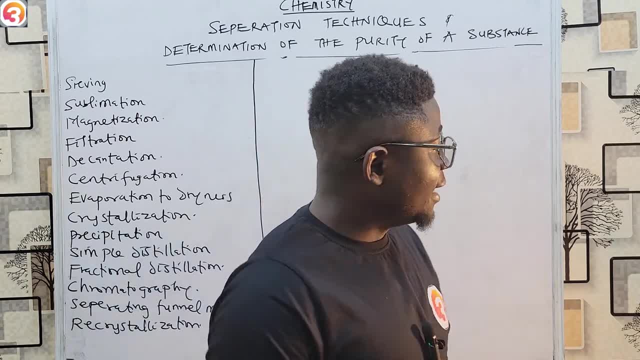 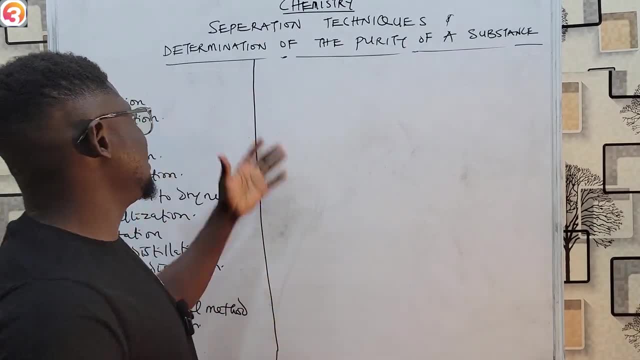 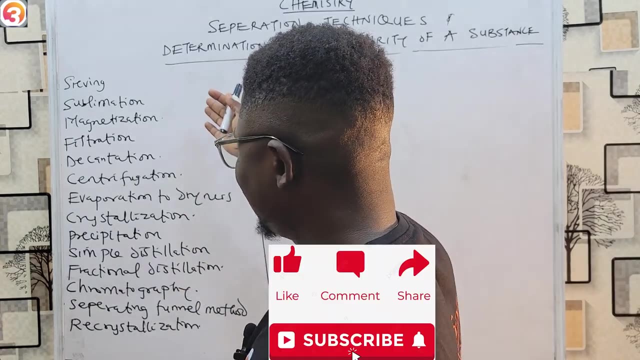 hello guys, and welcome to another chemistry class, and in this class i'm going to be looking at, uh, very obviously, separation techniques and the determination of the purity of a substance. that is just a side thing, right? so these are the separation techniques are going to be looking at. 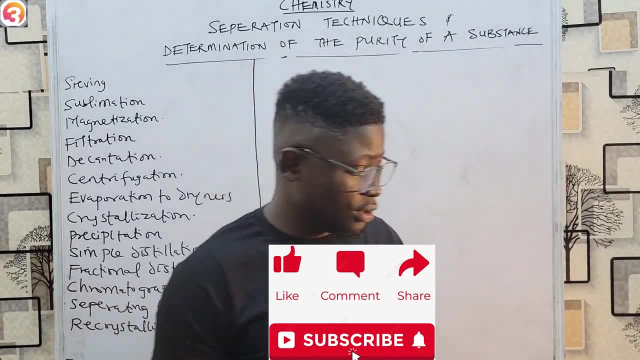 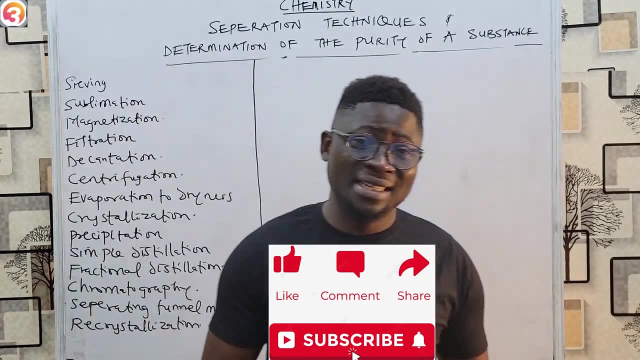 but i'm going to be looking at, uh, what they are, and then, of course, we are going to explain to you, uh, several ways they can come out in the examinations. it is very important and pertinent that you watch this video to the end. a lot of you watch two minutes of a video that is over 30. 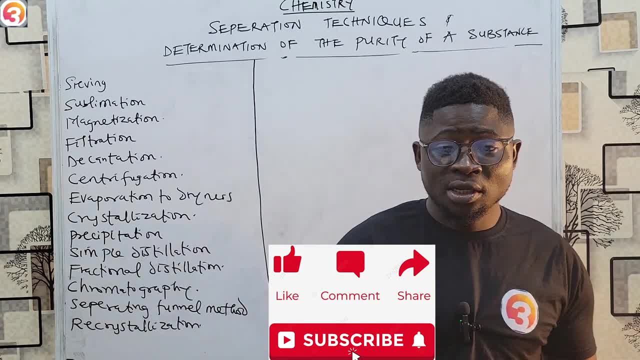 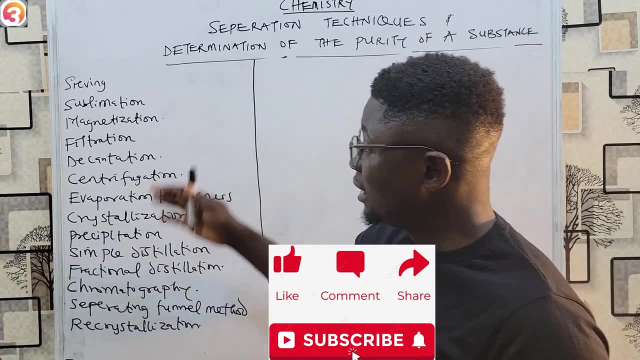 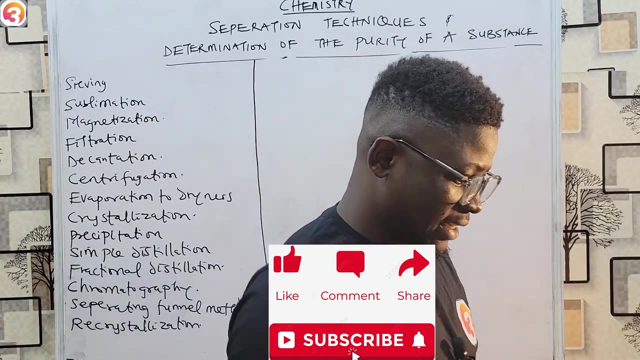 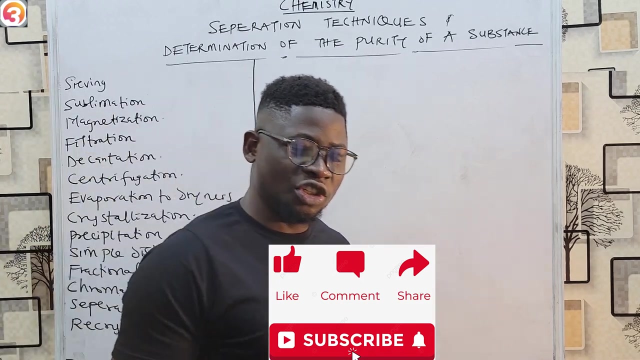 minutes, and then you think you have known everything about the video. well, that is your choice. that's your choice, basically. but make sure, please, that you learn everything about the separation techniques, because you do not know where jam is set that question from in separation techniques, right? so, uh, we have said before now that, um, the constituent of mischief. 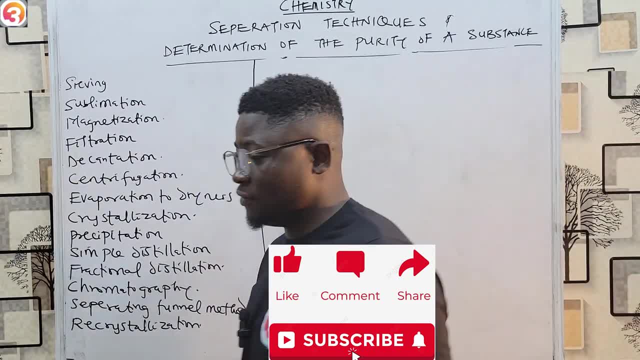 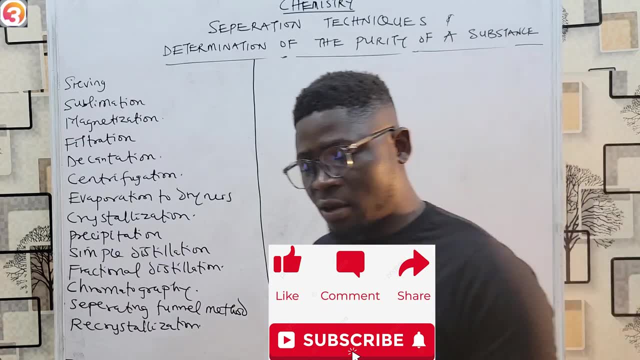 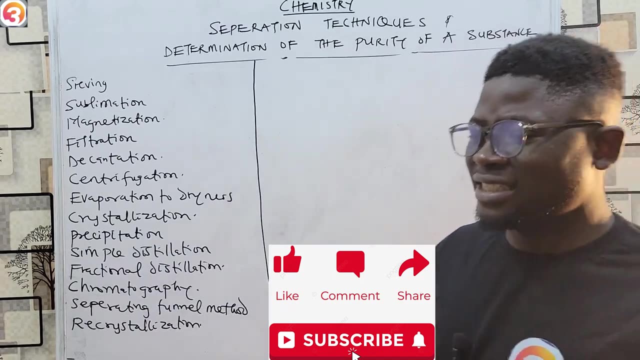 can be separated by physical means in the last class- if you have not watched that class, please go and watch it- on elements, compounds and mixture. look for it in this channel and watch it right? so i'll say: the constituent of mixtures can be separated by physical means and that is why we 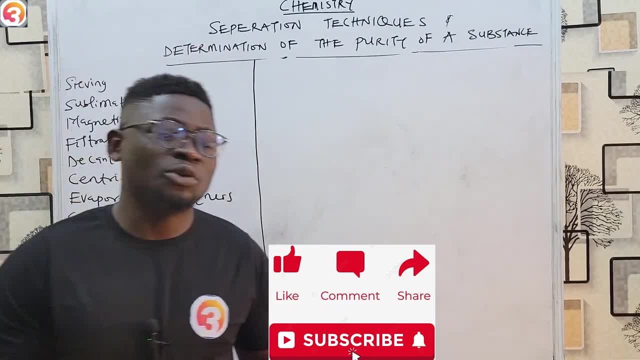 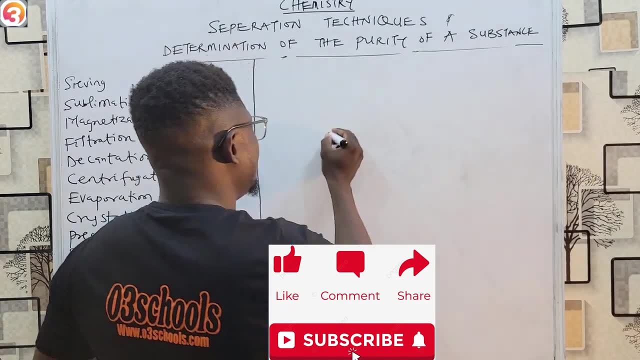 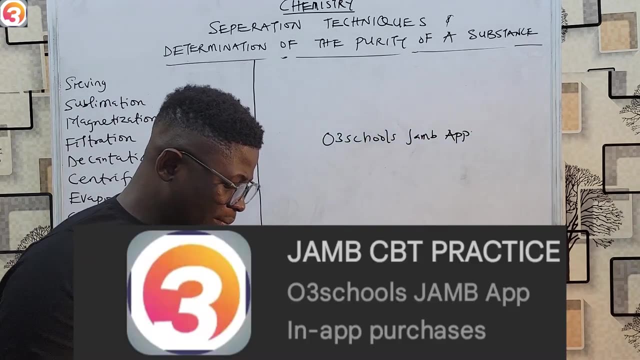 are discussing about separation techniques. what are those ways we can separate mischiefs, right? so, uh, do not forget, of course, that this class is brought to you by the old tourist schools. jam app- all three schools jam application- is the best cbt practice app available out there. 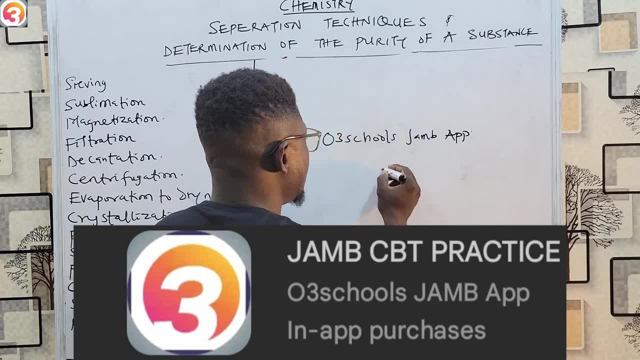 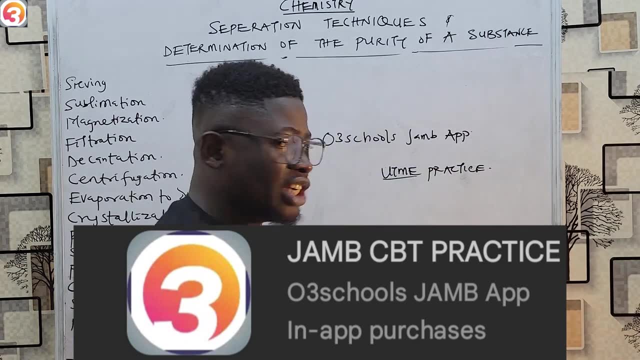 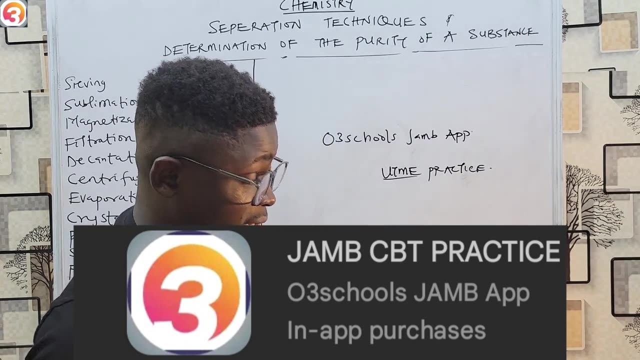 it has all the jump past questions under the utme practice session. utme practice: you know you don't write jump, you write utme. so a lot of you make the misconception: ah, my jump exam is utme, you are writing web job. well, you could say jump do, because jump is the body. 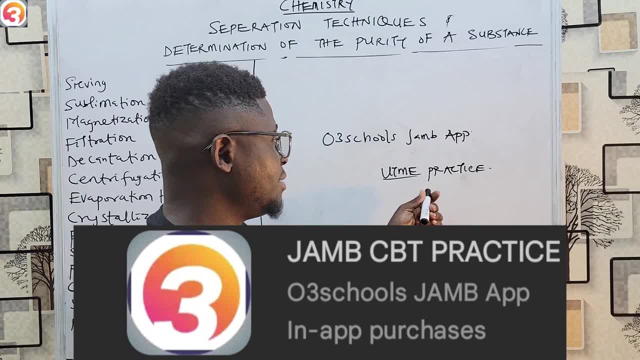 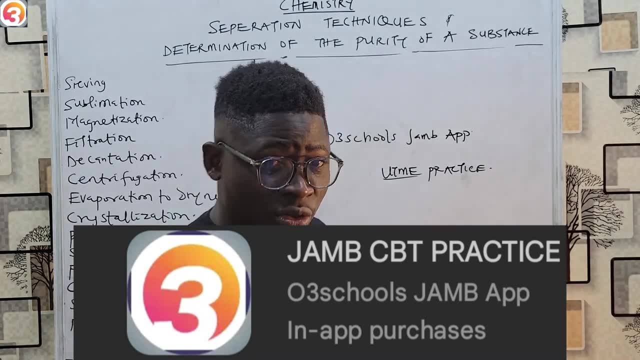 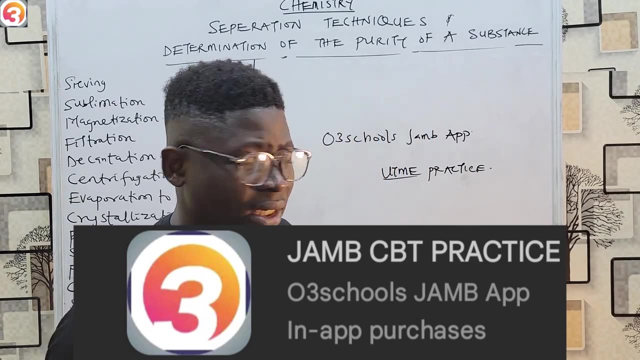 according with the exam you're writing is utme. so one day the utm practice is where you find all the past questions on the app up to date, right? so of course it has all the past questions for all subjects. for all subjects it also has likely questions that will come out in your exam. that is. 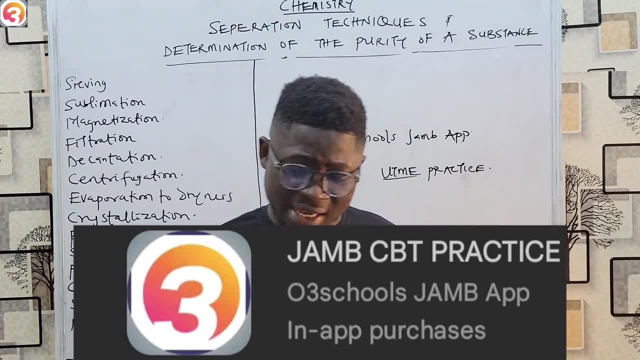 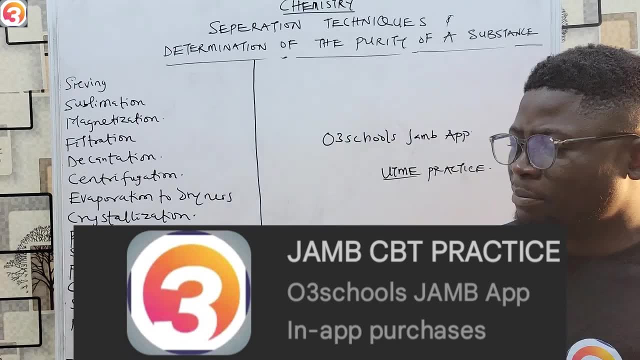 why you should not play with this app. all questions on the app have been carefully explained, the reasons for the answers i'm carefully giving, and that is why you must launch into this app likewise to see. they say there's a utm challenge every saturday to test your preparedness for the exam. 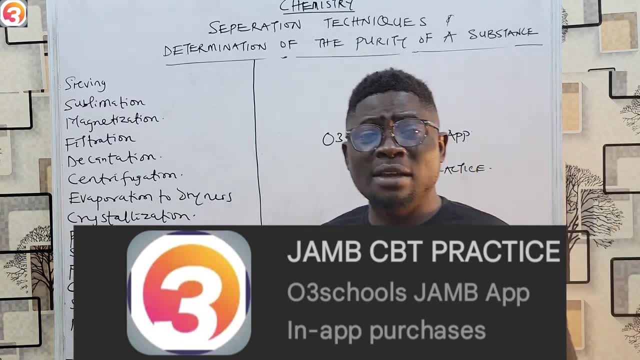 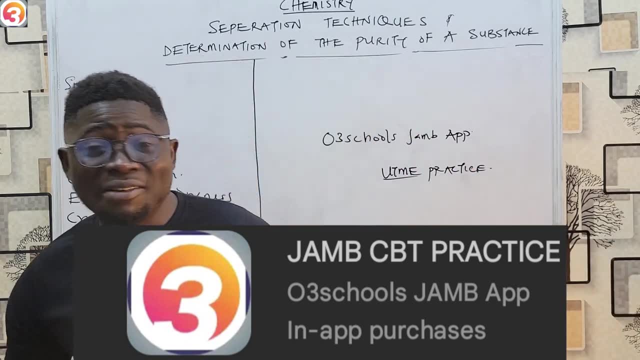 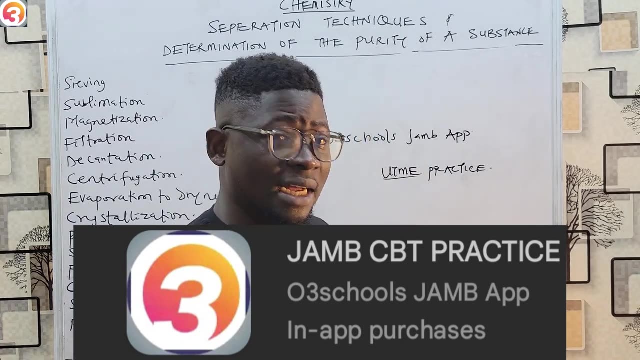 to see how prepared you are to test yourself. it's a mock challenge every saturday and people win prizes. we share up to 43 000 era in prizes every challenge day, so you can get your activation feedback through. that means well. so the app is- uh, it's not free. the free version allows you to. 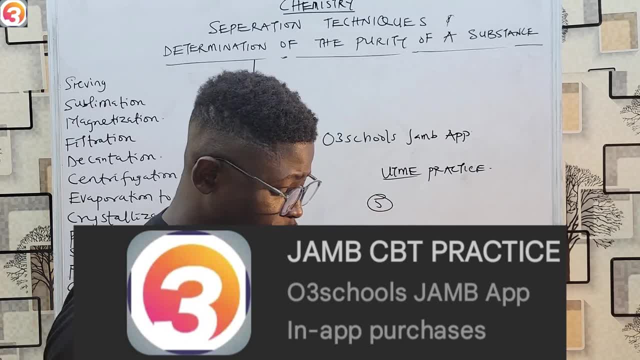 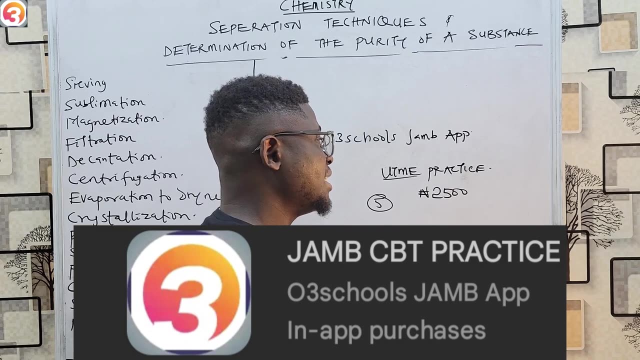 answer just five questions. after five questions, you'll be told to activate and the activation fee is just 2500 naira. and in case you have trust issues that, ah, if i pay this money, will i get activated? of course you get activated, just simply send your payment proof or your receipts to zero. 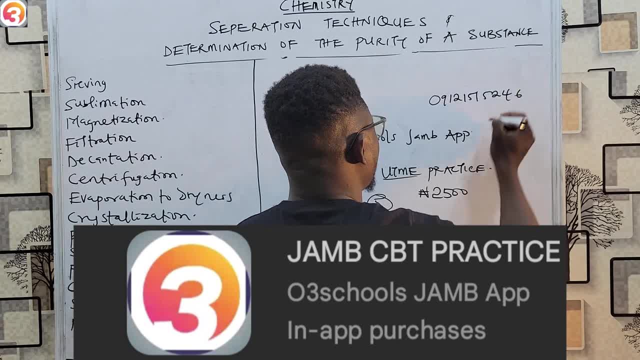 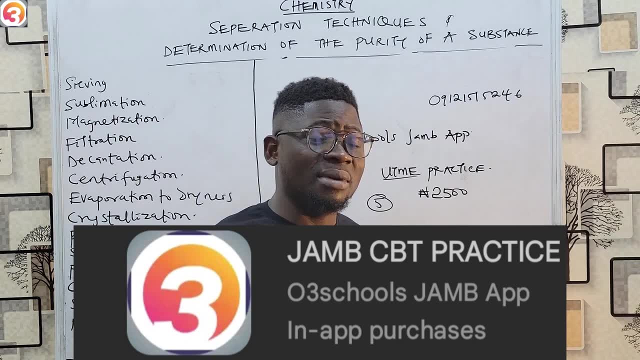 nine, one, two, one, five, one, five, two, four, six on whatsapp once you send your receipts, your payment receipts, right, your debit alert- a screenshot of a debit alert on your payment receipts to this number you'll be attended to. please be patient sometimes because i may be shooting this video and i will not be on my phone, so don't think you have been scammed at. 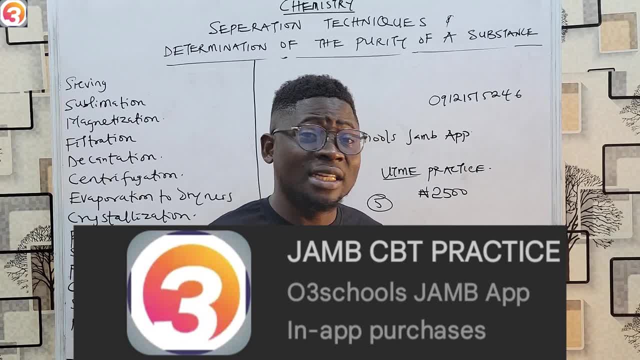 all you must definitely be attended to at least three the the the highest can be one hour and they have attended to. if, in case i've not attended to, just call the line too. it's our customer care number. call the line so an agent will pick it up. if you are too busy in the next one hour most. 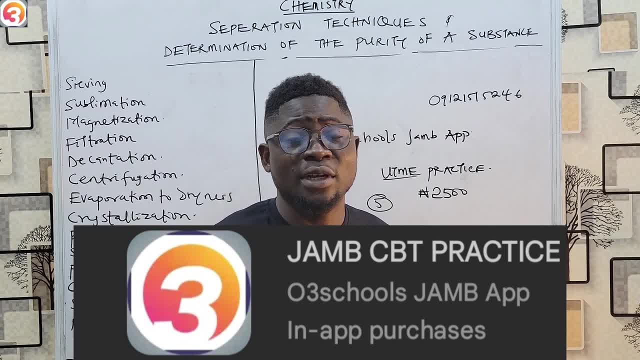 because we'll be in the studio to the shooting videos. you'll be able to get your activation key. well, that's, by the way, please get your app is very important. it's very necessary. you can also set mock exam for yourself to study. you can put it in the study mode, in the practice mode, in the uh mock mode. right, there are so many. 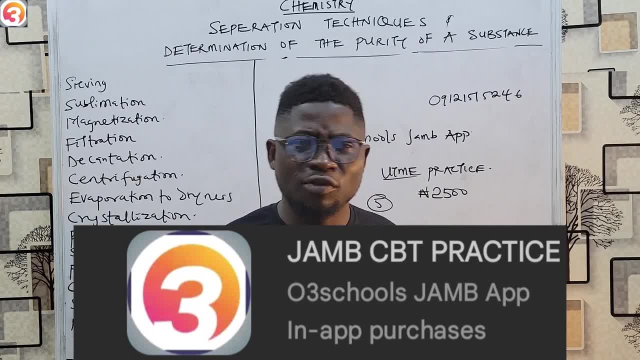 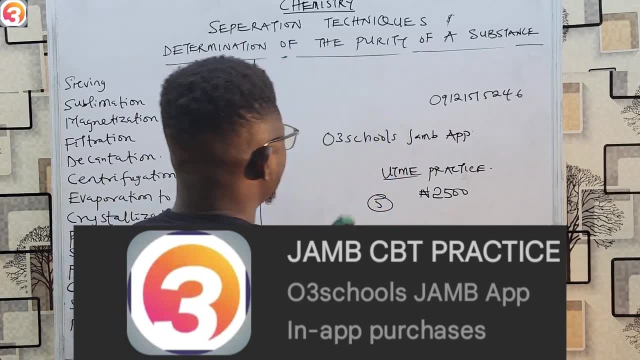 modes on the world. on the app, you can put it on random mode, where questions from different years will be thrown at you, right? so the app is very flexible for your using, all right. so today we're going to be quickly jumping into suppression techniques, and i've 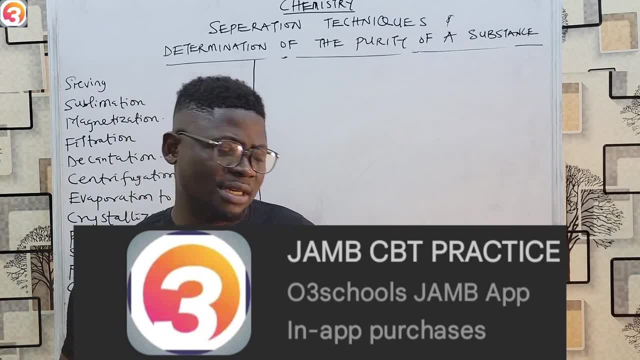 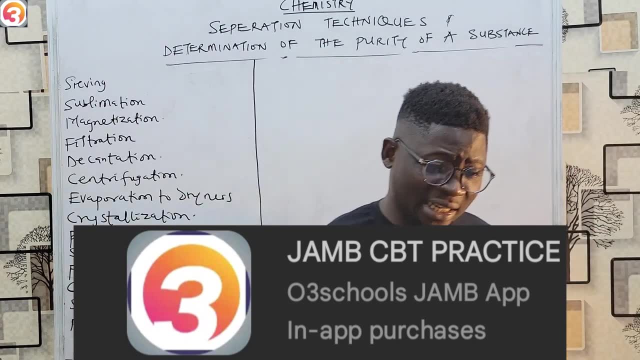 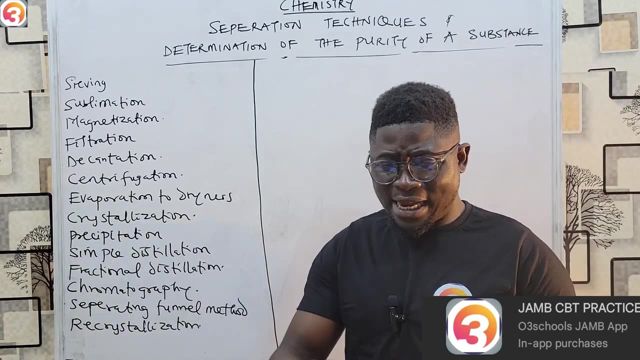 laid the foundation that constituents of mistress can be separated by physical means. so let's look at this: separation techniques for saving those of you that have been, that have seen where gary is made right. so you see that when that woman, that man, holds one that looks like a basket, that has small 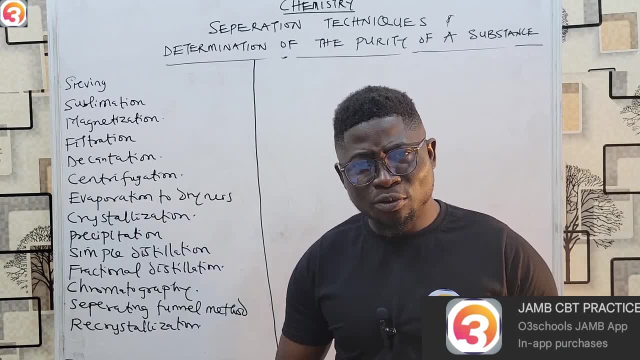 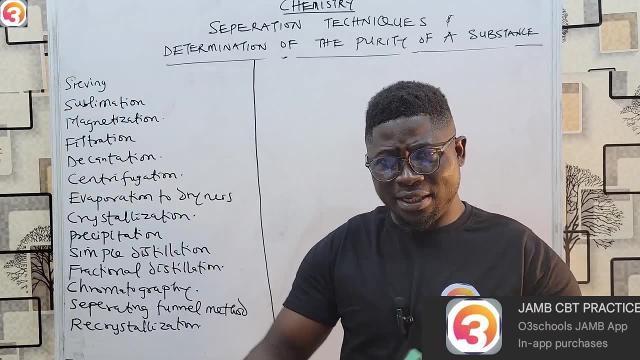 small inside. she'll be shaking it like this so that the smaller particles will be what will be dropping on inside the rubber she's shaking why the big up lumps will stay at the top of the of the name of that thing they're using in separating it right. so that is saving. that's what the woman. 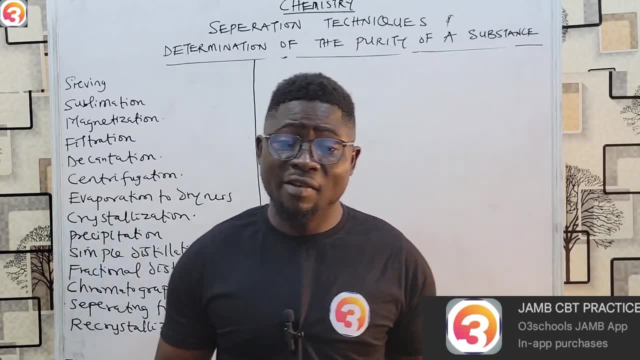 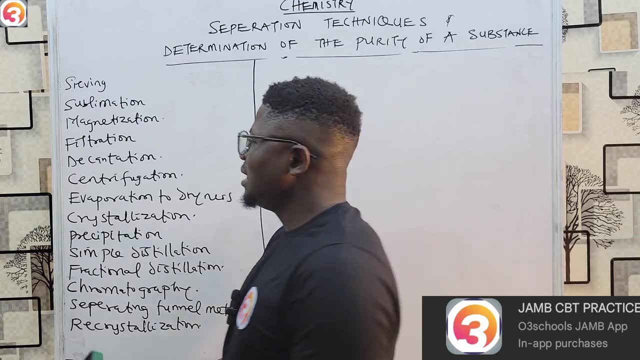 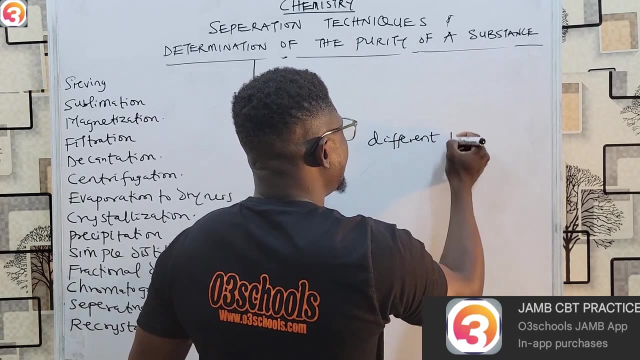 is doing, she's saving. so my fear avoiding fried gary before me. i've been weird. gary was fired before. i've also fried small gary too, so right, so that is saving. saving is used to separate what mixtures of what different particle sizes. different particle particle sizes. 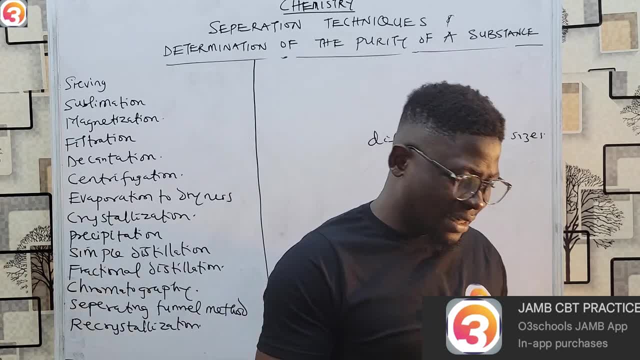 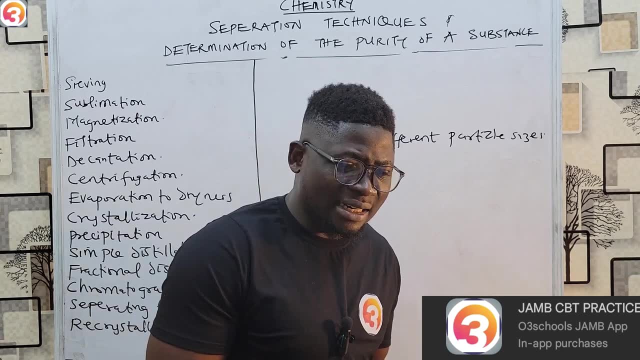 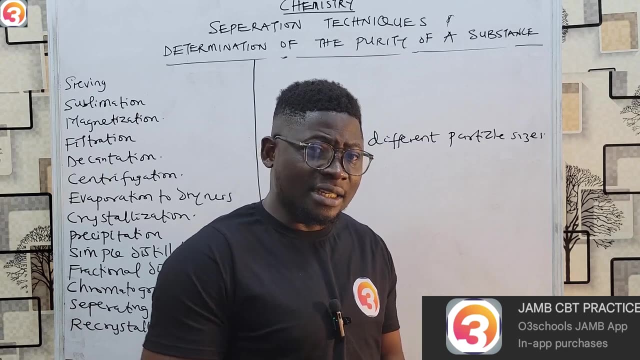 it is a word for separating what mixtures of what different particle sizes, such as the mixture of what like that that we're talking about just now, the garrison right, or mixture for sand and the stone right. when you have sand and stone there are four different sizes- right, you can easily wash, sieve what, the, uh, the, the sand out and leave the. 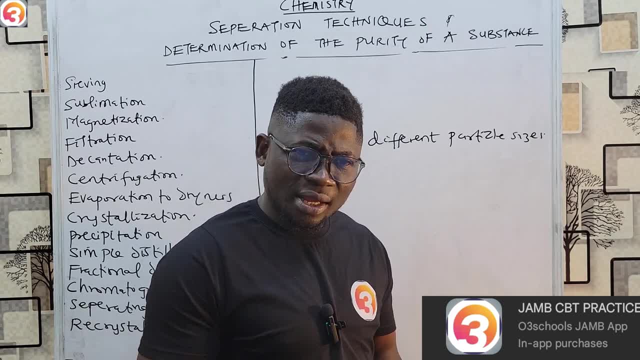 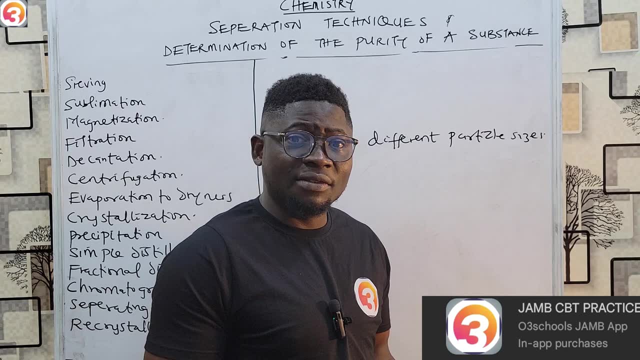 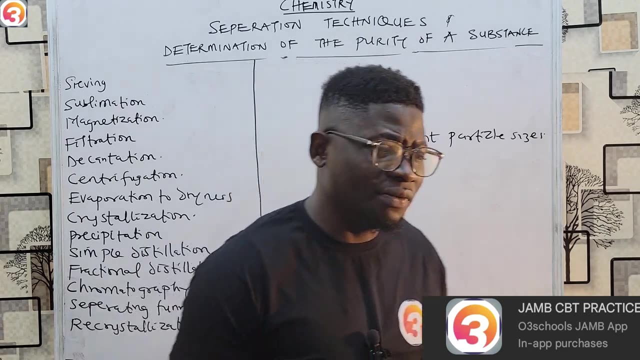 stone at the top right. so that is what. that is what uh, uh sieving. also, uh, what about uh, a gary, gary and uh and sand? they're different, that the gary and sand are different, that they have different sizes depending on the sizes of the stand right. so that is what cv is used for: cv. 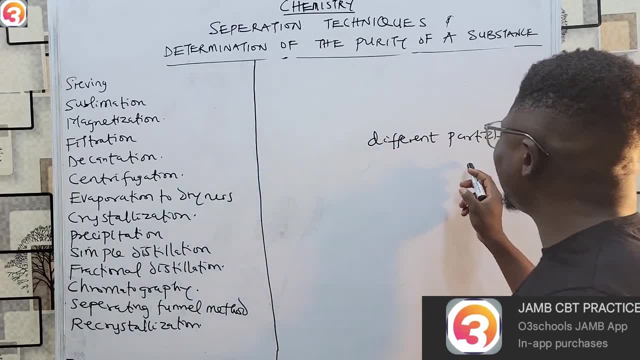 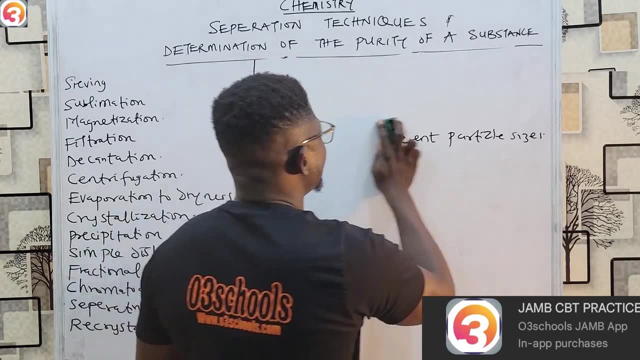 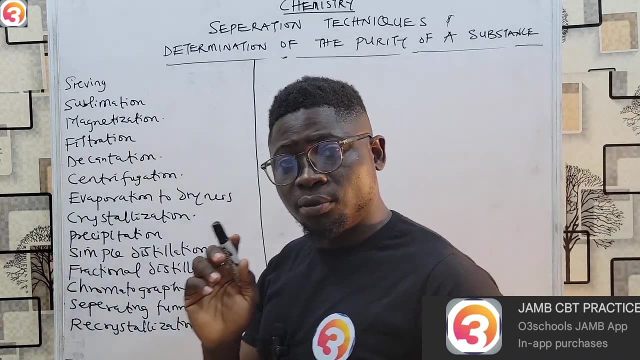 issues for what to separate mixtures of different particle sizes. it's used to what to separate mixtures of four different particle sizes and francine sieving will go to sublimation. when we're doing changes in matter, changes matter. we talked about sublimation. if you have not watched. 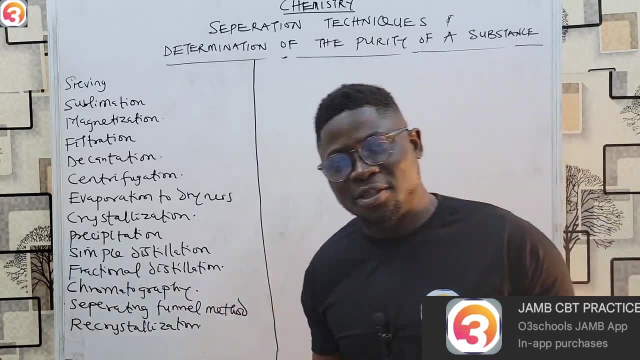 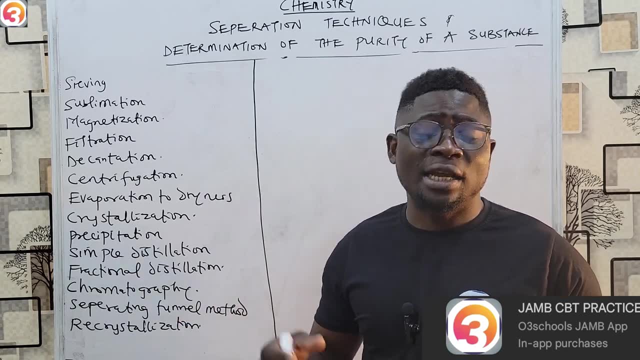 that video. please go and watch it. every video is a precursor to this one, so we are doing a step-by-step by episode to help you. in case you have not properly taught chemistry in your secondary school, right, this jump class will help you and build the foundation, so please do not miss any. 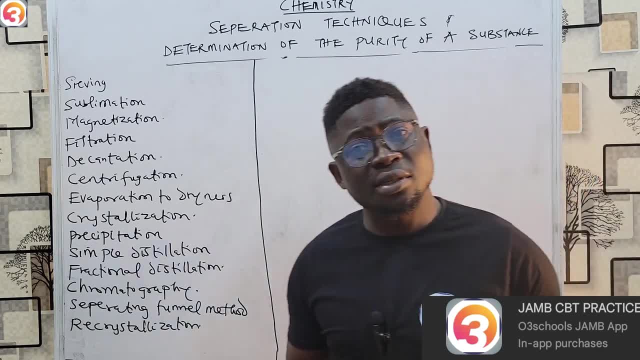 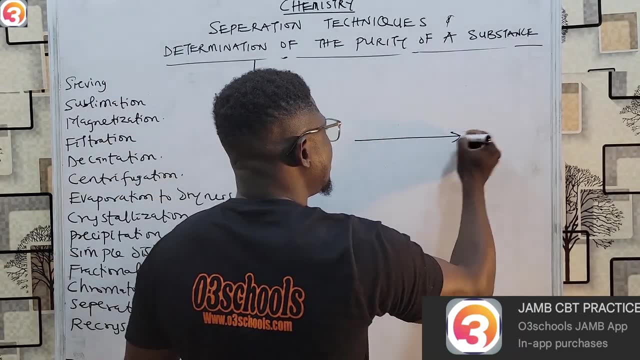 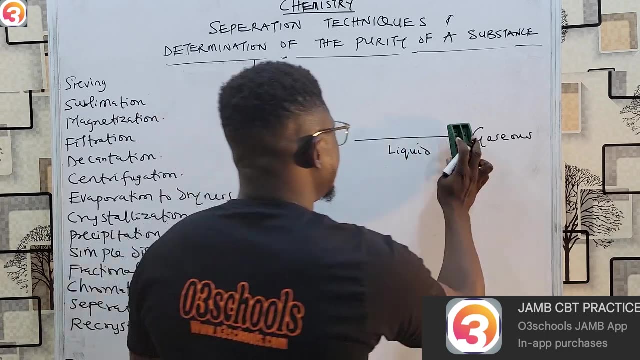 of our classes and do not watch half our videos, because you will do yourself right. so sublimation: we have said that when a solid can change directly to water, to the gaseous state. so we have solid, we have liquid before we now have gas. right, we have solid, we have liquid. 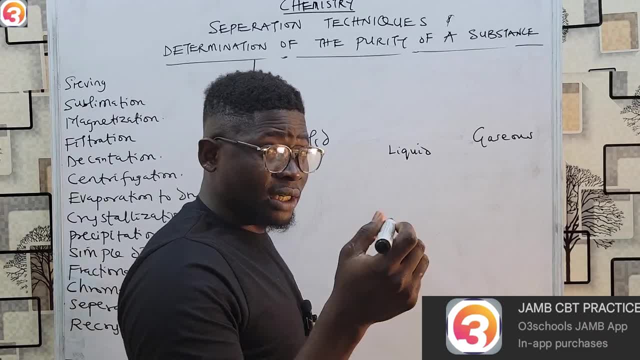 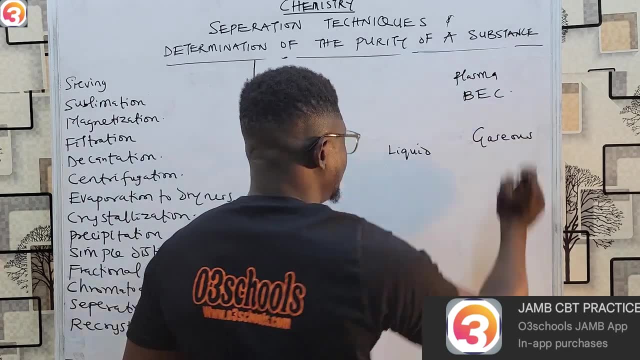 then we have gaseous water state. isn't it now so if we that we did changes in matter? we are other states, such as what the plasma states, and we have the bursar esteem condensate bec. this is theoretical in nature, like we said in that class. but these are the three words. 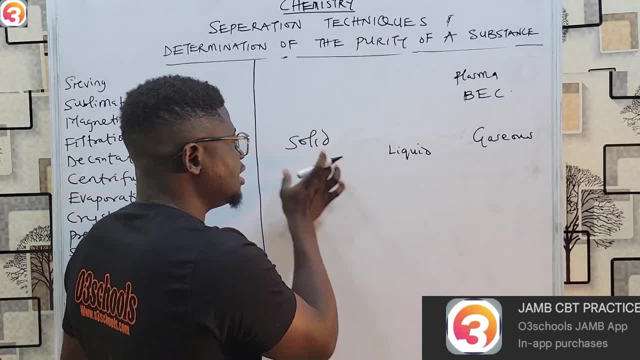 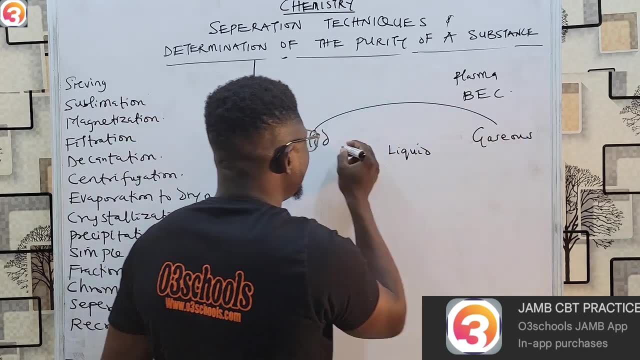 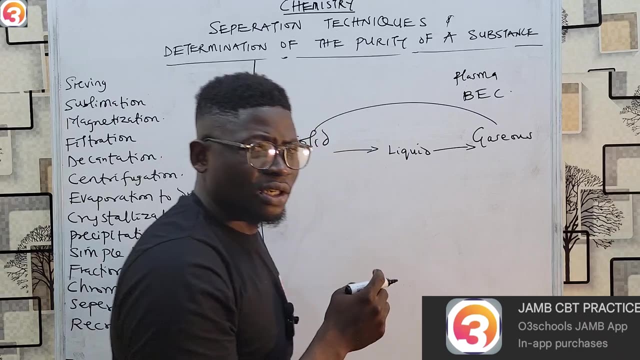 states, three most recognized state of matter. so we have solid, liquid and gas. now a solid can change from what? from the solid state directly, so from solid to liquid, from people to gas. but the solid can change directly to the gaseous states without passing through the. 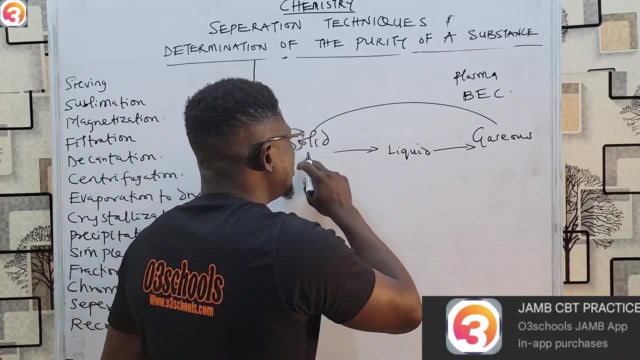 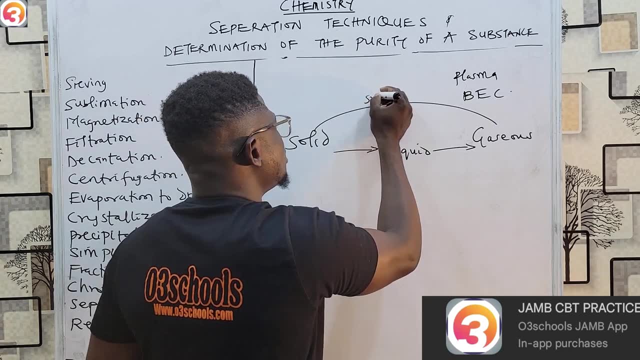 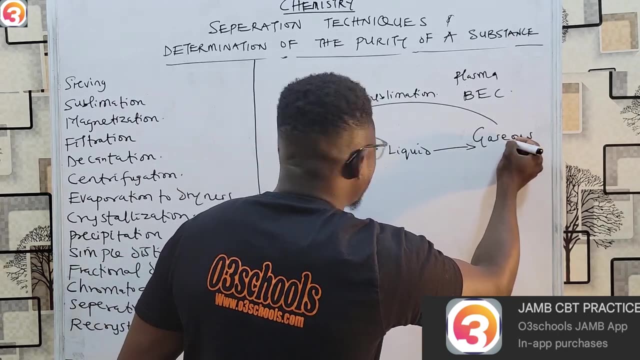 liquid states. the solid can change directly from what? from the a certain constant, directly from solid state to the gaseous state, without passing through liquid states, and we call that a process for sublimation. so that is what it's called and also say that it get a gas against your substance. 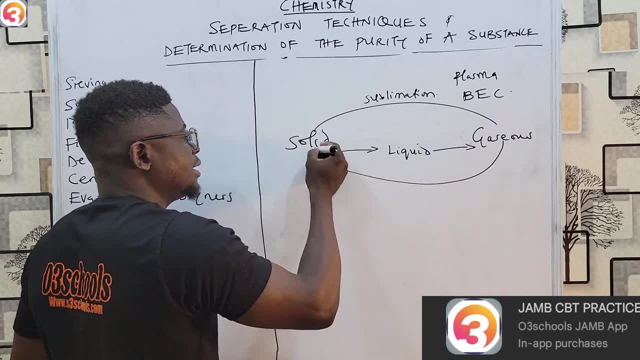 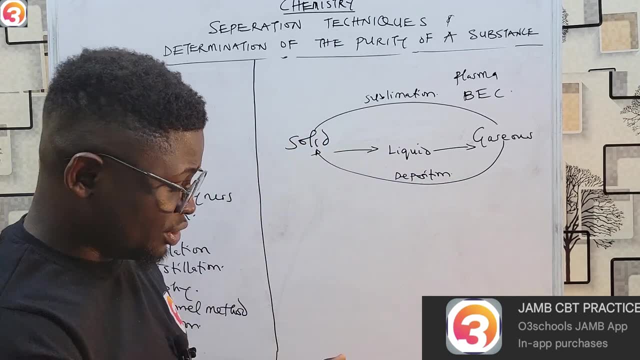 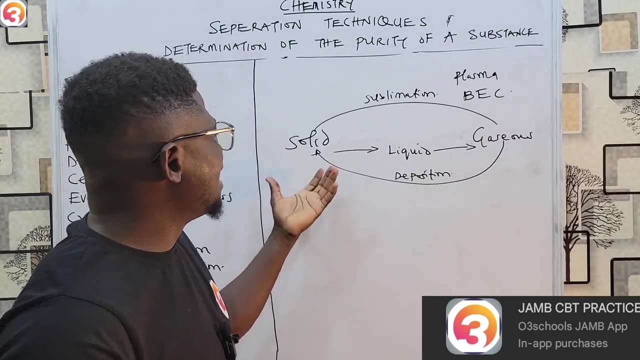 can turn directly to the solid without passing through the liquid state. right, i'll call that process what deposition, if you remember in that class gonna process the polish the position. so, and of course that means that sublimation is just a word, separate work, a substance that can change directly from the solid state to the 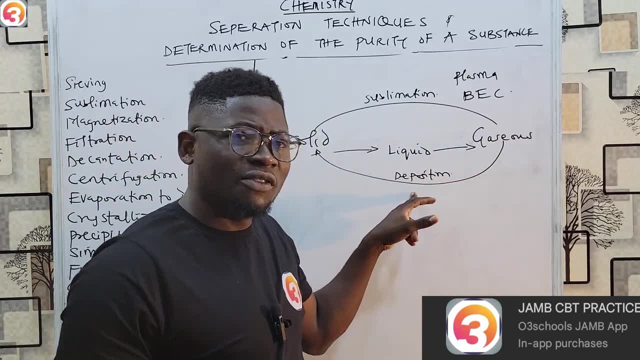 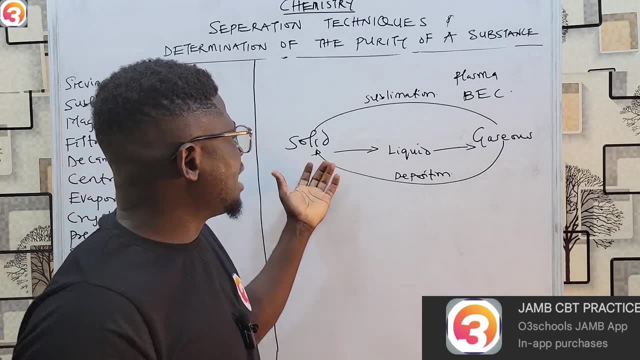 gaseous state without what passing through the world, the liquid state from the mixture of this word. solution. so if you have a mixture of a substance that can sublime with another substance, right that means we can simply was sublime what that substance, away from the nature, leaving the 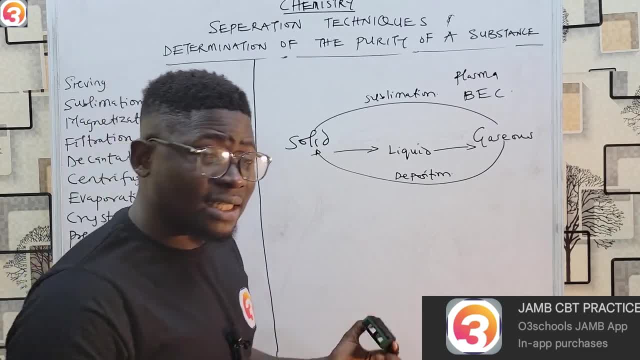 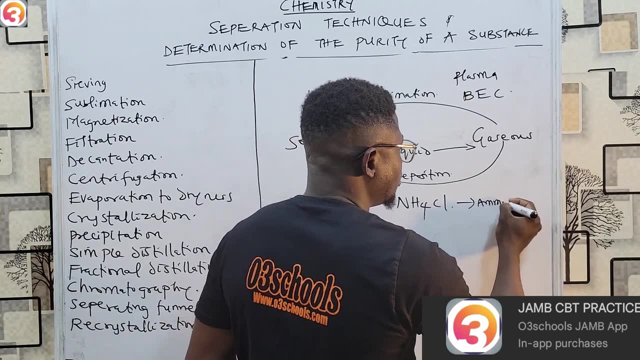 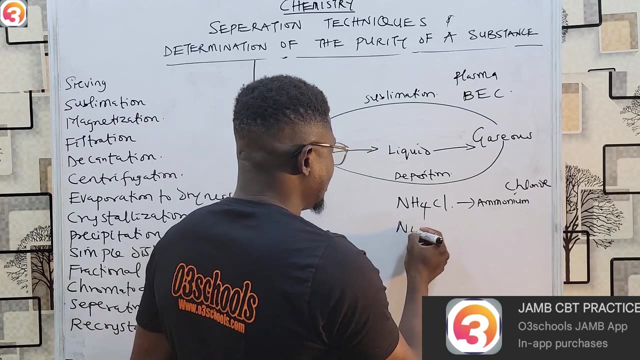 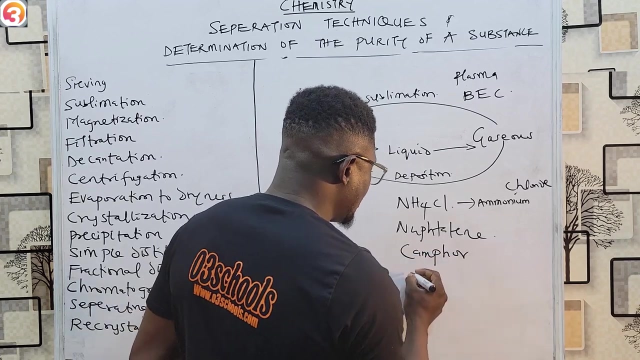 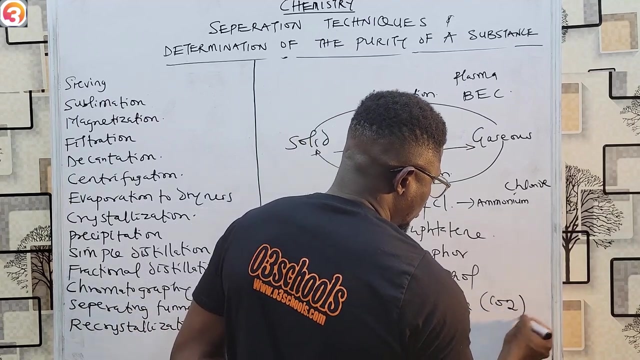 other mixture there, right? so there are several examples of substances that can sublime, like one we have, nh4cl. this is what ammonium chloride- ammonium chloride can sublime. then we'll talk about naphthalene- naphthalene, right. we'll talk about camphor, talk about menthol, talk about dry ice- right. dry ice, right. so 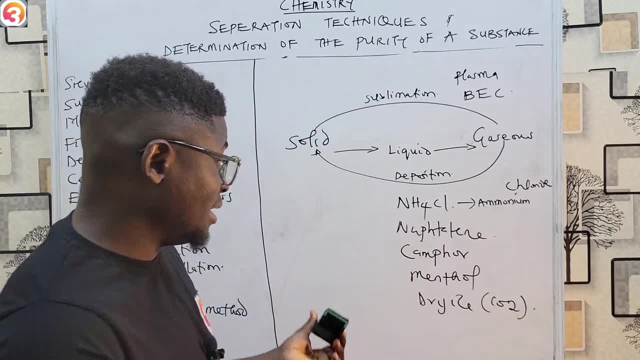 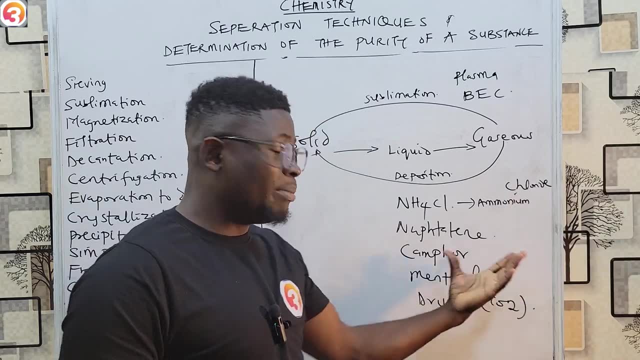 many other substances that can sublime, but these are the major ones that, at least at this stage, we should be familiar with. right, this substance, they can change from the solid state directly to the gaseous state. remember this in past questions. right, which are the following is: which are the? 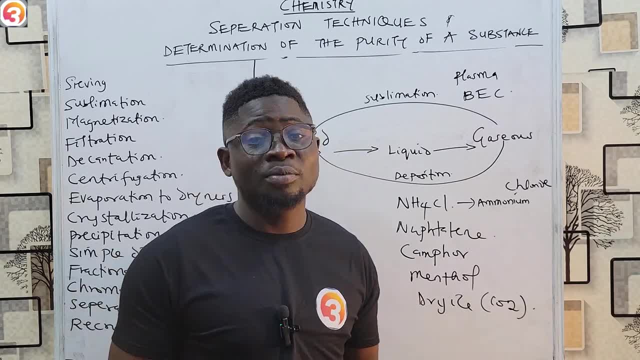 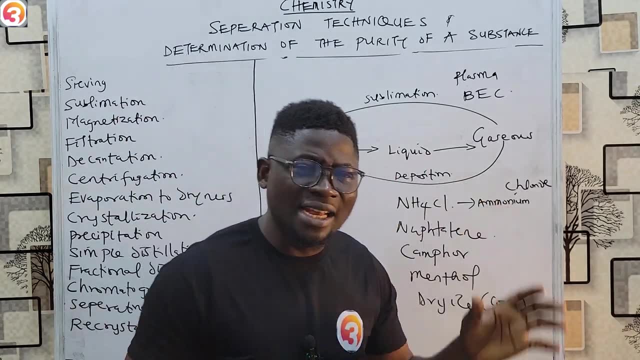 following: substances cannot sublime. so if you know this, it will help you a long way, right? so please take note of this substance that can sublime. so this is what sublimation is used for: so you can easily was sublime. that's something that can work. i can undergo sublimation and then leave the other. 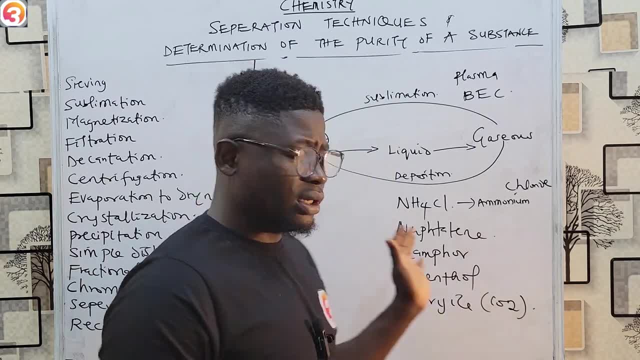 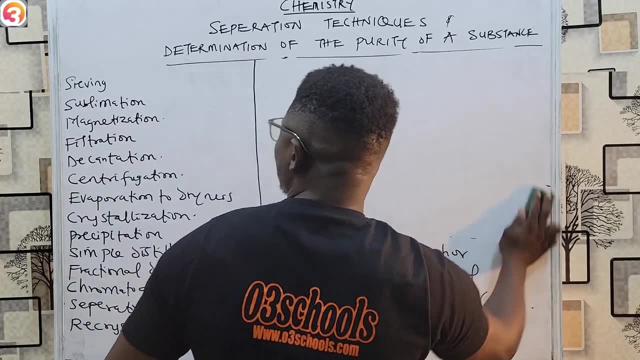 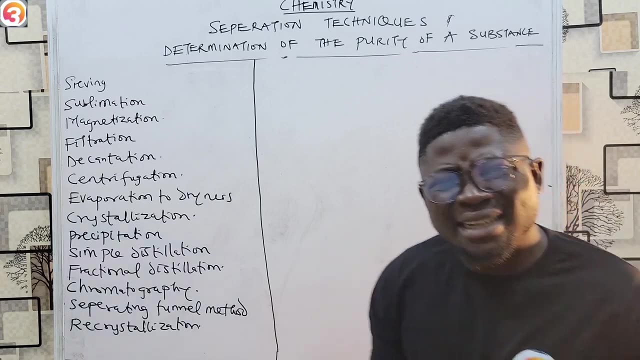 substances in the mixture so you'll be able to work carefully with separate using sublimation. so please take note of these substances that can sublime. so we'll go to the third one, and that is magnetization. magnetization is used for separating what magnetic substances from non-magnetic ones. so 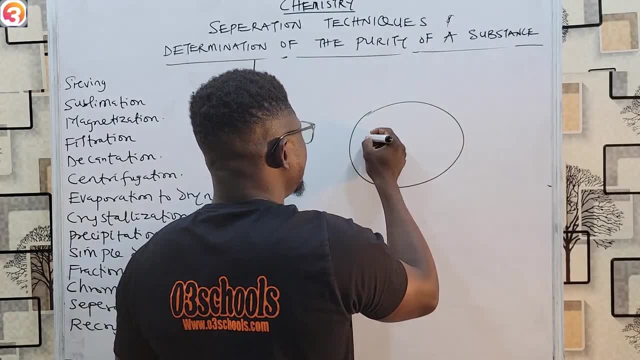 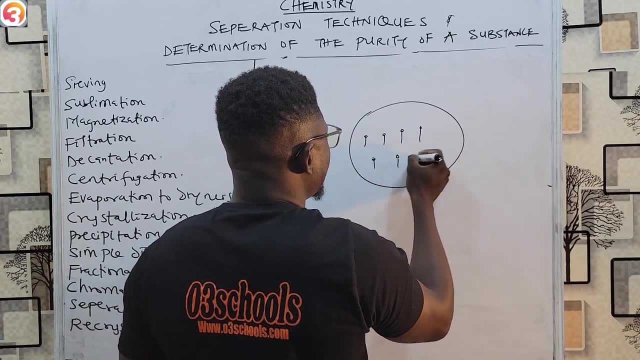 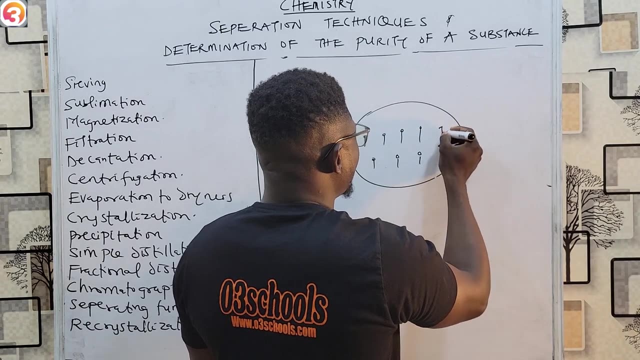 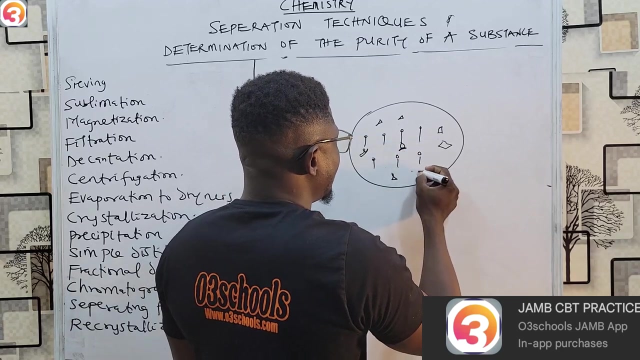 let's say you have a bowl here. you guys say nails, nails. this is near, i don't know. let's say this is me, yeah, yeah. and then let's say there's plastic. maybe some caught plastics and uncut plastics. there's a plastic, you know, like all those workmen that have different things, like 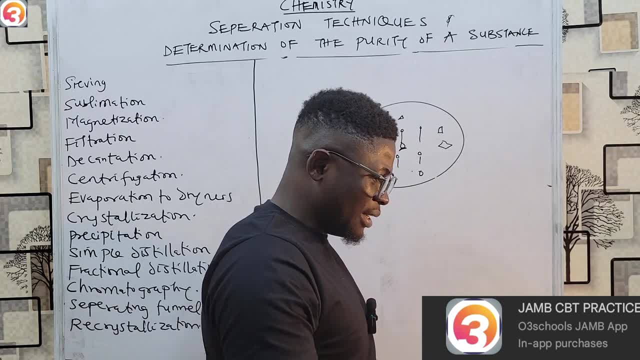 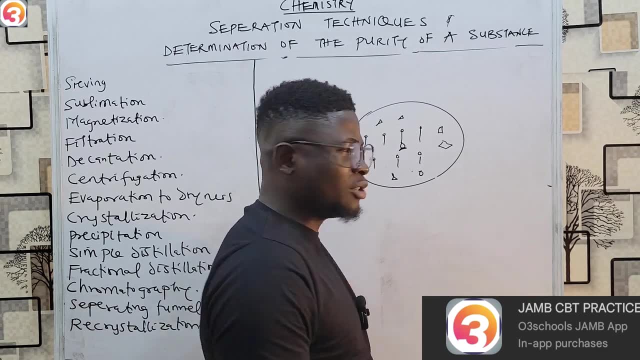 if you see an electrician's bag now, they'll be nailed or hammered. there will be a different, different, different plastic, other things they're using in putting holes on the wall and putting inside. there will be so many of them inside. so, but a, a walkman maybe job, let's say a walkman. 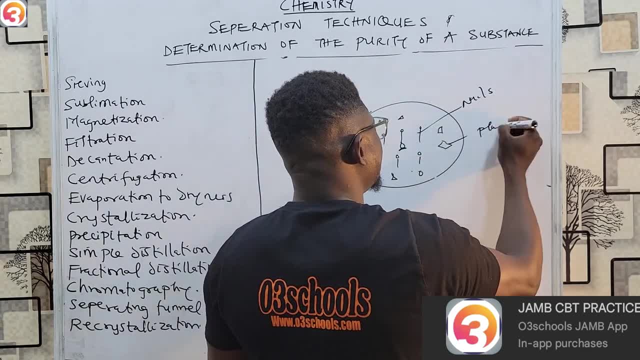 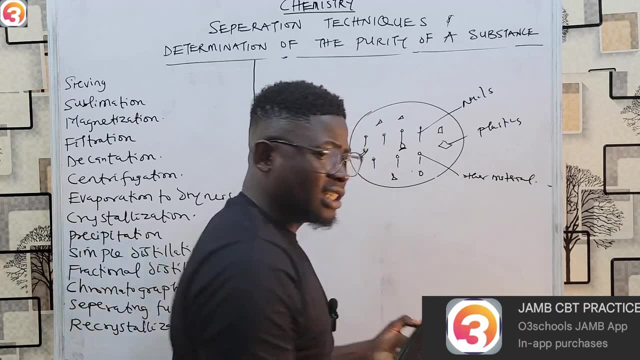 say: this is nails, these are yield strata and this this out plastics, and then then- this punto lesser- the other other materials that are not magnetizable. so what the workman can easily do is to carry a piece of magnets close to this. is what this bag. 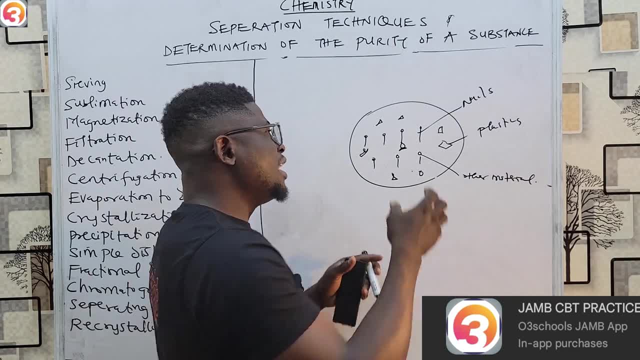 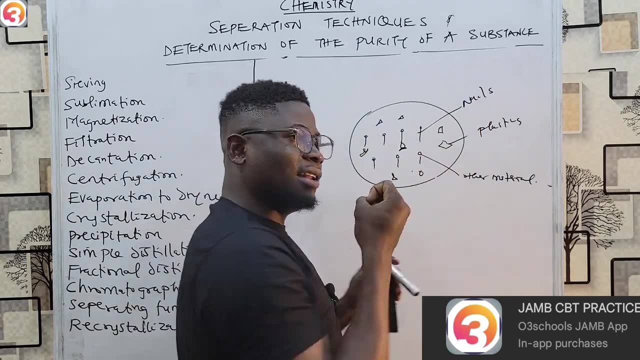 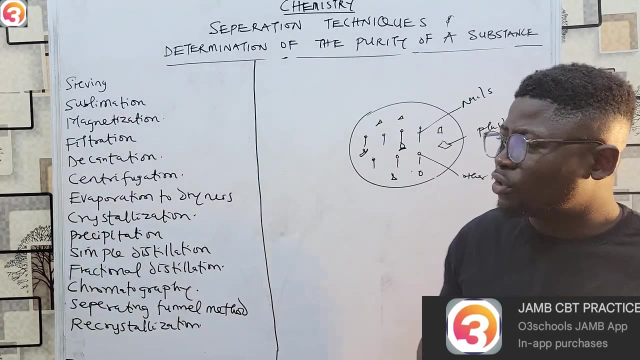 adds contact has for these different materials in it. so if he wants a nail, of course know that a nail is an iron right that it can magnetize. so the magnet will magnetize the nail for him right, leaving these ones inside. so magnetization is used for what? for separating what magnetic substances. 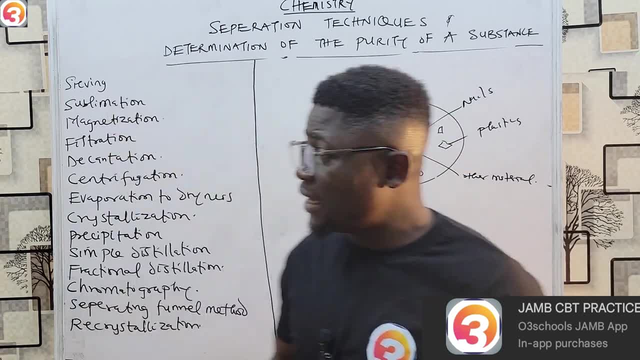 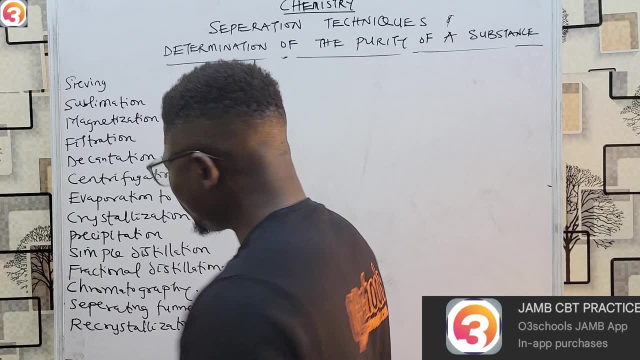 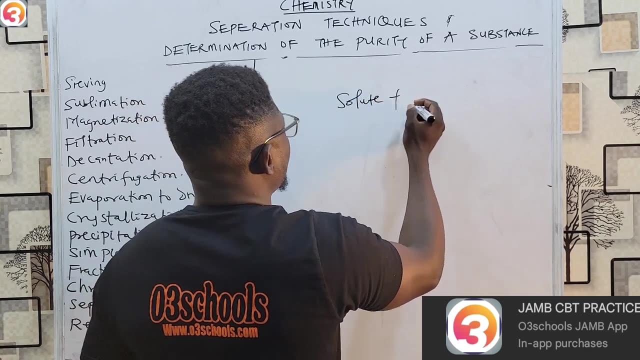 or magnetic materials from non-magnetic ones. it's very, very easy. there's not much to talk about about magnetization apart from that. so of course, we have the filtration. filtration, before we start talking about filtration, know that what a solute plus what solvent gives us was solution, i think. 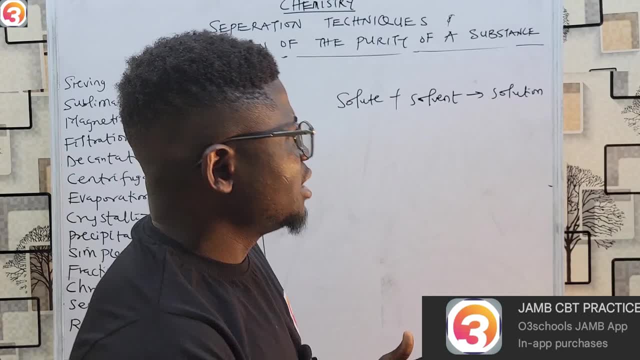 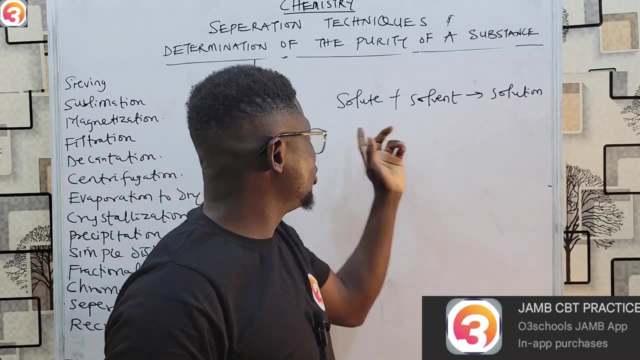 this would be about the first thing we thought in chemistry, right, right. so so it's so much. we dissolve in a solvent, so give what a solution. so what is a solvent? the solvent is like a liquid that the solute dissolves in. right, why, you saw the solute? what is what dissolves in the water? 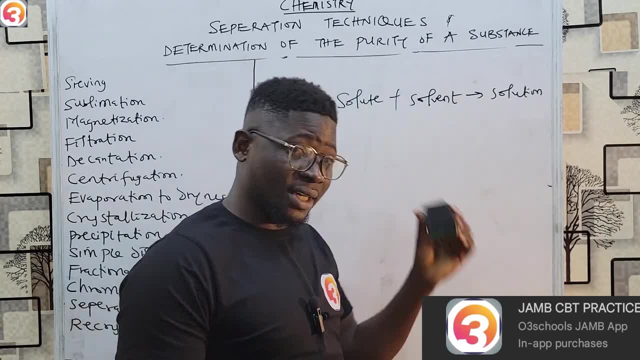 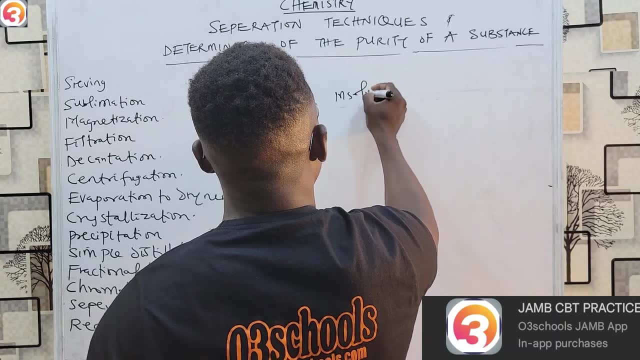 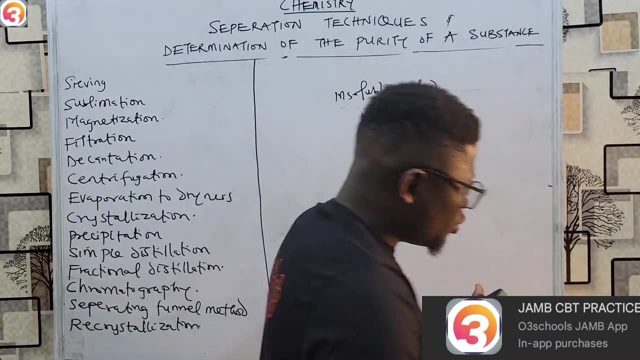 in the solvent will give us a solution. so you must just know this right by the, by the wayside. so a fit filtration is used for separating an insoluble, solid and what and a liquid right, so what you want to separate: what an insoluble, what solid and. 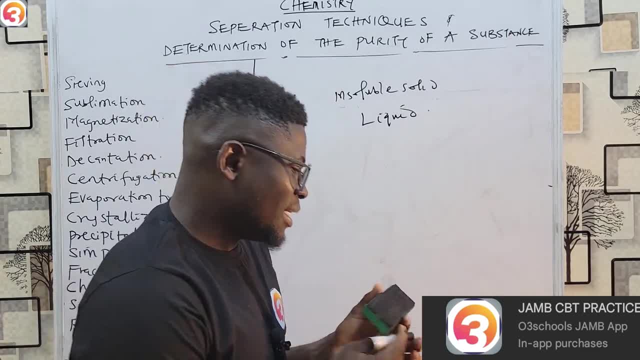 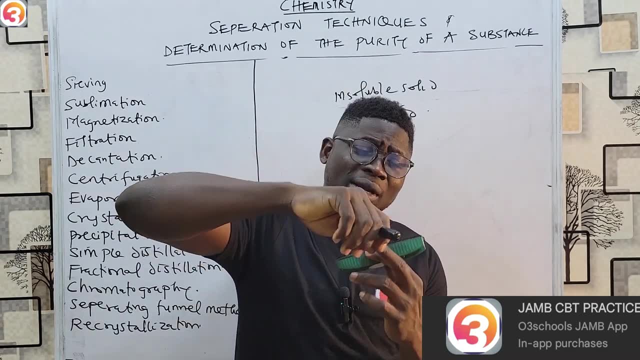 liquid, you use what filtration method, for example, let me make a good example. i don't know if any of you have. i've seen that lifting tea, right, that lifting tea, right, that very, very popular lifting tea. so let's say, for example, you want to drink lifting lifting, then you take what one? 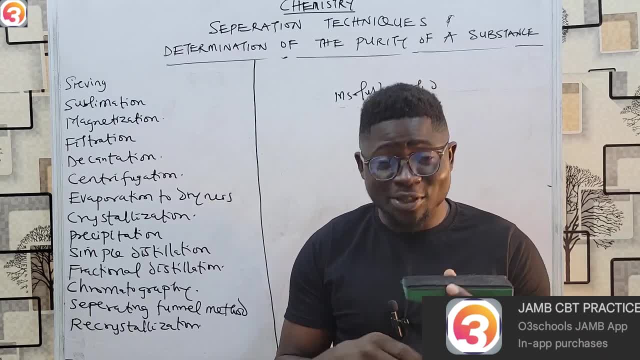 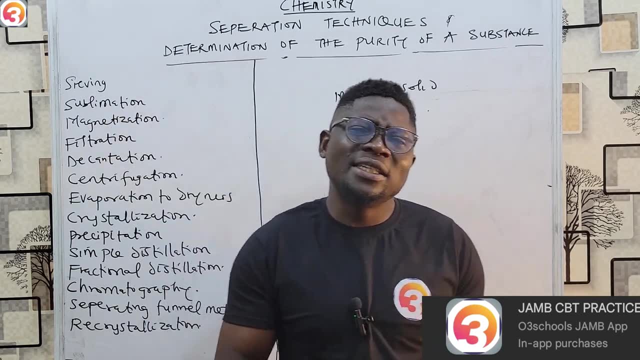 of that thing and put inside your kettle to boil, so that most of you say, so that the thing will come out the other way, right, that kind of thing. so once you put that inside the kettle and start boiling it, sometimes the, the, uh, the bag, the bag holding those particles may just burst and pour. 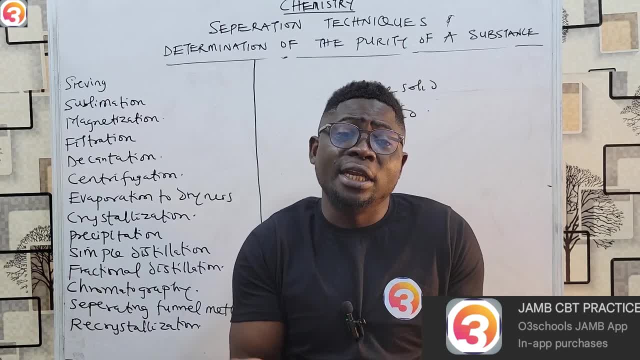 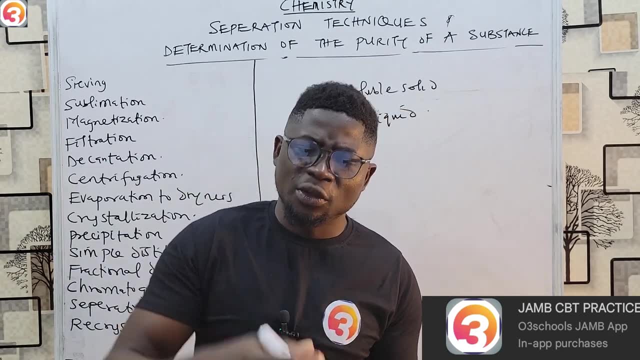 inside the kettle. so but let's say, for example, you don't have money to what, so go and get another one. what you simply do is to what is to separate all those particles from the world, from the liquid right. so you can take a filter paper, make a filter. 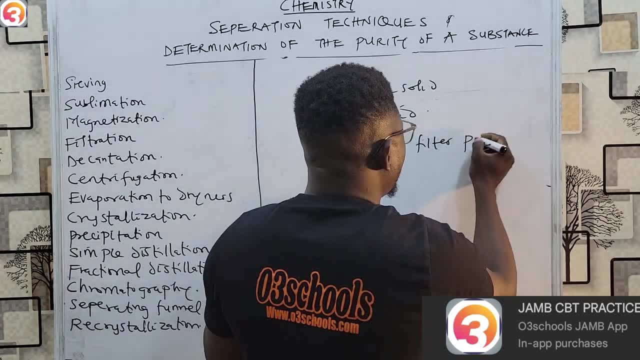 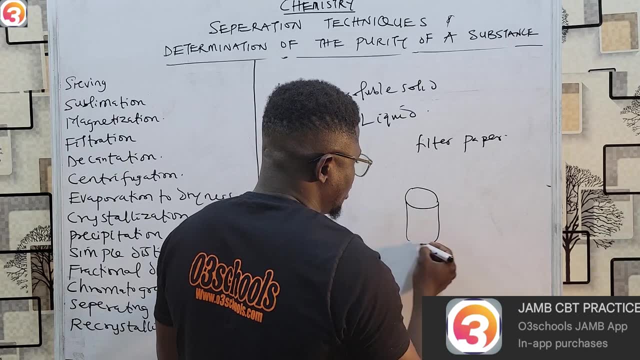 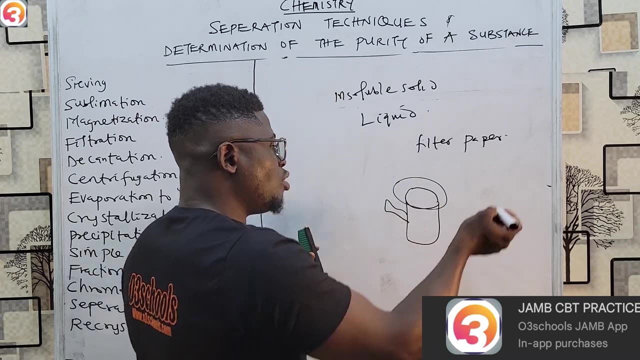 paper or a filter, a filter paper or a filter. and then you place it over a cup. let's say this is a cup- don't mind my drawing of a cup, i'm very, very terrible at drawing rest. let's say this is a cup, then you put your filter paper on top of it, right? so you pour your, what your, your the liquid. 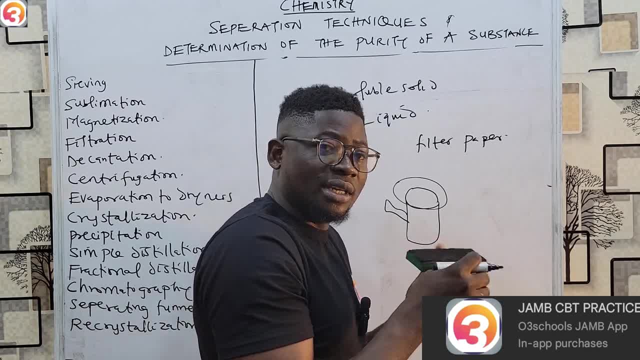 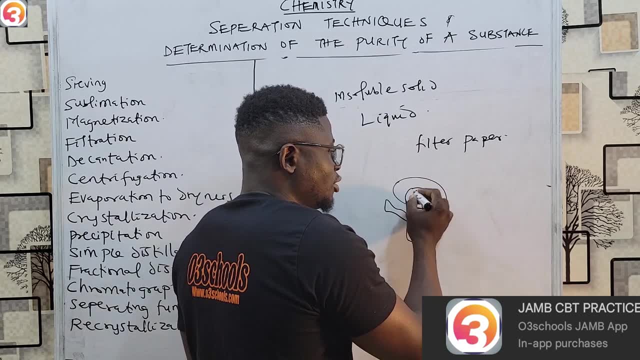 containing both the words, both those particles and the liquid from the kettle. you pour it on top so that the liquid water will come down into the cup. why those smells not coming out? so those particles will stay on top of the world, on top of the filter paper. i understand. 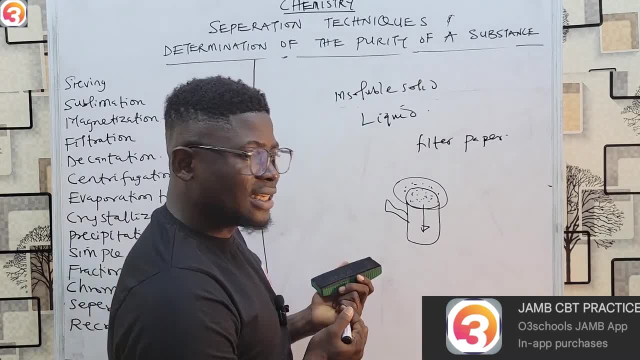 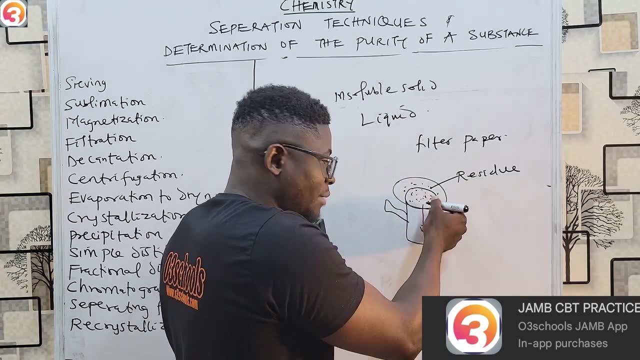 so that is filtration. you have carried out filtration. so what are you doing? in this case? these particles are still on top. they are called what the residue? why the liquid? that what that passes through the filter paper into the cup. we call the world the filter it. so that is what you. 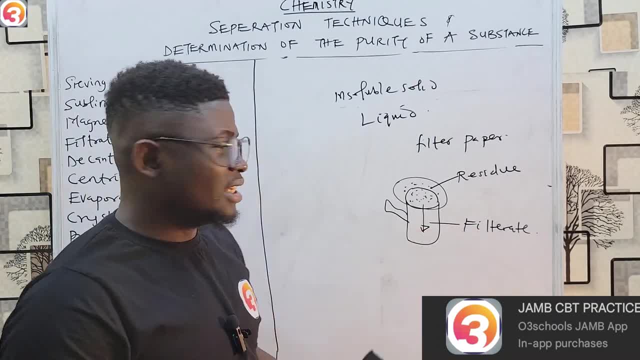 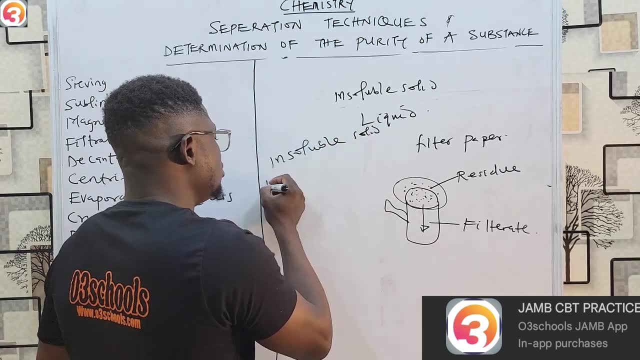 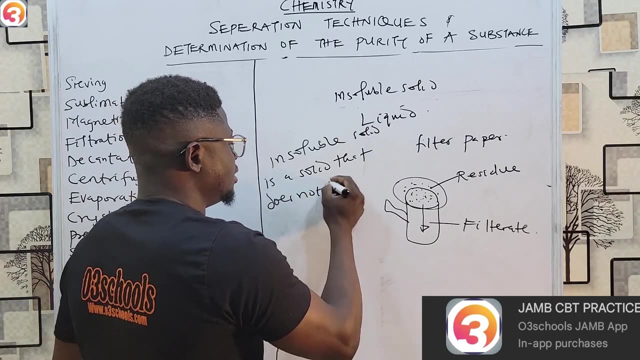 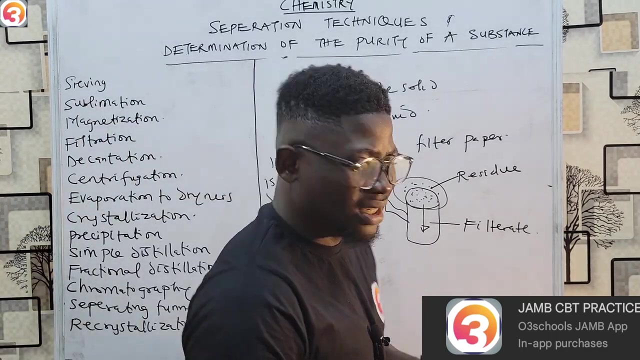 call filtration. we have been able to water filter. what the what? the insoluble solid and what is an insoluble solid? by the way, an insoluble solid solid, you say what is a solid that does not, that that does not dissolve in water. so an insoluble solid is a solid that does not what dissolve in water. so of course that is what. 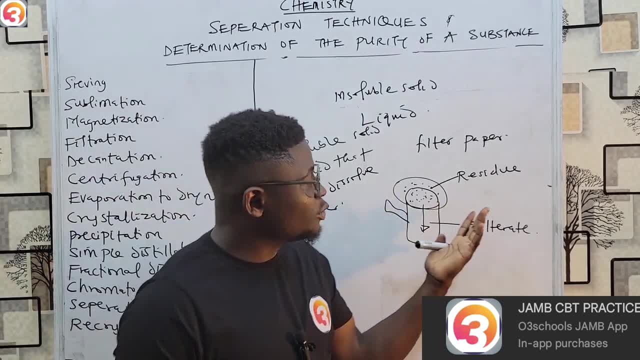 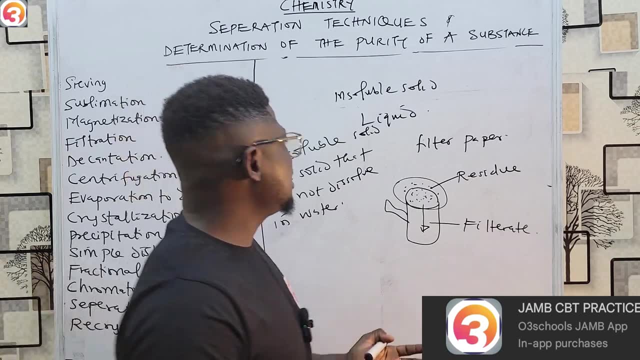 what an insoluble solid is. so, of course, uh, the particle that's still on top of the filter paper called the residue, while the one that's what goes down is called what? the filtrate. all right, so now we are going to continue with the next separation technique, and that is. 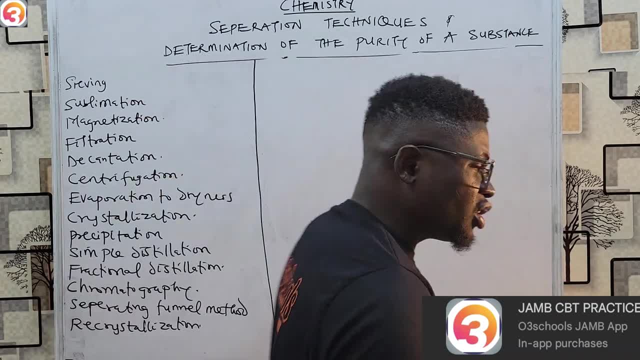 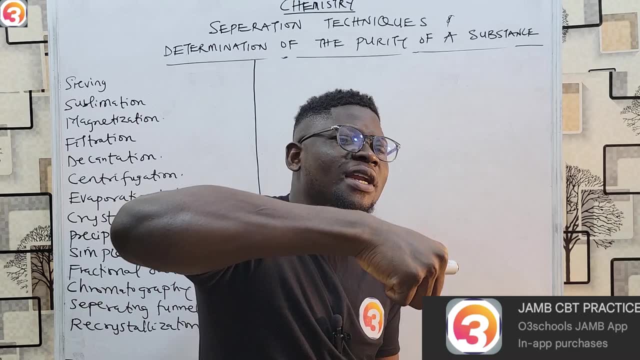 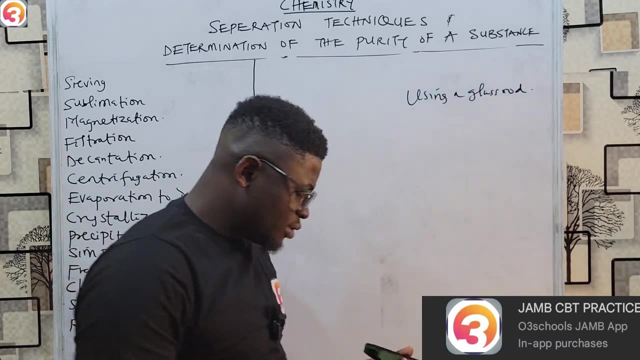 decantation, decantation. decantation also is used for what? to separate an insoluble solid and a liquid by pouring the liquid off carefully using a glass rod, using a glass rod. so once you are doing decantation, you are pouring the liquid off carefully from the mixture. by what, using what a? 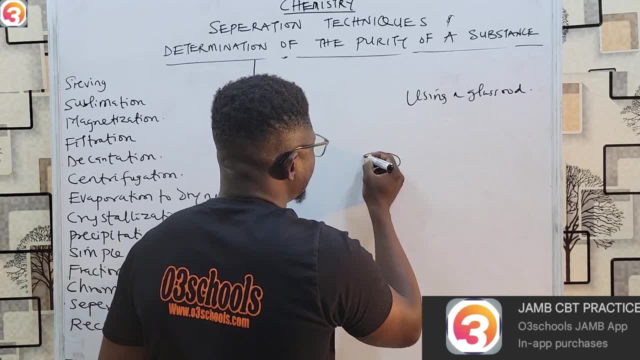 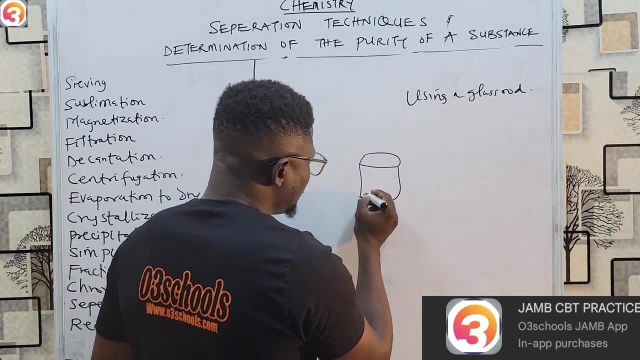 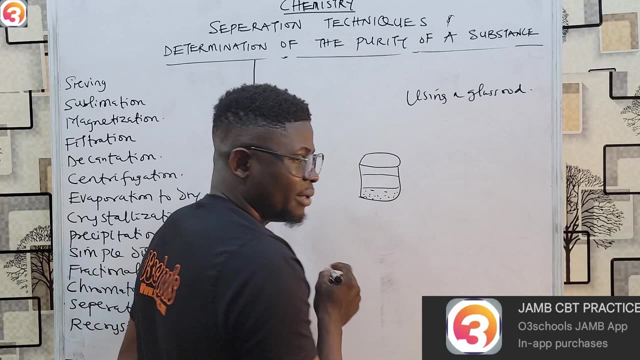 glass rod. so, for example, let's say you have a big car, uh, you have a big car like this. um man, i don't mind my drawing, you have a big car like this. and then you have what? an insoluble solid below. then you have a liquid. you have liquid, clear, clear liquid at the top here from: 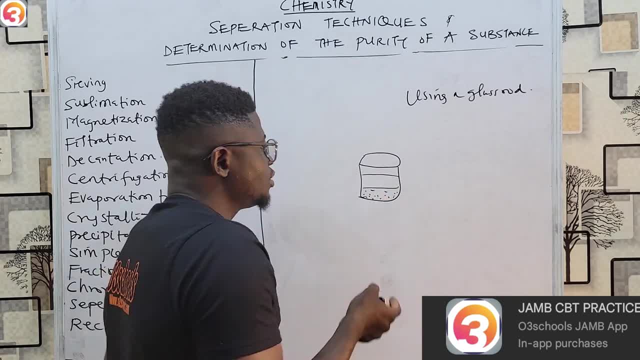 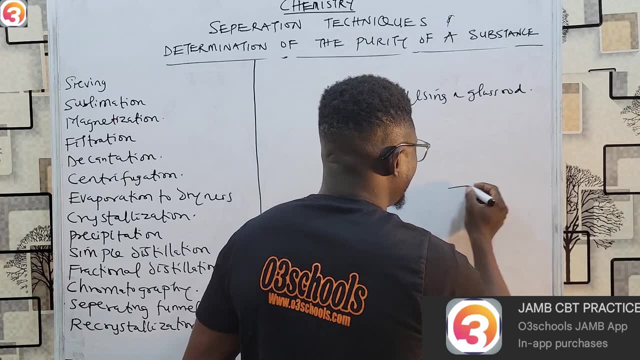 here to here, for example, where the liquid solid comes down, right, so you can use what the condition to separate what this, uh, these two mixtures, using what a glass, so you can have another, another, bigger, for example, that you are separating it into right, so you have your glass. 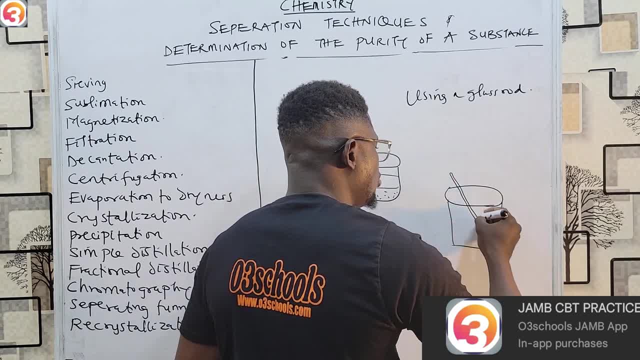 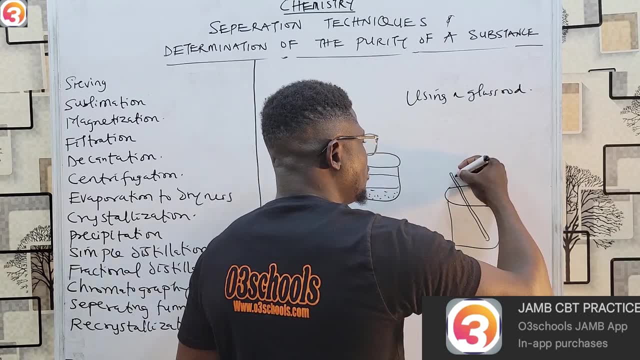 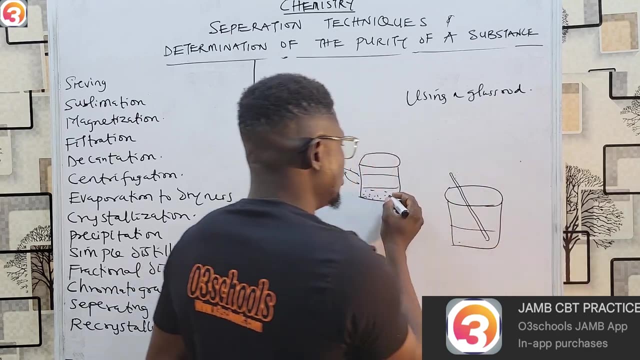 rod, carefully placed like this, and then you pour your liquid. it's a liquid now, let's say it has an angle like this, then you pour that liquid carefully on top of what this glass roll, so that goes on gently, so that liquid, what comes below here, right, and then it is leaving your 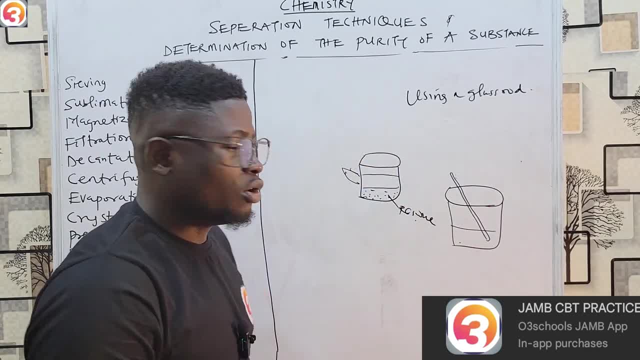 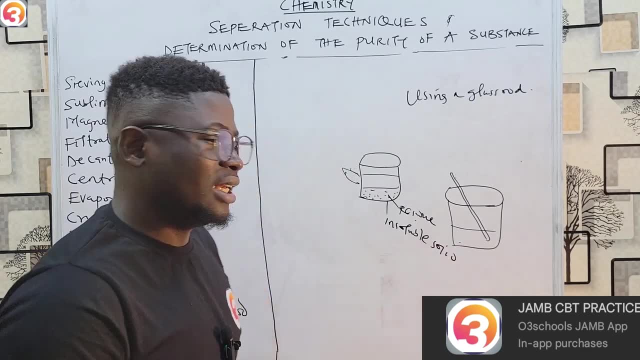 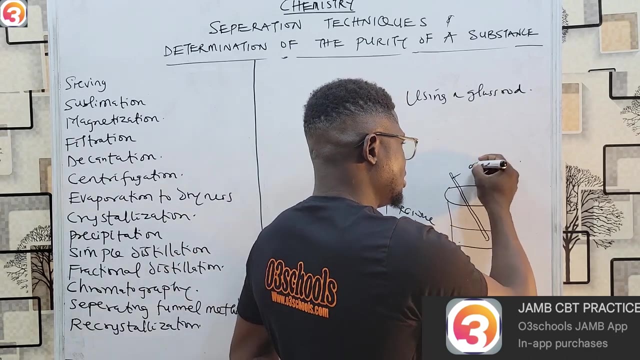 residue or what's your solid or your insoluble solid, rather, or your insoluble soluble solid or your ensemble solid in the water in the beaker. so you pour gently the liquid off using what's a glass draw. this is a glass, a glass rod i used to get out. so that is what, uh. 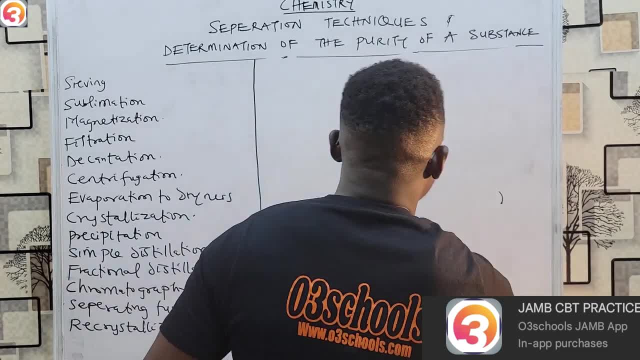 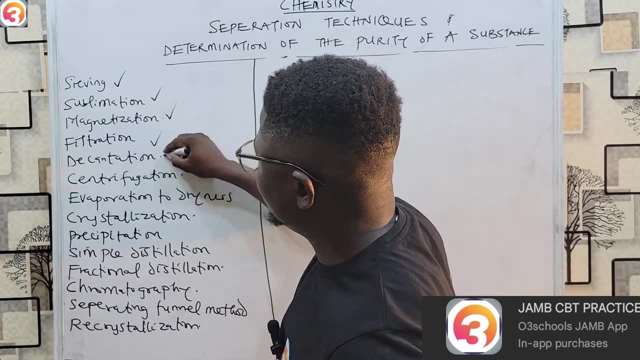 that is what decantation is about. so we now move over to the next one, which is what centrifugation? so we have done searing, we have done sublimation, we have done magnetization, we have done filtration- i don't decantation. now we are going to 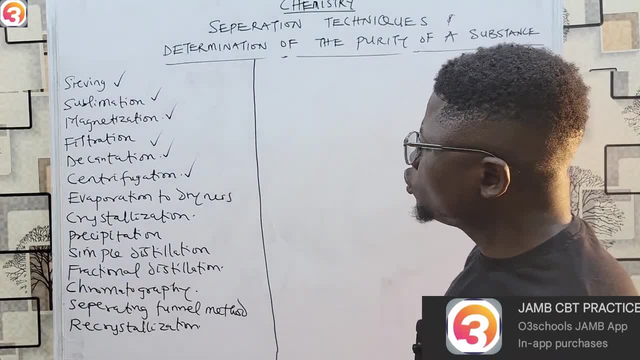 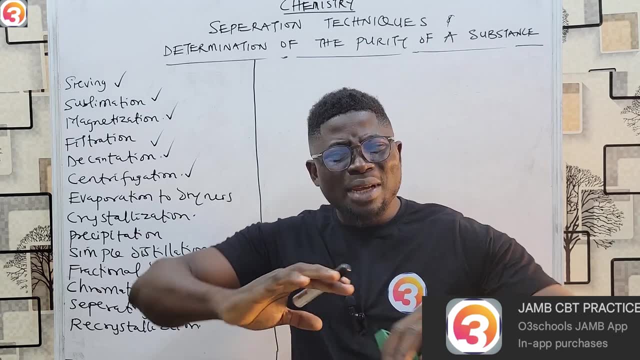 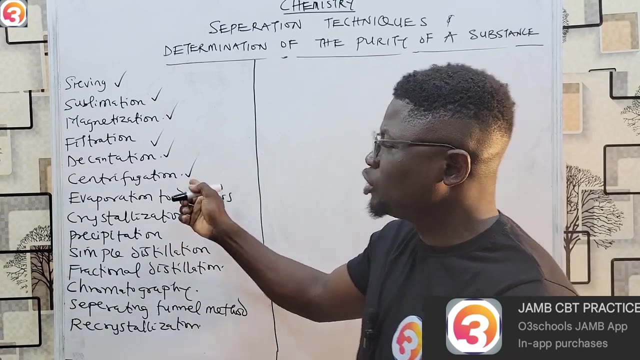 centrifugation. centrifugation is also used to separate an insoluble solid and a what and a liquid by pouring the mixture in the by what, by spinning the mixture in the centrifuge. so you have the centrifuge, you have a machine that has a chamber that you pour the water mixture of the insoluble. 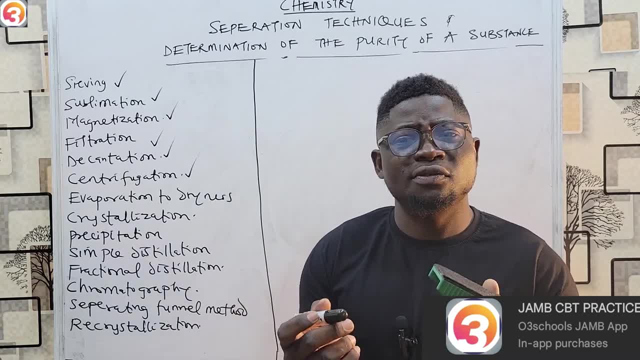 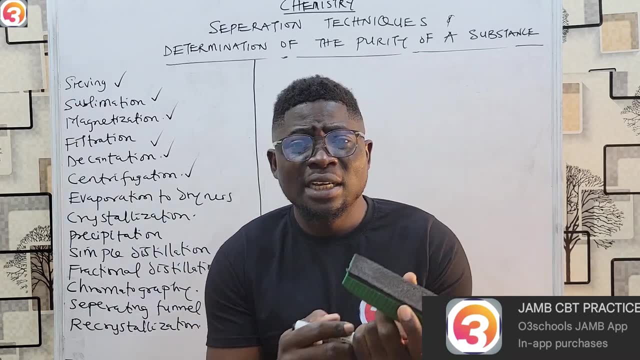 solid and the liquid in and then you spin it inside that centrifuge. the center of the centrifuge gas spinning machine is a very simple machine. it has just. it has a motor, it has a drive shaft and then the chamber where you pour the liquid in. so it is pin the mixture together. so of course that is what. 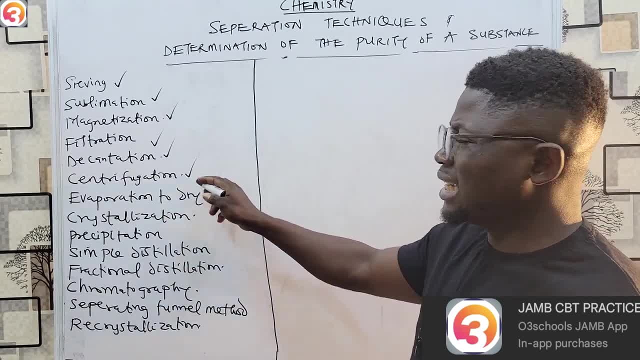 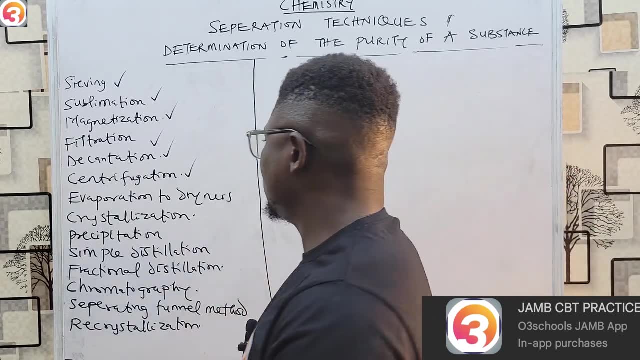 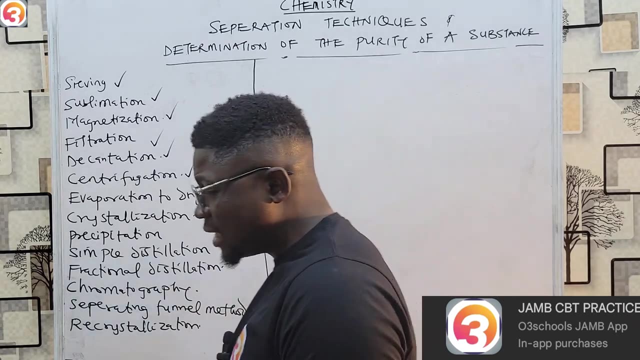 centrifugation is used- for it's just a word- to separate an insoluble solid and a liquid by spinning the mixture in the centrifuge. by spinning the mixture in the centrifuge, then of course we go to evaporation, to dryness. so this is by far one of the simplest. the easiest was separation techniques. 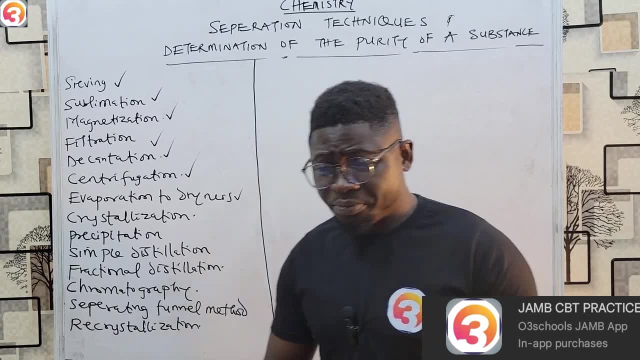 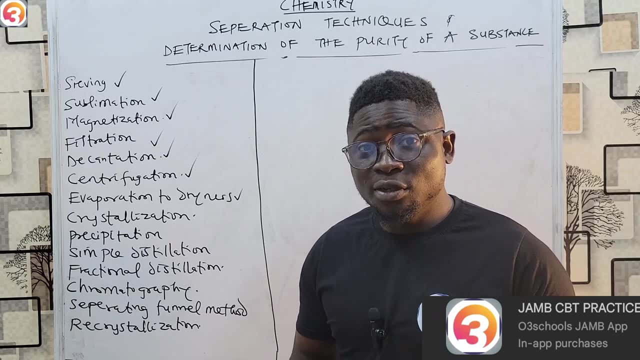 that we have because you yourself you might have done it before. let's say, uh, you want to dry, uh yam. let's say yam pills. in the village. some of you do it, right, you do. you dry yam pills after your mommy i peeled that yam. when i say, go and write us, i want you to do a robot, right, you must. 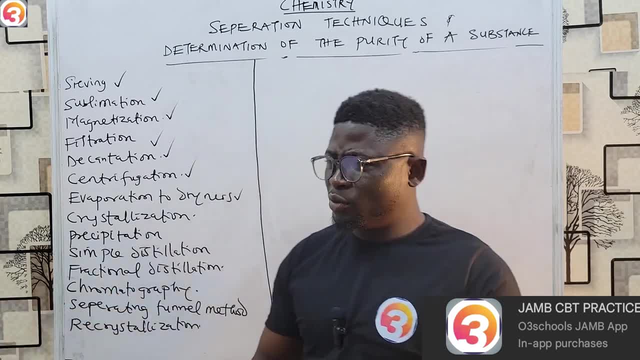 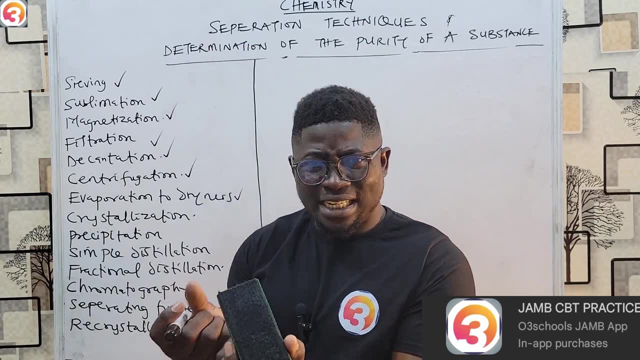 have heard that before. so what you do? you dry it under the sun so that what the liquid from the water, from the yam pills, we, what we evaporate to the atmosphere, leaving the dried water yam pills. right, that is evaporation to dryness. so it is what it is: separation of what is to what it is. 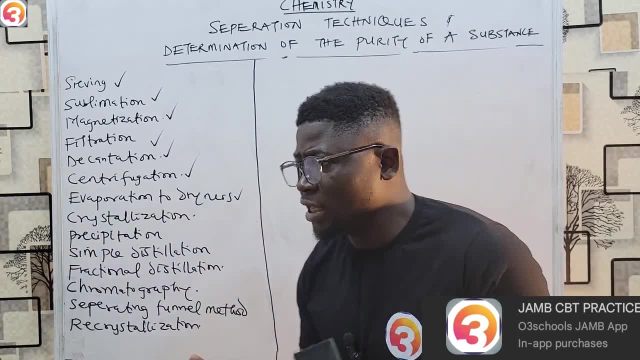 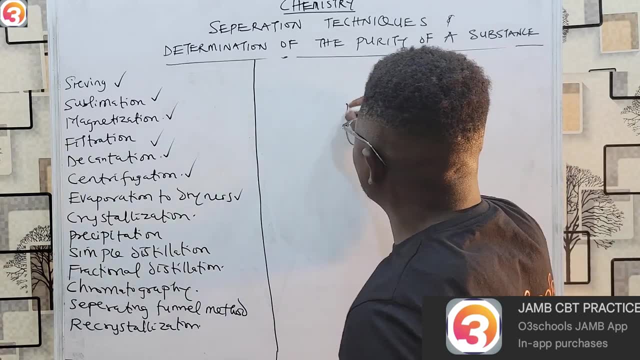 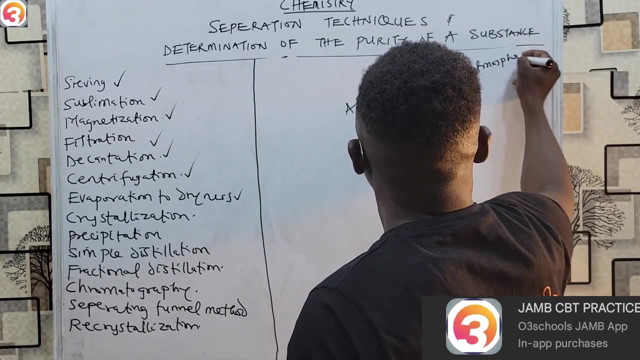 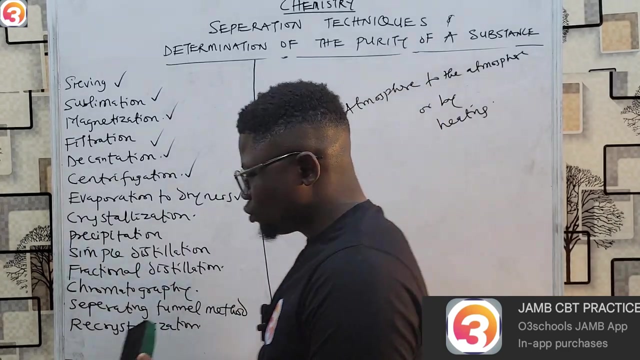 a? uh, recover what a, a a solid evaporation, trying to recover what is solid by exposing what is solid to the world, to the atmosphere. exposure to the atmosphere, or by what? or by or by heating. you say that you heat or what you expose to the atmosphere. so 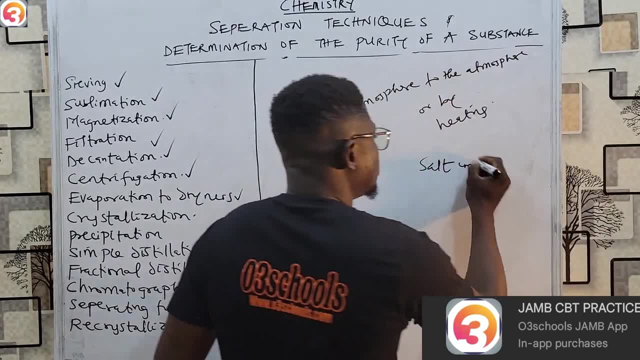 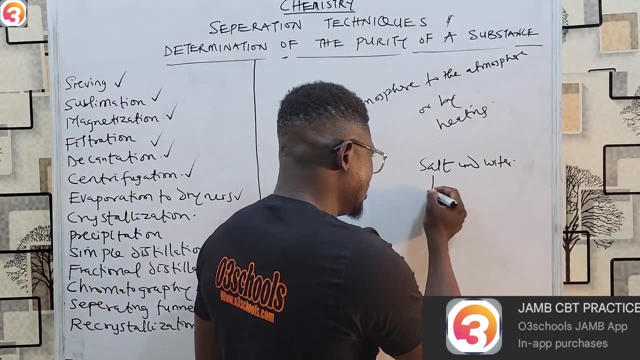 for example, a mixture of salt, salt and water, water, a mixture of salt and water, right, it will dissolve it in it, but you can, you can easily what recover? what is the salt from the water, from the water? so, if you, if you heat, if you hit the water, 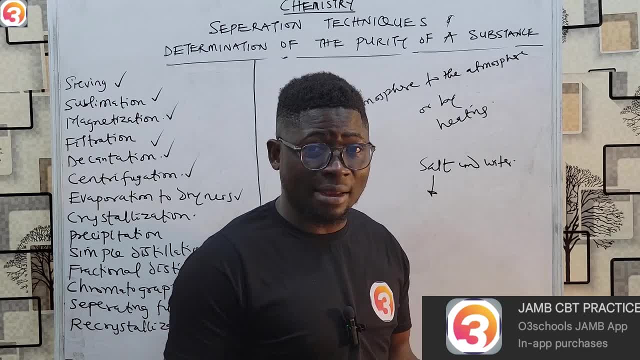 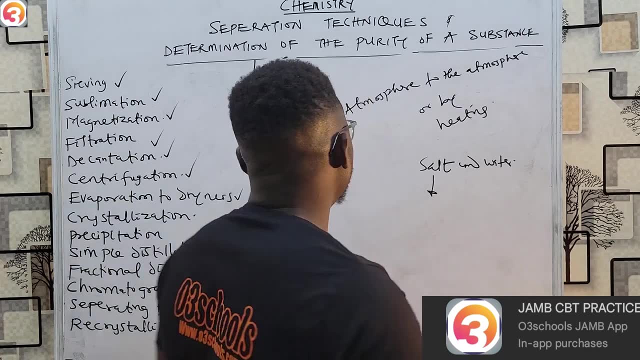 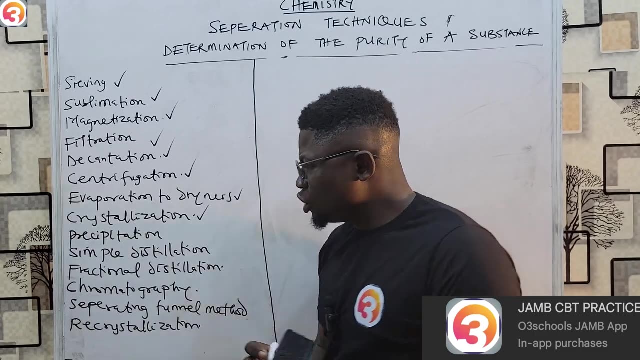 will evaporate, or if you expose to the hospital for a very long time, depending on the quantity of water. anyway, of course the water also would evaporate, leaving what the salt out. so that is evaporation to dryness. now we move over to crystallization. crystallization is used to recover. 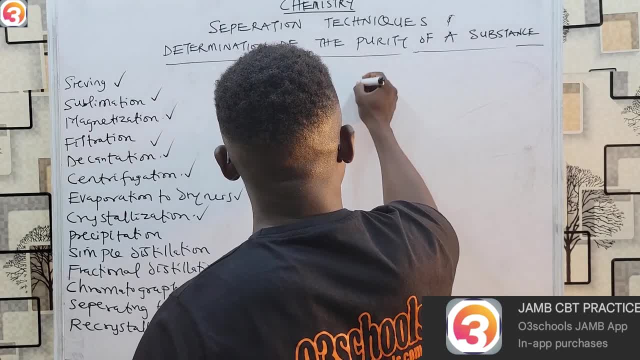 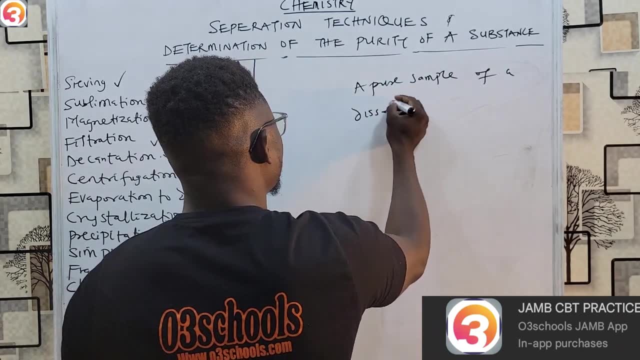 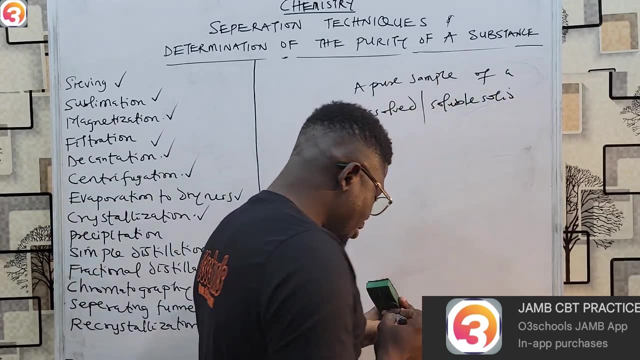 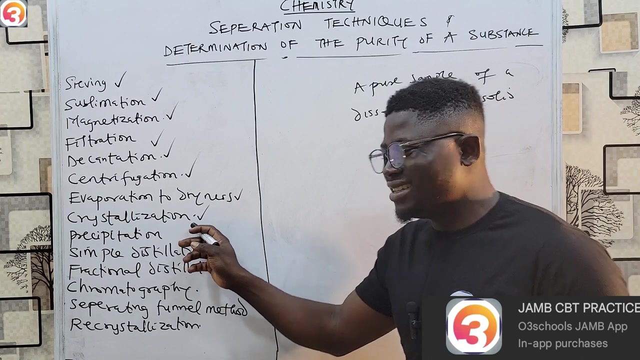 a pure sample of a dissolved, a pure sample of what of a dissolved, dissolved or was soluble solid by various means. there are various means- or to recover what, this pure sample of what of a dissolved or soluble solid. that is what about crystallization. now we say crystallization is to 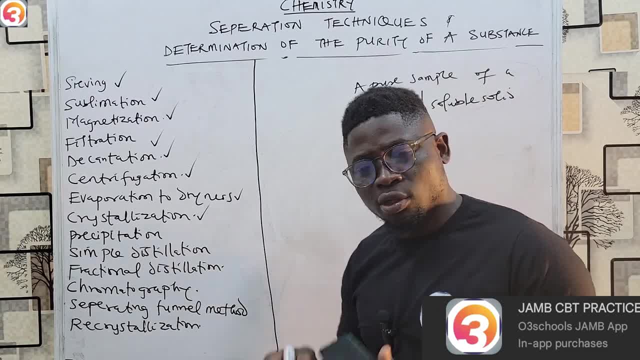 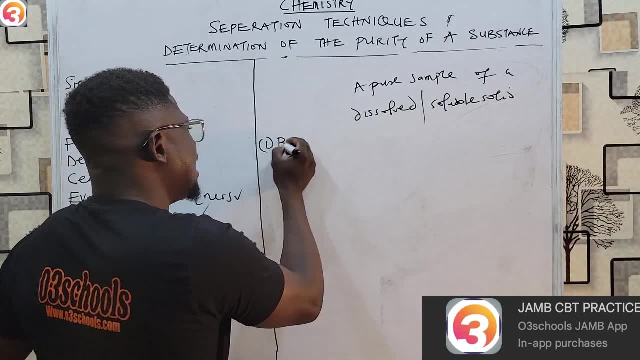 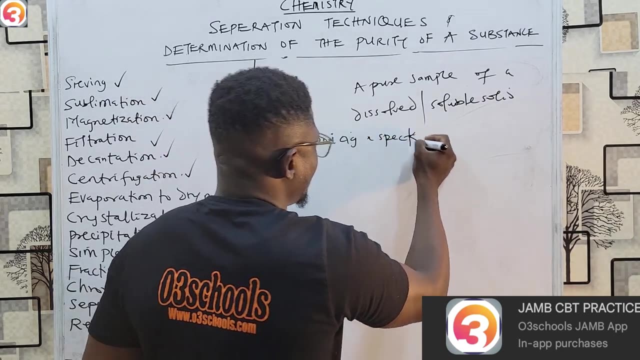 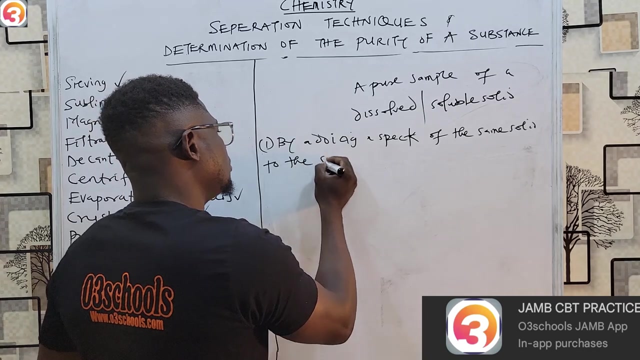 recover a pure sample of a dissolved or soluble, or soluble from a solution by various means. what are the various means? number one: by adding, by adding. by adding a spec expect of the same solid to the solution, but by adding a speck of the same solid to the solution. that is one of the way to recover what 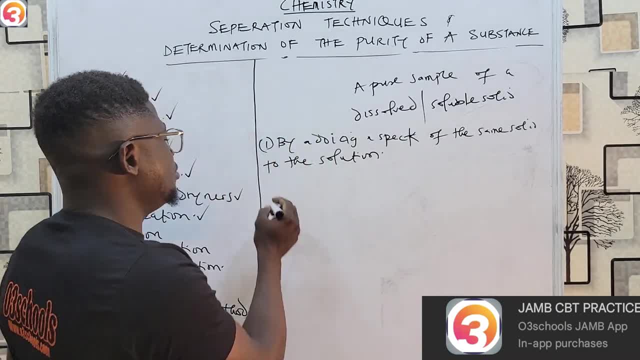 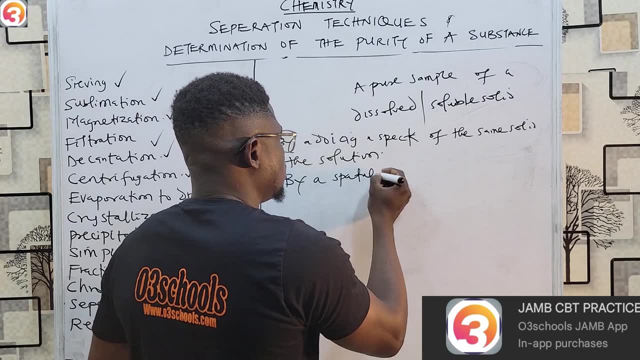 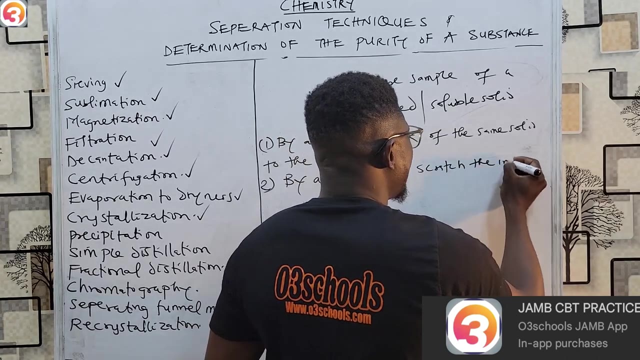 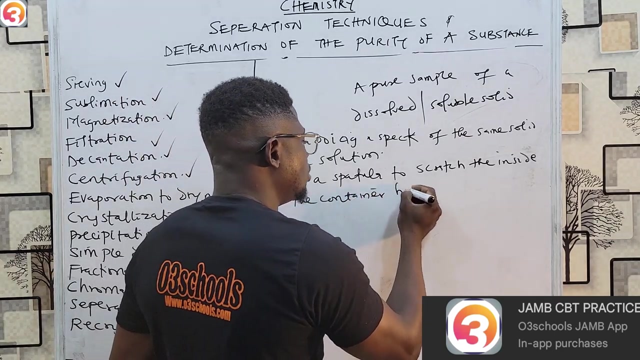 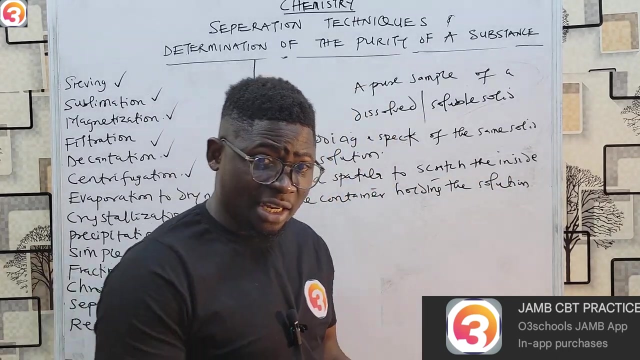 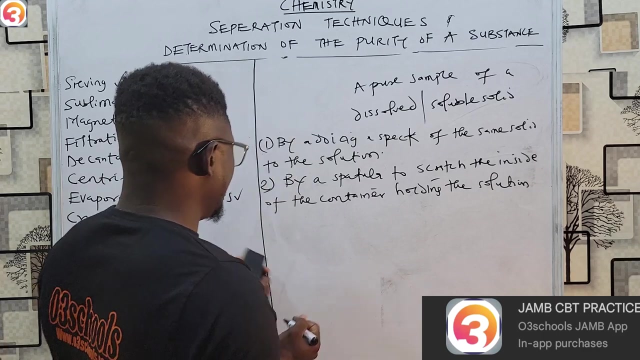 that pure sample. number two: by what? by using a spatula to what? to scrape or to scratch the inside of the container, so holding the solution. so you use what a spatula is like, like a spoon to use water scrape or the inside of what, of what the container was holding what the solution. then, number three: by shaking. 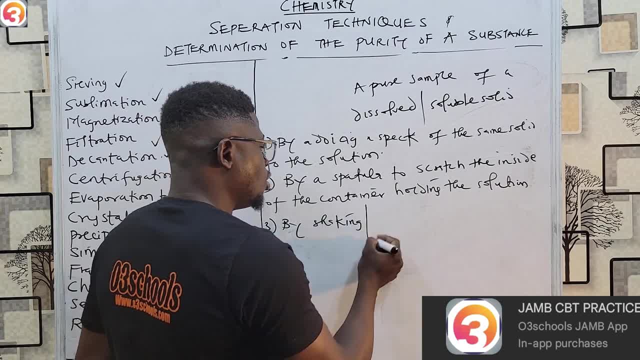 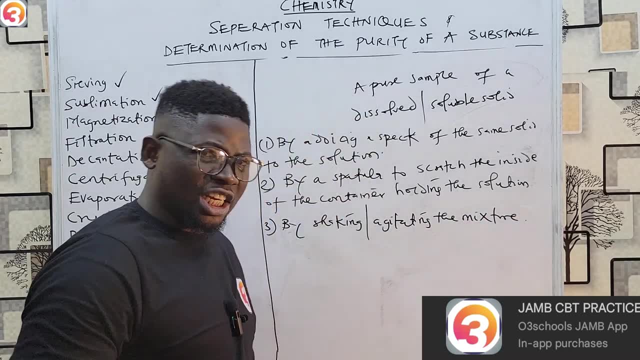 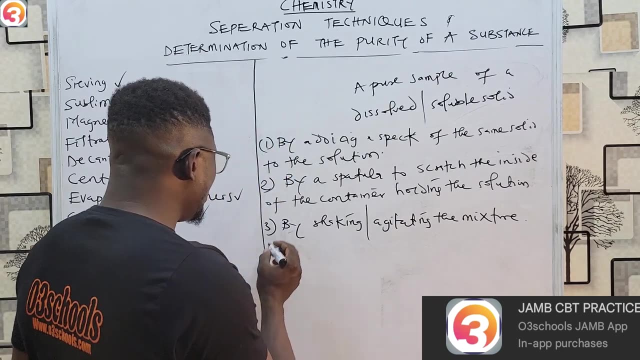 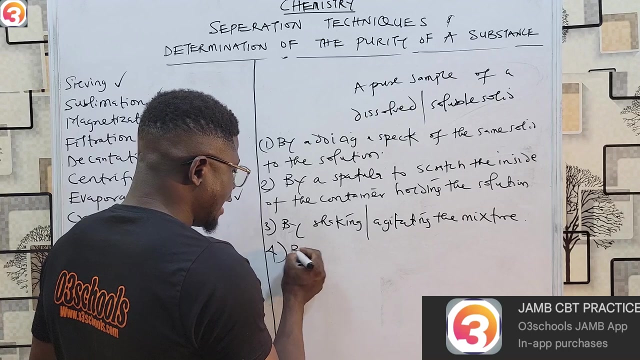 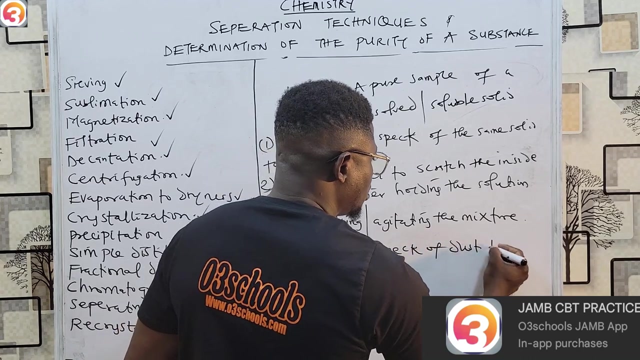 by shaking or agitating the what, the mixture. so you shake it or you what you know what. shaking, shaking something, as well as agitating. you shake or you agitate what the nature in the solution, and one very unpopular method or do of of what, of recovering this pure sample, is by what? by adding a speck of dust, of dust to serve, to serve. 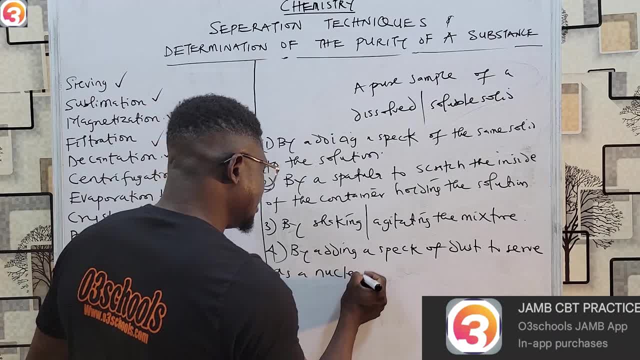 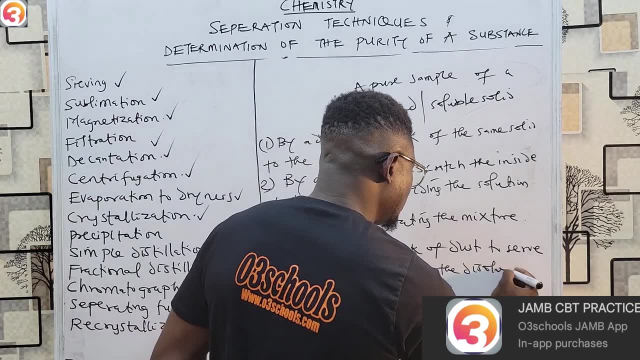 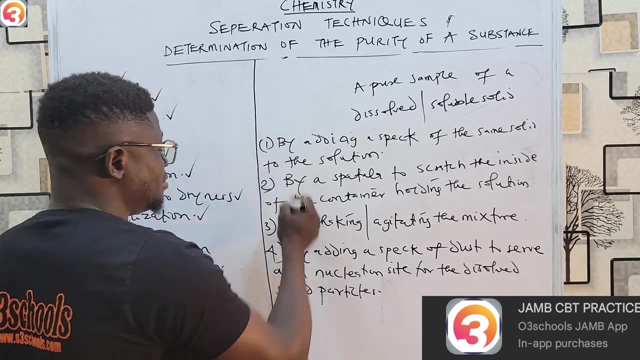 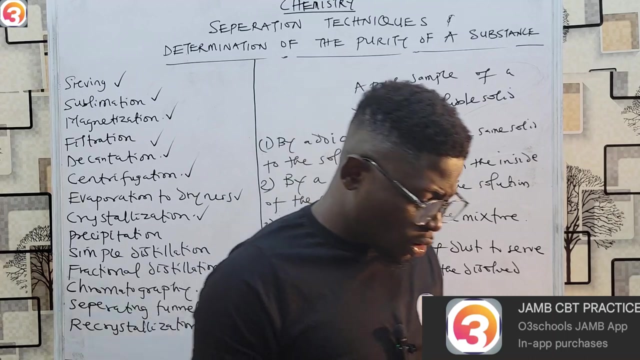 to serve as a nucleation side, to serve as a nucleation site for the workout. as you showed, his first three methods actually very popular, but this one is not what very, very common right? so, uh, crystallization is used for what? to recover what dissolves solids that are easily would decompose, that easily decompose on it. 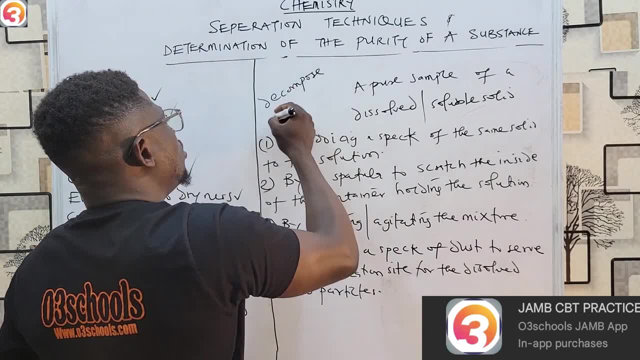 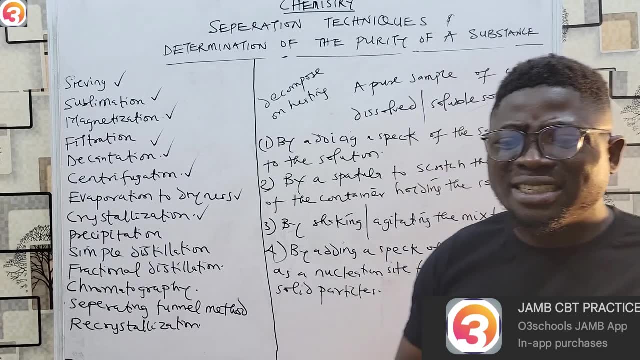 that easily decompose on it. that is easily decompose on it, right, because the crystallization. and that easily decompose on what? on heating, that's what the tradition is used for. this will recover what they deserve, or solid the least would recover: dissolve solids that. what easily? what decompose on it in order to cover solids that? 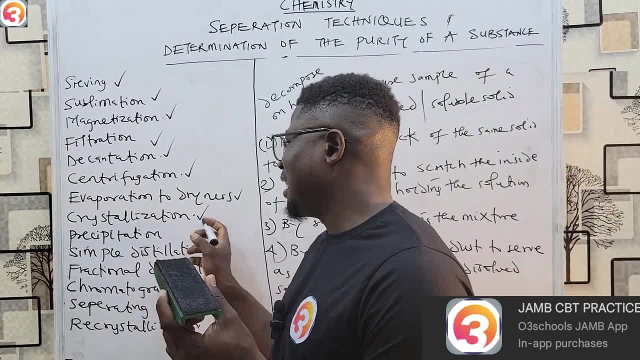 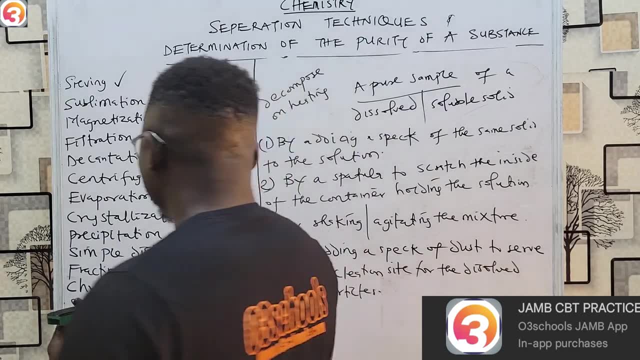 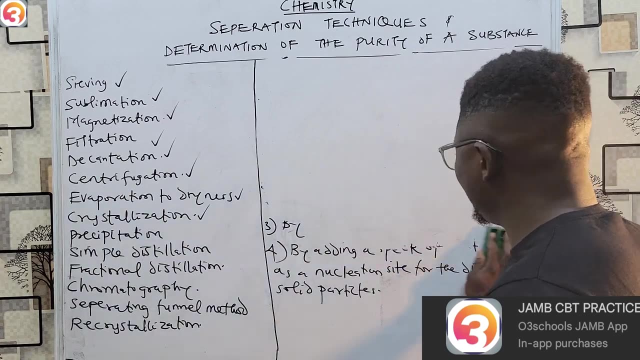 easily decompose on heating and, of course, when we use crystallization, a very pure sample, a very pure sample is what we usually would get, all right. so now let's go to the next one, and that is what precipitation? precipitation is also: what recover? what an insoluble. what is to separate? what an insoluble solid? 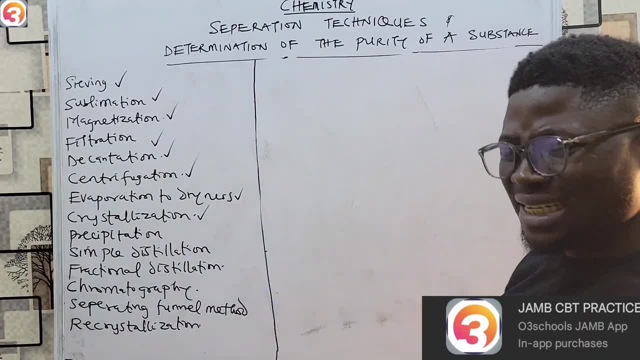 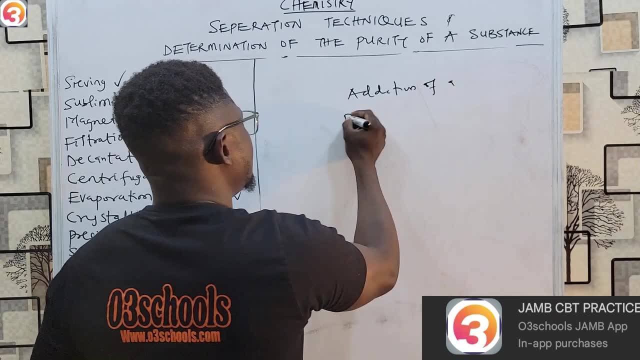 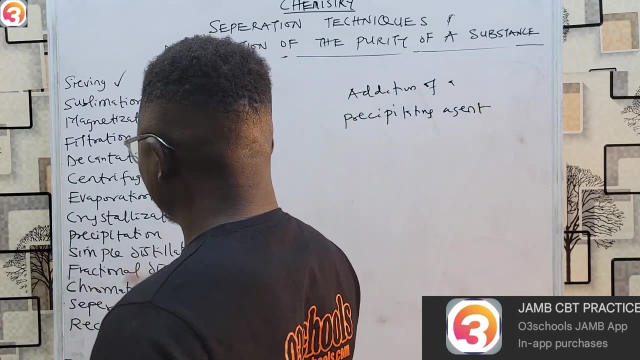 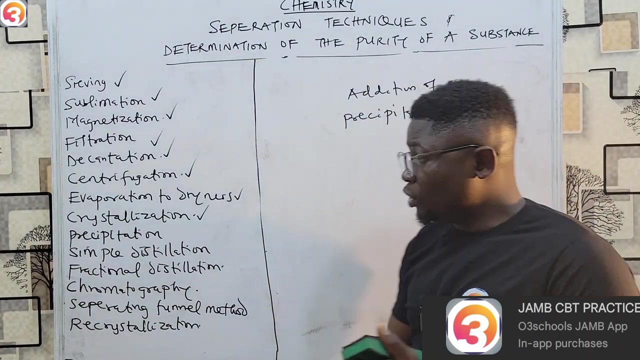 right for me sort solution by the addition of a precipitating agent, by the addition of a precipitating precipitating agent. so for precipitation was a resort, a precipitating agent to recover what that dissolve, what solid from what from the solution. so, unlike what crystallization right we'll have all. 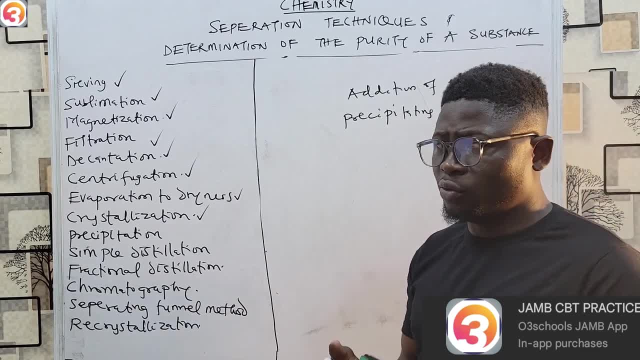 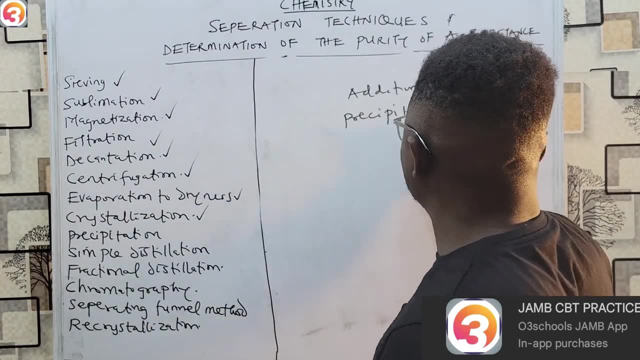 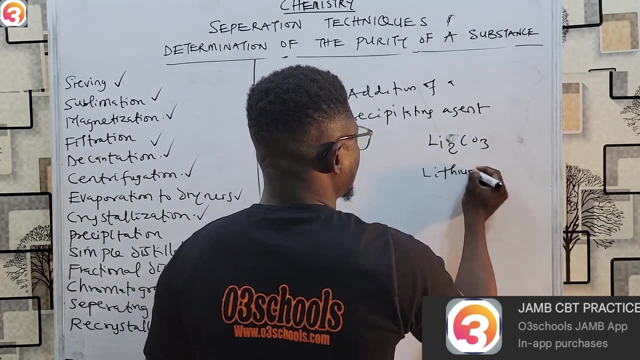 that means of what? of recovery? the pure sample for that dissolved solid, or what solution? so for precipitation, news what I will add, what a precipitating agent. example of a precipitating agent to go out. I like to, I like to see: oh three, this is lithium carbonate. 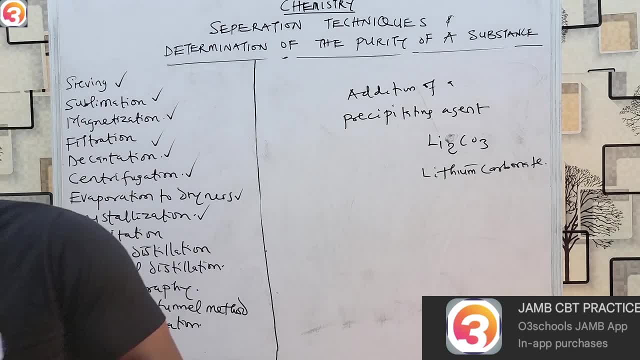 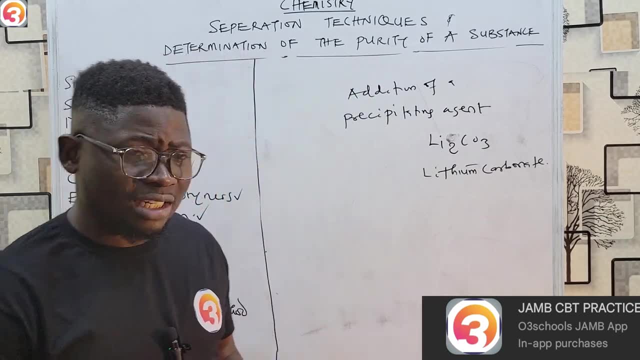 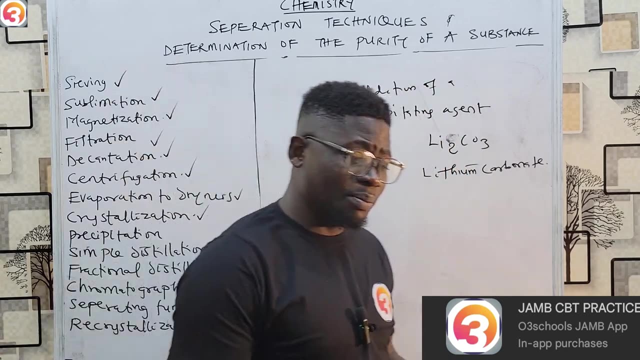 like by the addition of what of a precipitating agent. so press patient is just a use of what? or recovery works, so this dissolve or solid based on that, what defense rate of? or so the solubility in what different solvents, just for recovering what solid based on that different, or solubilities in different. 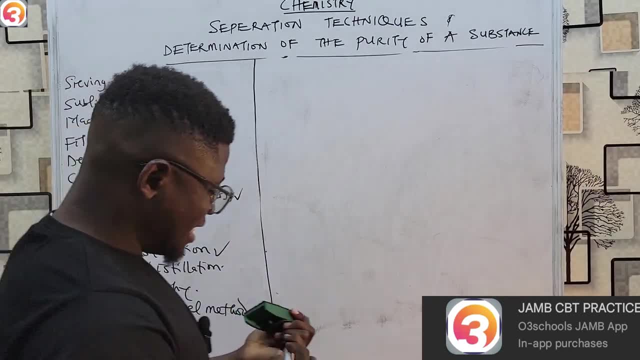 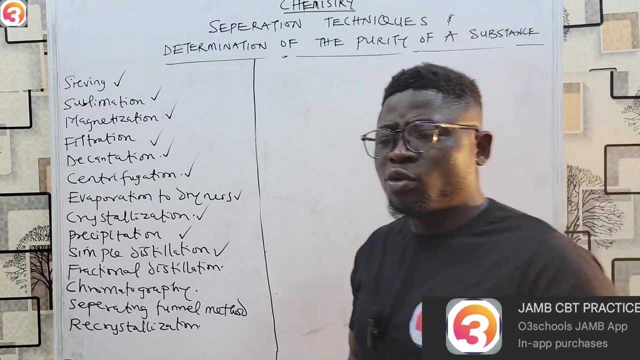 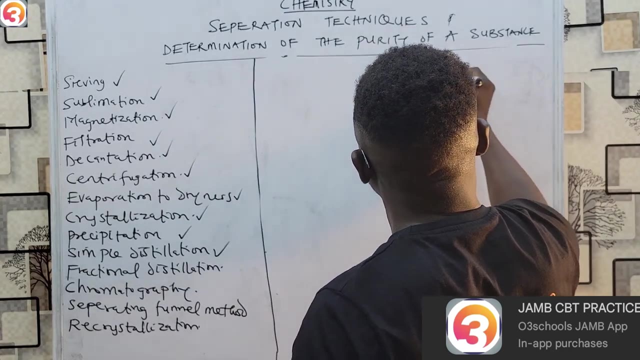 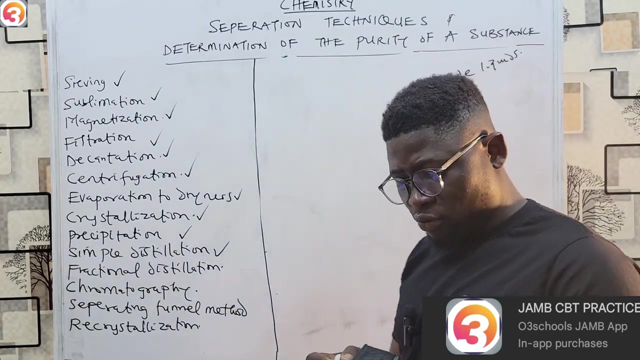 solvents. so we'll go to simple distillation now. and simple distillation is used to separate what, just to recover what's all the different ones based on, or to discover to recover to miscible liquids. to recover to miscible liquids it is to recover a solvent or what to miscible what liquids, whose boiling. 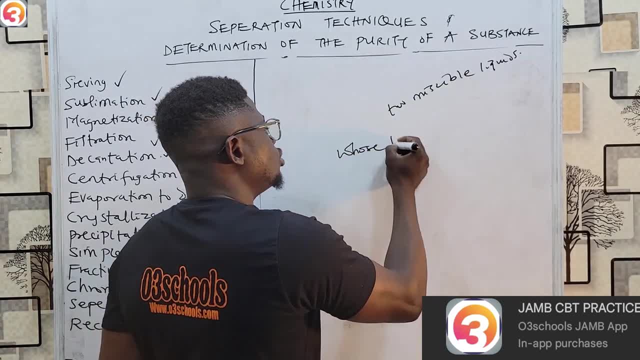 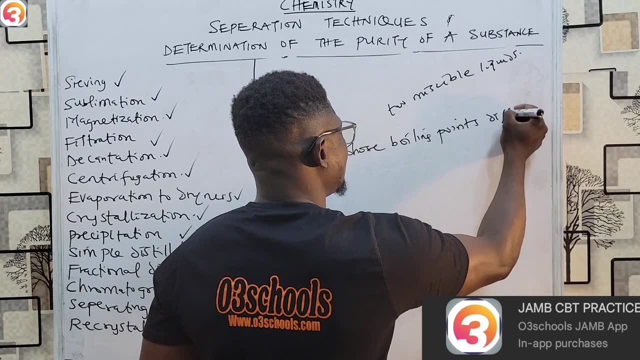 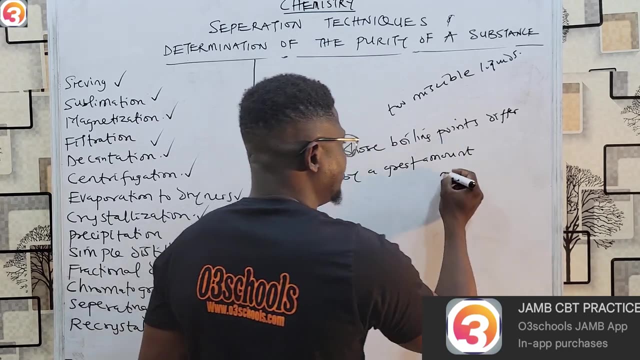 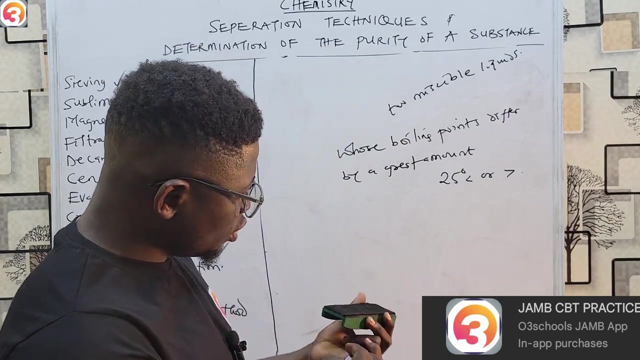 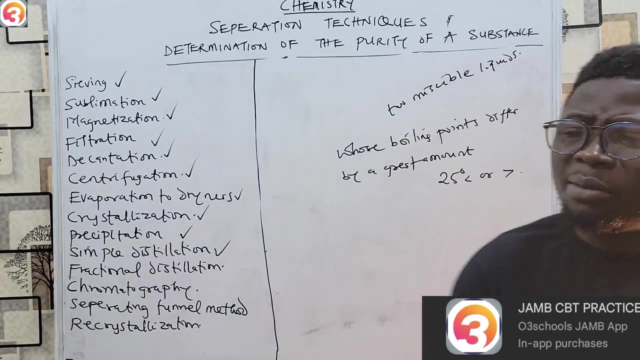 points, whose boiling points, whose boiling points differ by great amounts, differ by ignorance. amount is always 25-degree, says it was or was or great, half time between 37 socials over it up. so it is to watered to or to the Nokia buy. it was its own tool or were two separate, two miscibleterm oneband. 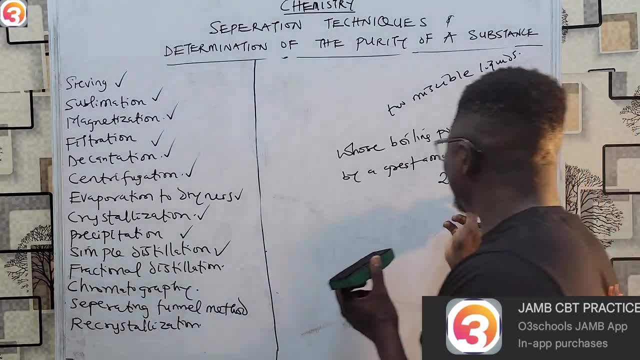 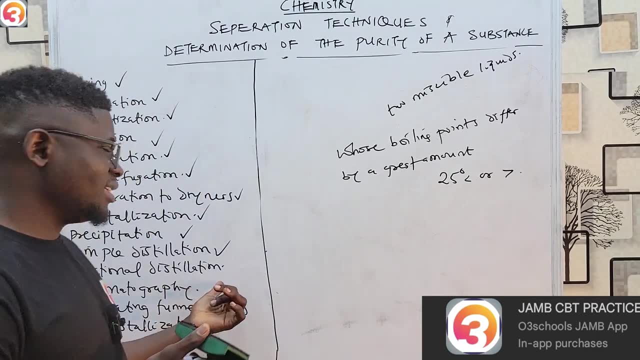 loyalty, compensation for building point by a great amount of any facility or what, or greater than a 36 or so mo 마, we are alijk looking at whether it is simple distillation or fractional distillation. whenever you are seeing temperature, look at the temperature that you are using water to separate and, of course, if it is, 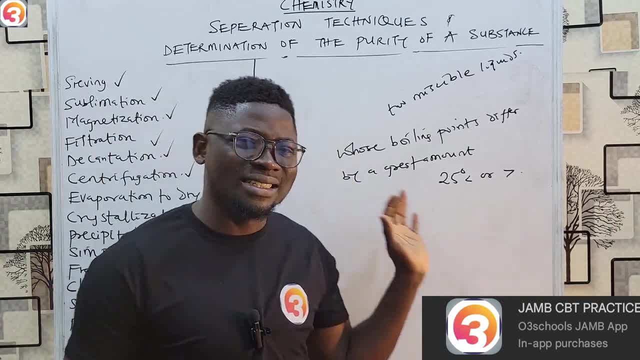 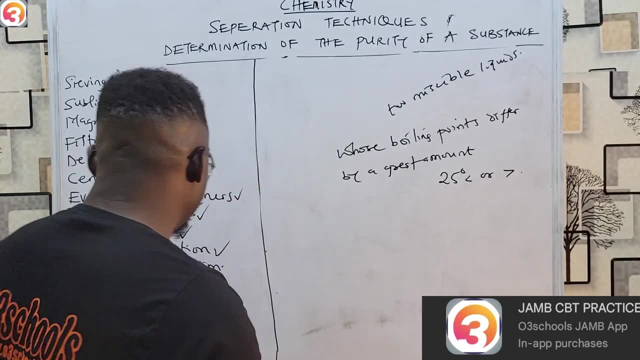 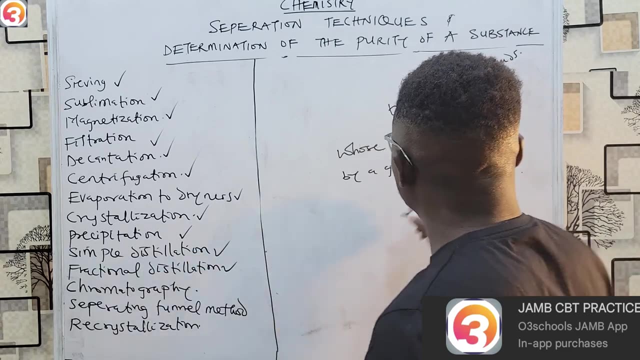 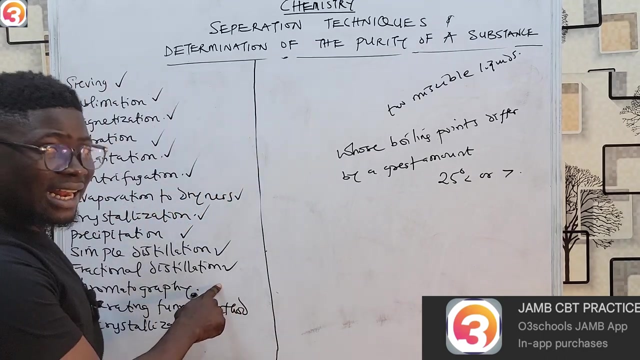 25 degrees Celsius or more than it know that simple distillation is the separation is the best suitable separation technique to what to use. why? fractional distillation is also used to separate two miscible liquids whose boiling points are what are close together? whose boiling points are close together? is it a less than 25 degrees Celsius, right so? whose boiling points are close? 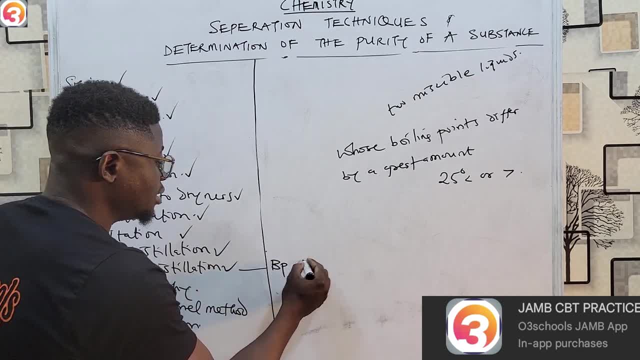 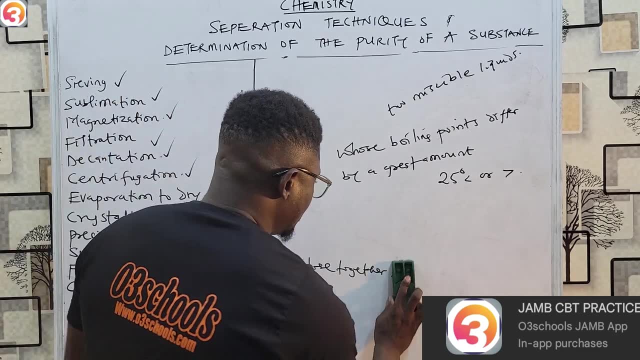 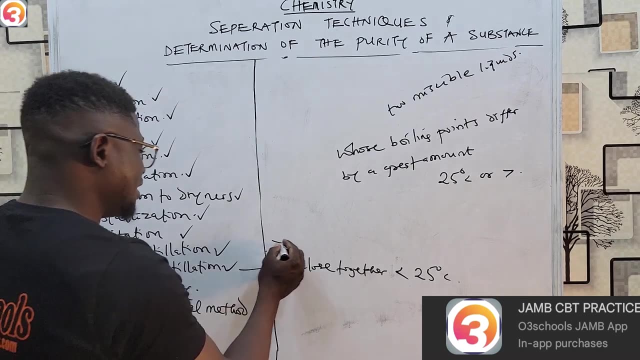 together at this one. boiling points, BP boiling points are closed together. that is a less time. this is good time. sorry, so not sorry. that is less down to 25 degrees Celsius, right, but for simple distillation. great thought. and what he said are 25 degrees Celsius, or greater than 25, if I decrease. 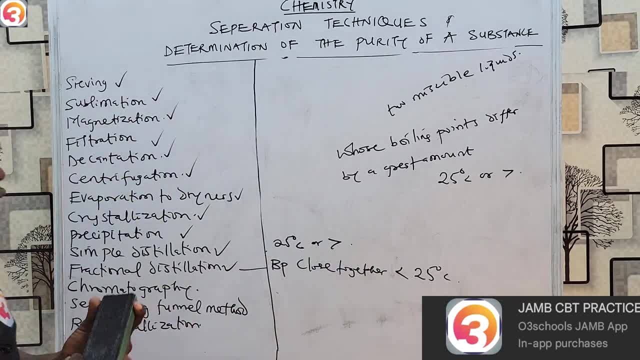 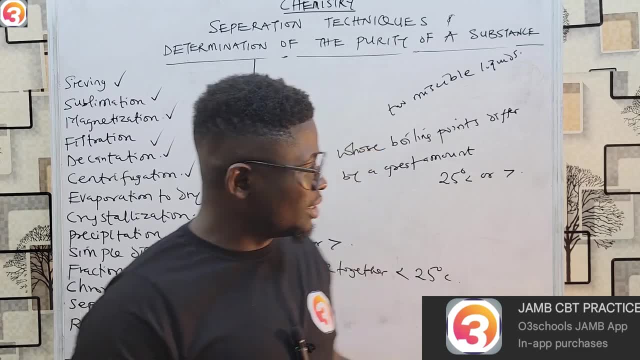 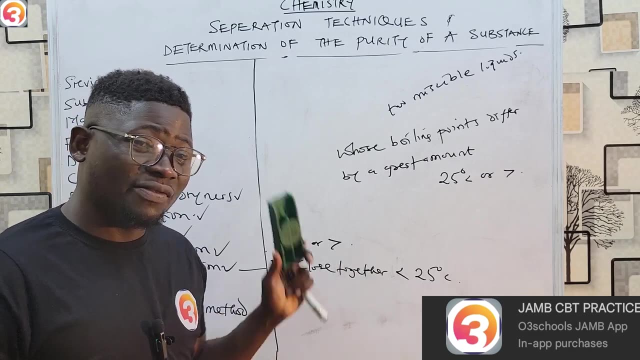 a or greater right. So you must take note of what those two do not get confused, that they do the same thing. But of course the temperature is what differentiates them. So if it is, if the abutting points are close together, less than 25 degrees Celsius, use fractional distillation. 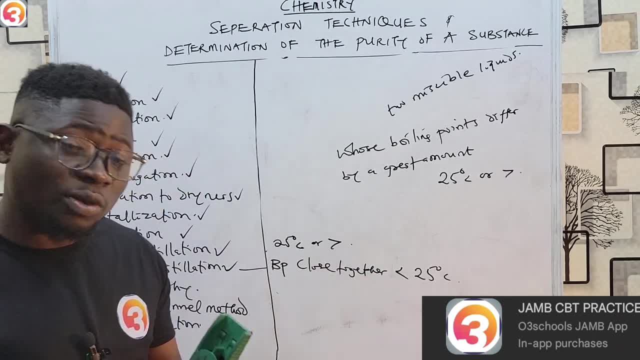 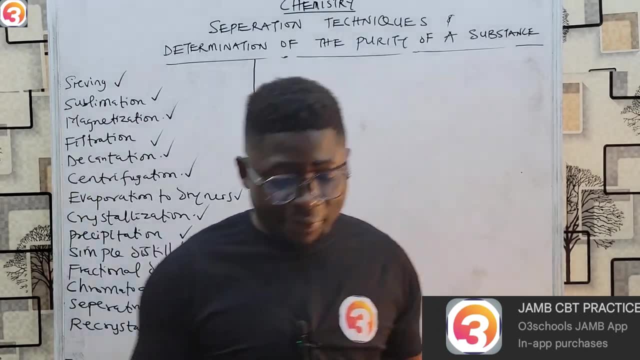 But if that temperatures are what are 25 degrees Celsius, is 25 degrees Celsius or greater than 25 degrees Celsius? then you use what? simple distillation. We now move to chromatography. Chromatography is used to what? To separate solutes based on their different rates. 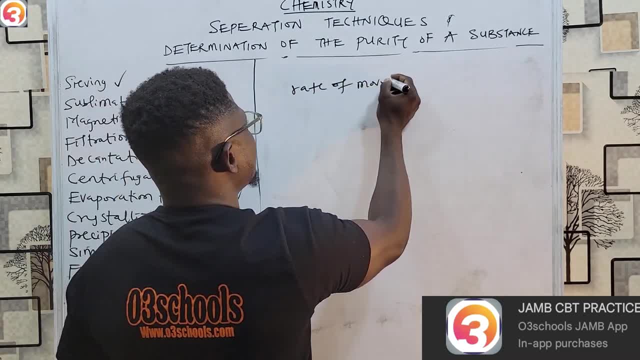 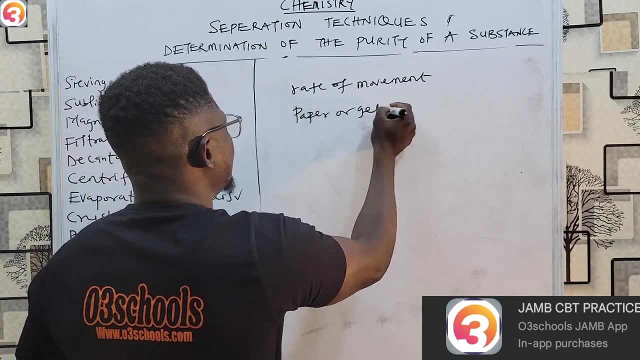 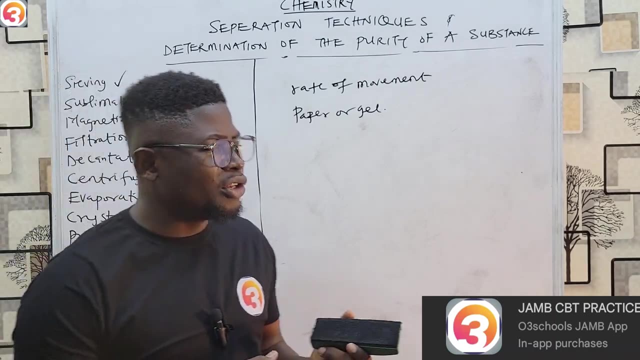 different rate of movements along a medium such as what- paper or gel. So chromatography is used to what? To separate solutes based on that different rate of movement along a medium such as paper or gel. So, based on technique. based on technique. 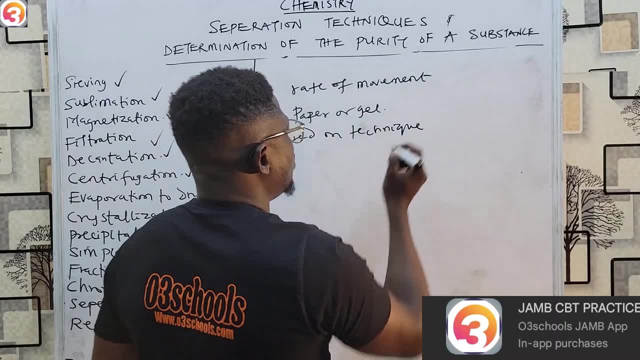 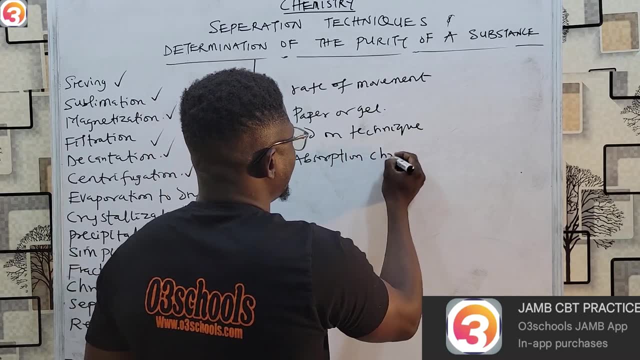 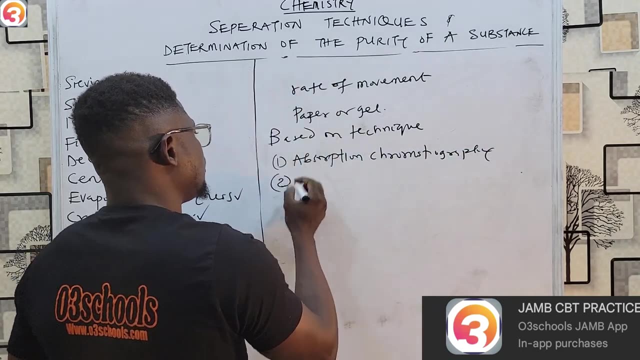 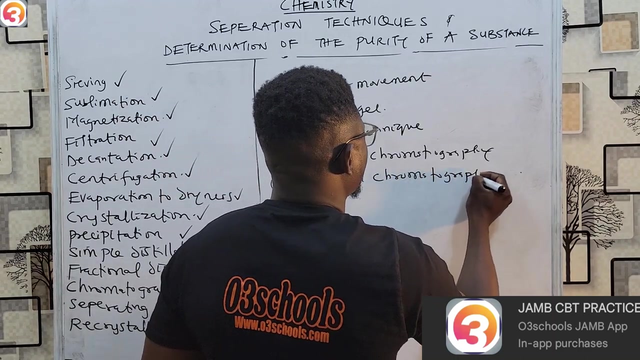 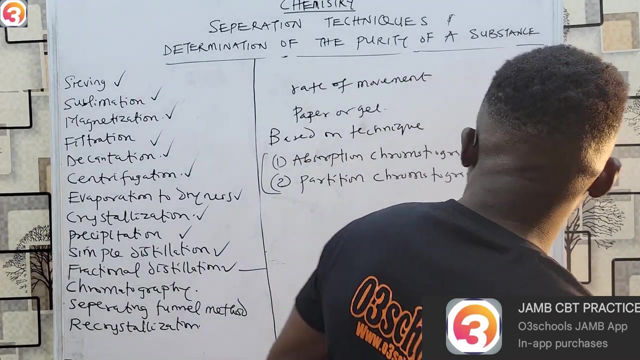 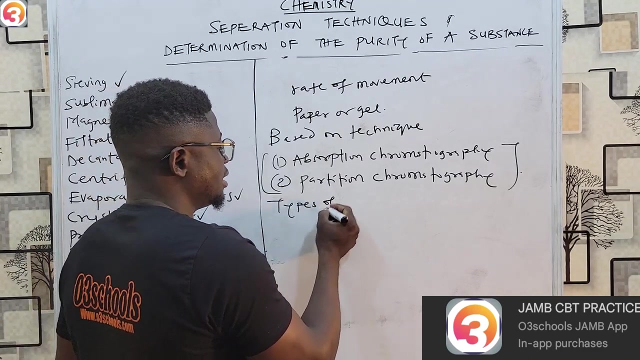 We have two types of chromatography and that is what: absorption, absorption chromatography chromatography and to partition chromatography. So, based on technique, we have two types of chromatography: absorption chromatography and partition chromatography. also, we have different types of chromatography, the types of chromatography. we have types of. 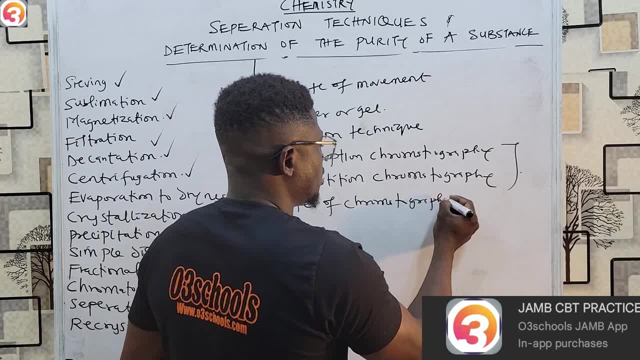 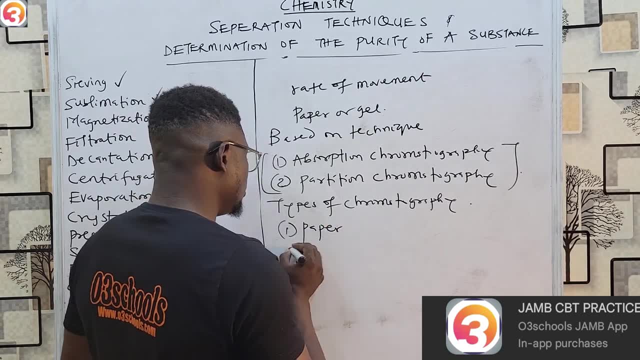 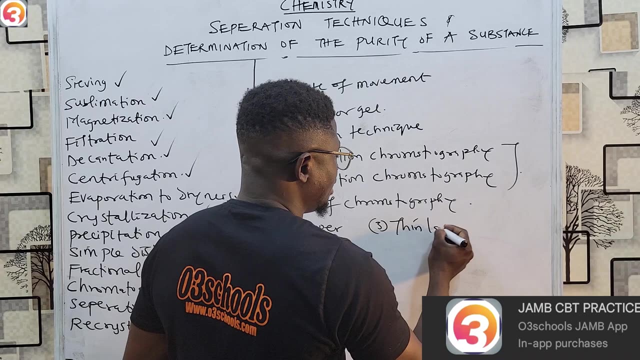 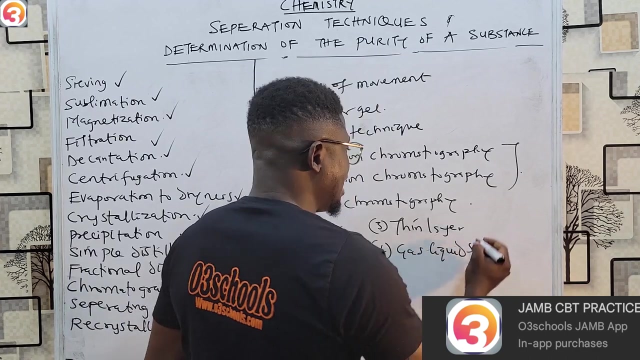 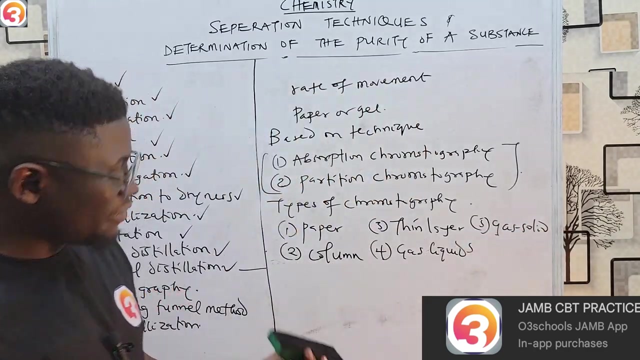 chromatography we have include: one: we have paper chromatography. two: we have column chromatography. three, we have thin layer chromatography. four: we have gas liquids chromatography. five, we have gas solid chromatography. so these are the types of chromatography that we have, now the constituents of what ink and 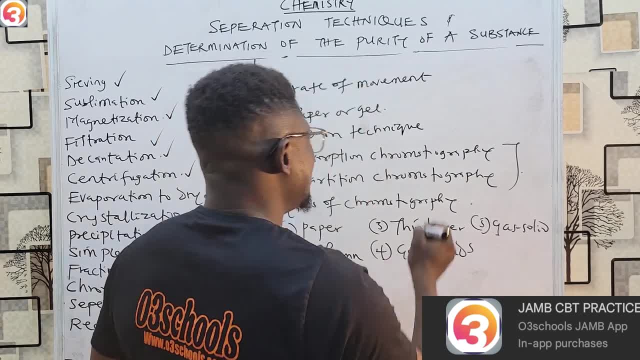 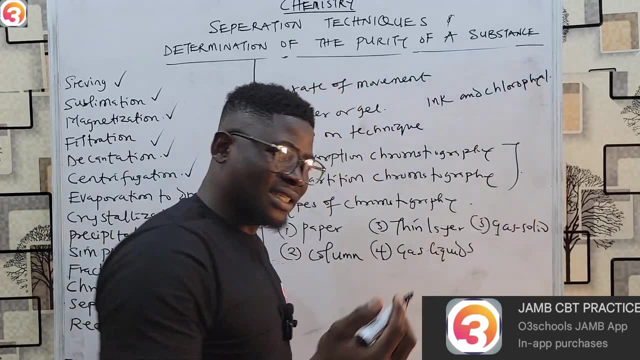 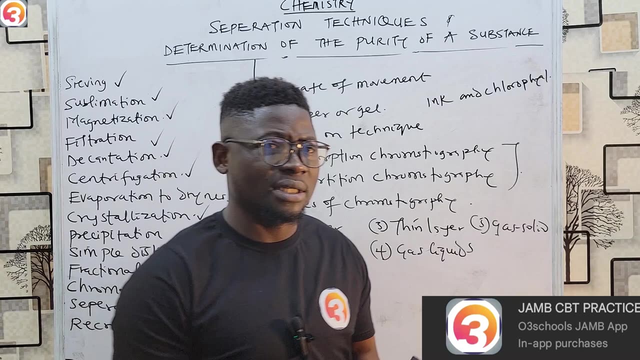 chlorophyll can be separated by what chromatography ink and chlorophyll. you know chlorophyll is what is the? what is the? is the something that will give what plants that green coloration, right? no, chlorophyll. it has different constituents. the major constraint of chlorophyll is 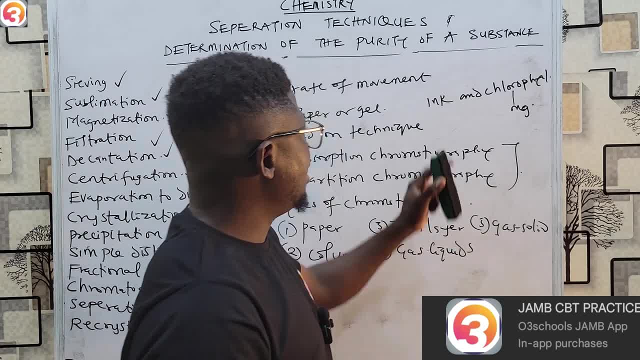 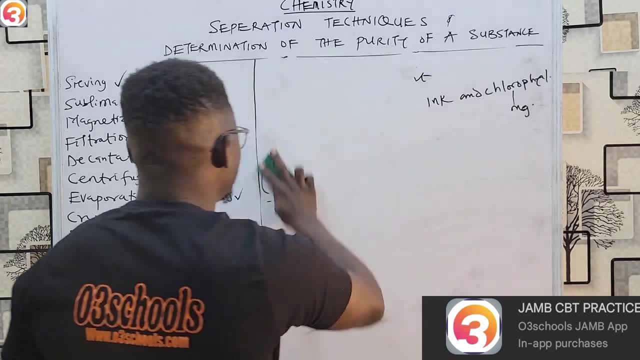 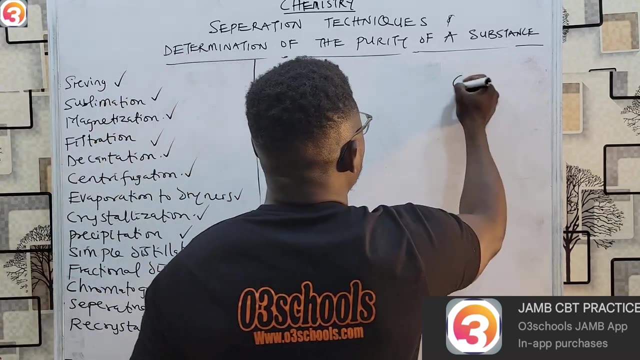 magnesium. it has other what constituents. but for ink, ink has several, it has lots of constituents. I think that is where I want to base our study of chromatography in ink and chlorophyll right. so for ink, ink has lots of constituents, chlorophyll right ink has lots of. 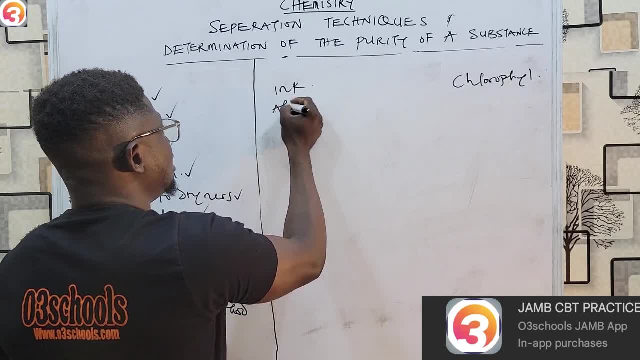 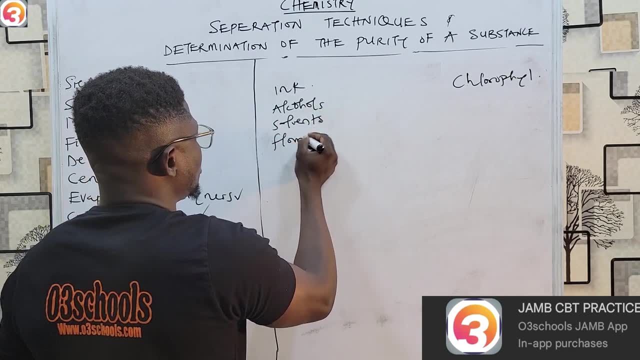 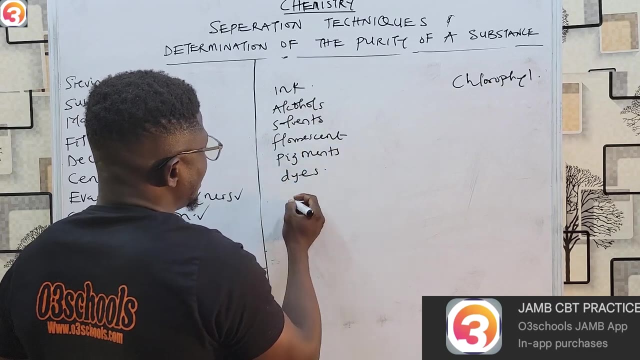 constituents such as the. it has constants. it has a aqueous in it. aqueous, it has solvents in it. it has what fluorescence. it has pigment. it has dyes. it has resins. it has water. it has dyes, it has resins, it has water. 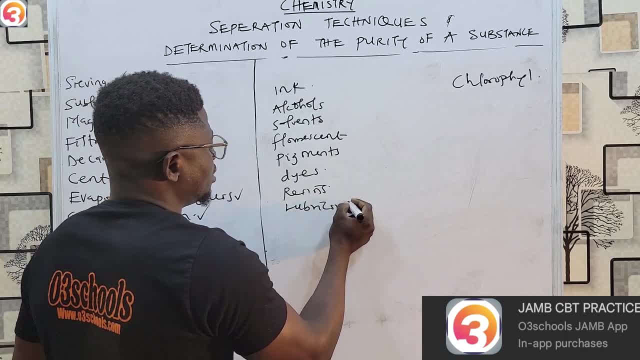 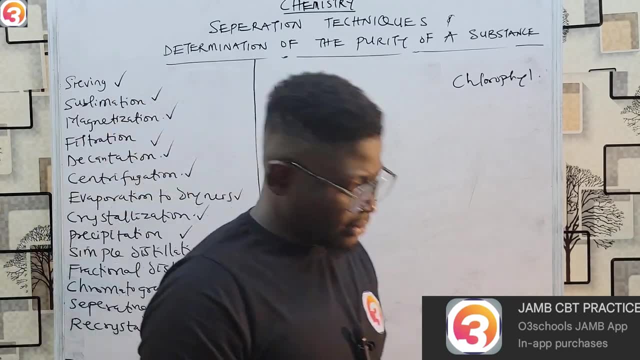 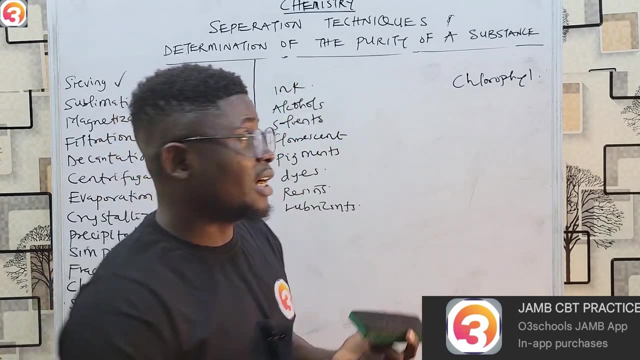 again. it has a lubricant. it has amazing dyes. they are even more more concentrate of what ink. ink is made up of a lot of things. right, so you can separate the concentrate of ink and chlorophyll using what? using chromatography, and what would i have said that? the major constraint of photography. 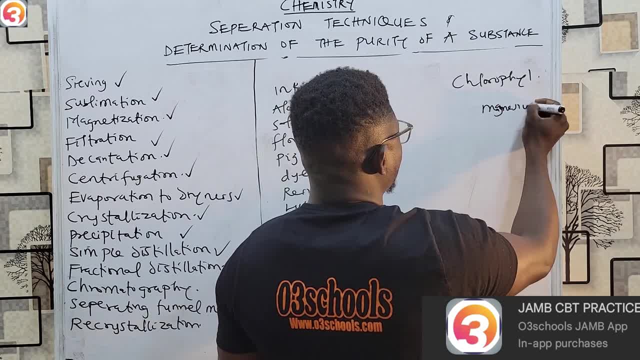 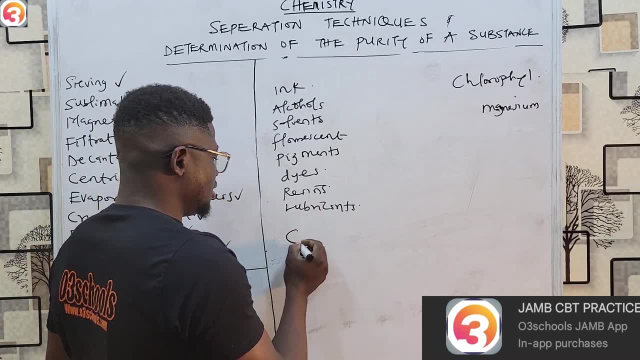 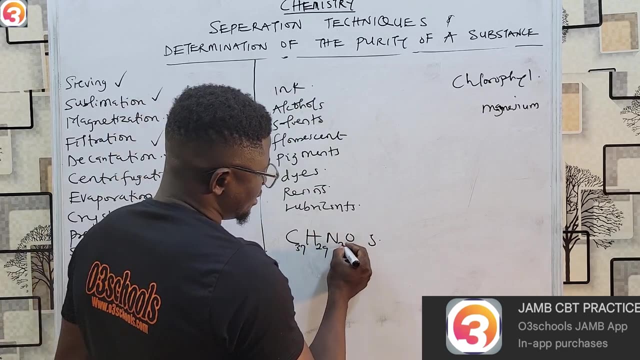 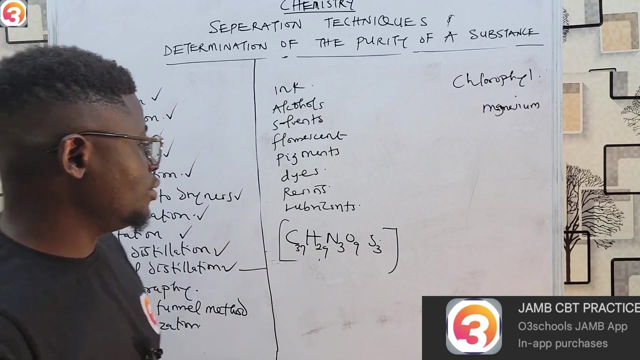 is what is magnesium? magnesium now, the chemical formula for ink, or ink, if essentially blue ink, is c37 h29 393. so this is what the chemical formula for what for ink right, c h n o s, 37, c37, h29, m3 o 9. 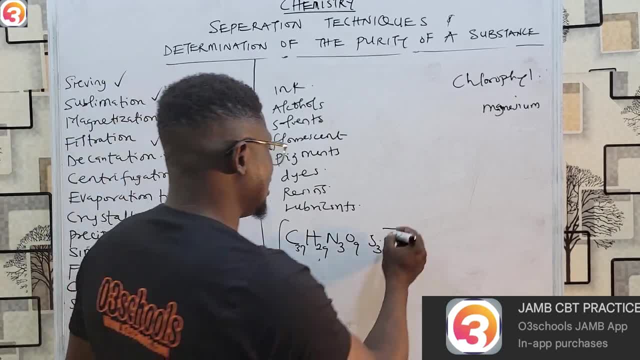 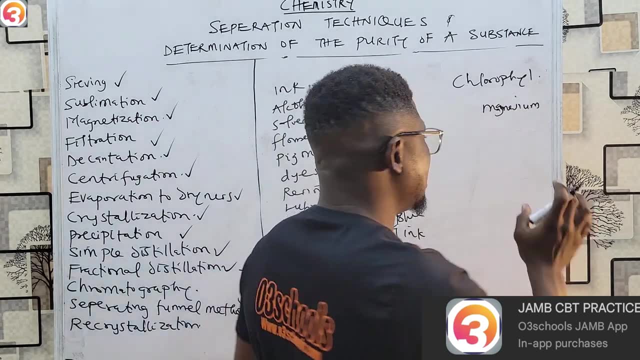 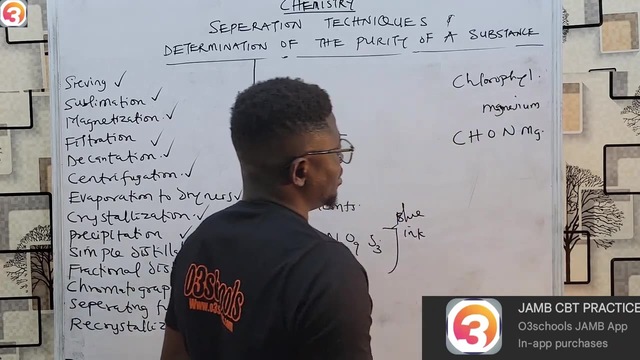 it's three. this is the chemical formula for inch for blue, ink for blue, increase this take note. and therefore for chlorophyll acid. the major content is: what is magnation on that? uh, c, h, o, n, n, g, right, this is the formula for what? for chlorophyll, and this is 55h72. this is 5, this is four, like this. 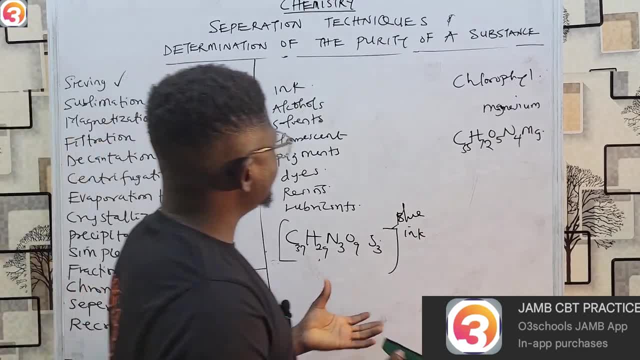 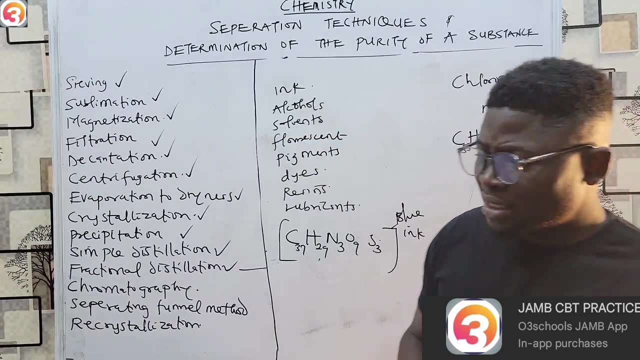 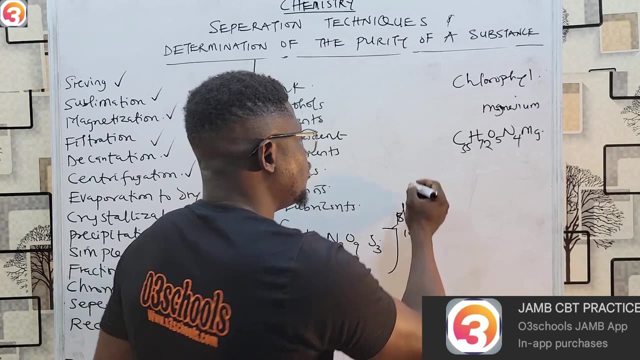 so this is the chemical formula for for chlorophyll right? so the constituents of both ink and can be separated using what? using chromatography. now know that what chromatography can also be useful. first, can both be used for separating colored and colorless substances, for both colored and what are colorless- colorless. 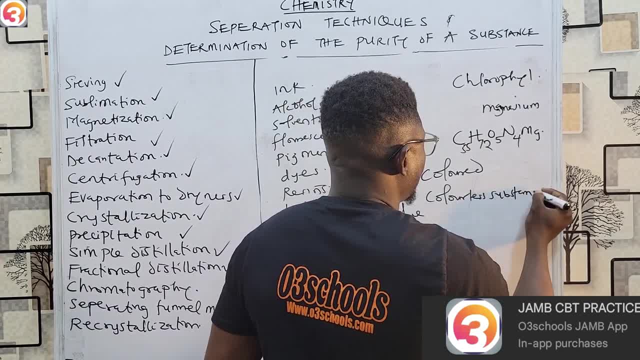 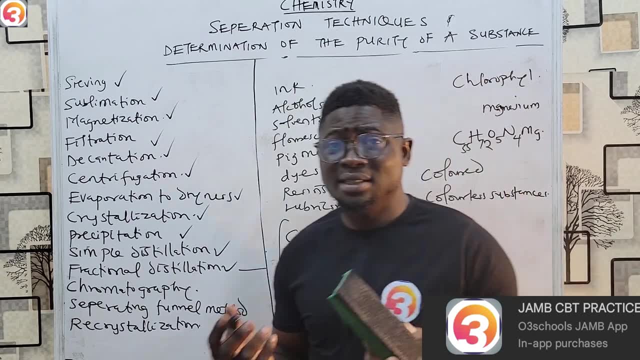 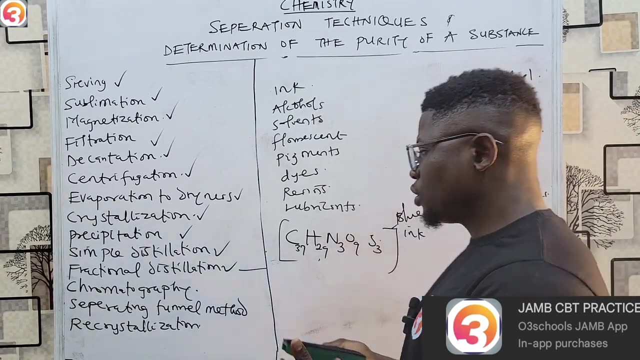 colorless substances. please take note. so whenever I hear about color, usually is what's going to be chromatography. so for as a patient, as a patient technique. so chromatography is both useful, separating color and what, and colorless substances. then of course we'll go to the next one, that is, what, separating. 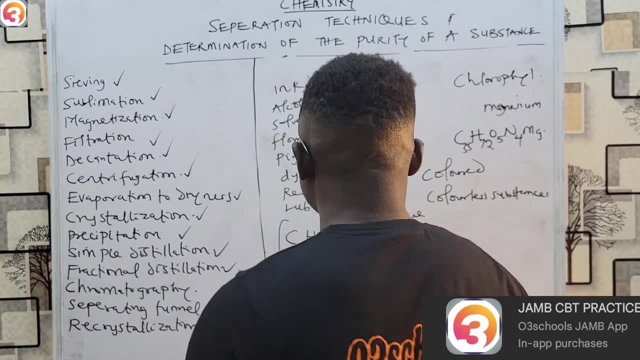 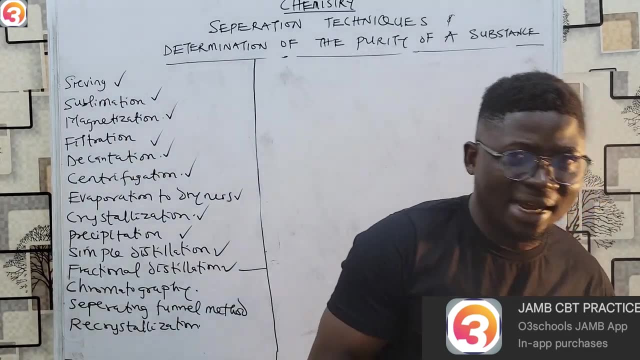 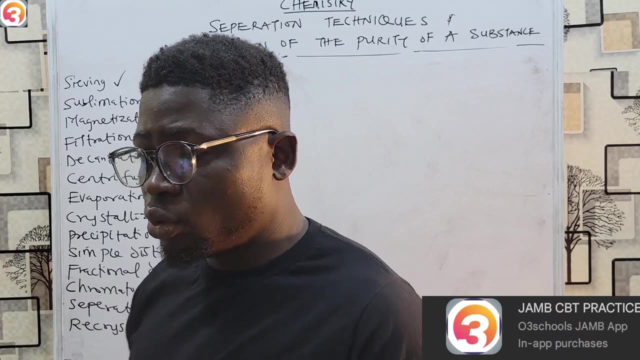 funnel method. separating funnel method is used for separating two immiscible liquids. two immiscible liquids, that is, two liquids that cannot mix together. right, like a water and oil. right, they cannot mix together. so you use what separating funnel method to do that? why the last separation technique. 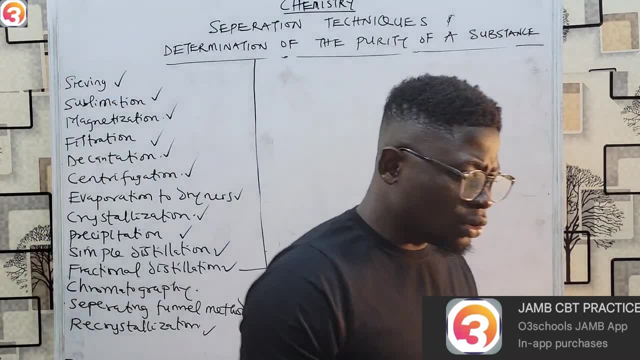 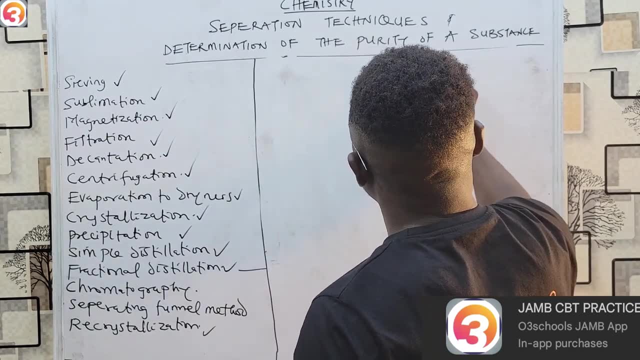 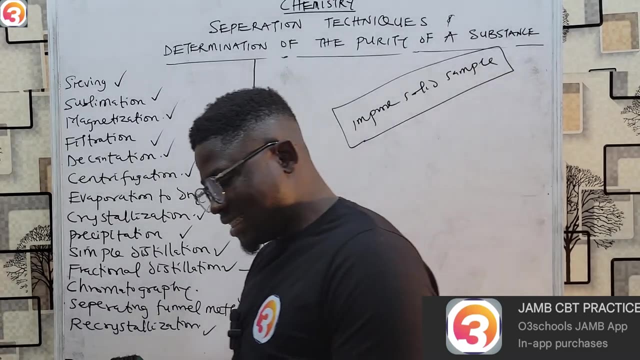 we are discussing is recrystallization. it's used to water to to purify an impure solid sample. so if you have an impure solid sample, you use water recrystallization was to purify or it. so that is the last separation technique. we are going to what discuss. 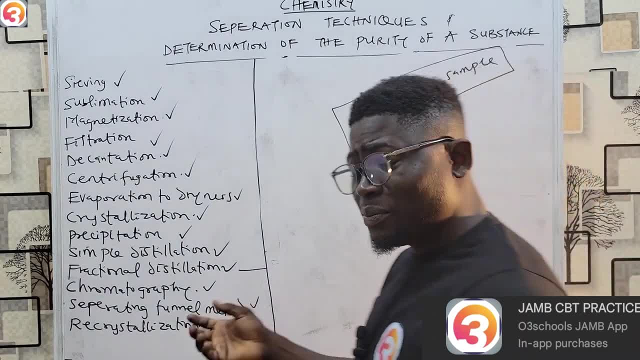 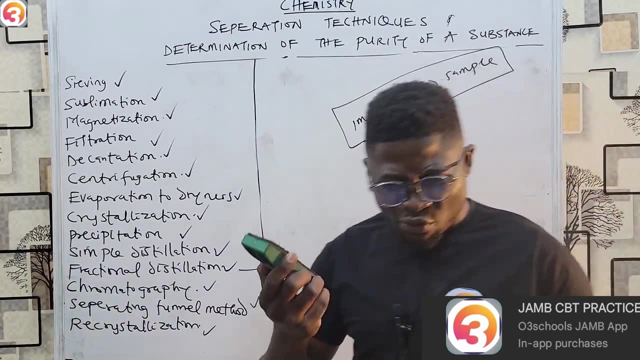 and, of course, with this we have learnt about all the separation techniques that are available, and then we can. we are ready, we are bruised up for what? for the going up, so we could have a dry p осв da for for this class to the last part of. 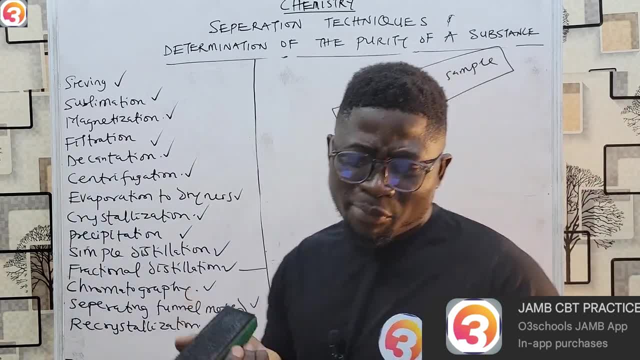 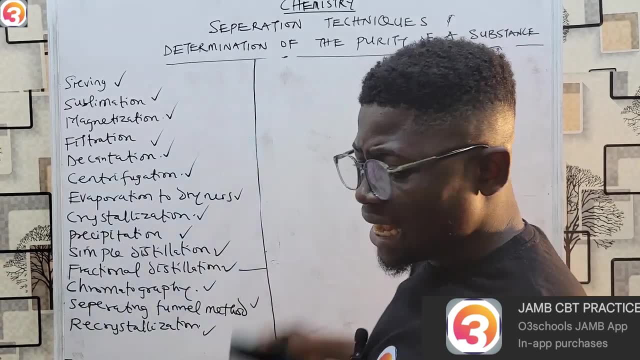 what this class determination, the purity auf so pass. how do we know that is somethings with this? pure as so, there are different due forms, so let's go to our practice q plus, and then, by the way, I can be here today and you can actually. 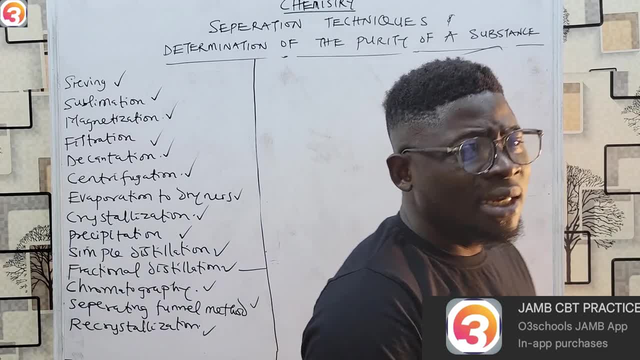 also do answer my question. in one of my six questions you have one that will give you a little bit more detail. look at this question is? it at least establishes what this practice is? and we move on to the last part of our tuitions, to the last. 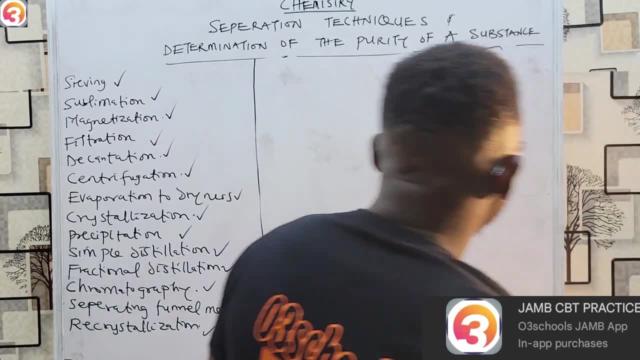 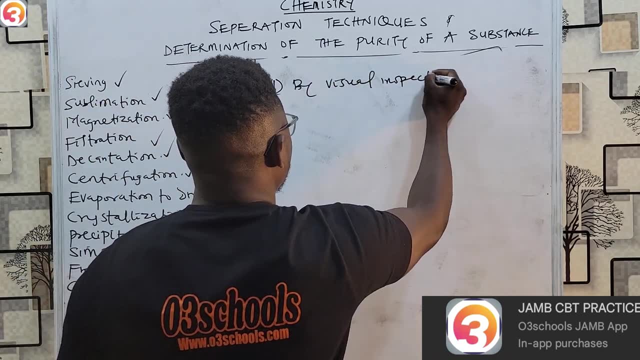 part of this class, because i will replace the inter meaning to some of the words: an order country. our subject is: where is the without here? and so there are different techniques and methods we use. one is what? by visual inspection. by visual inspection, so you have your eyes right, you can see. sometimes you see something that is 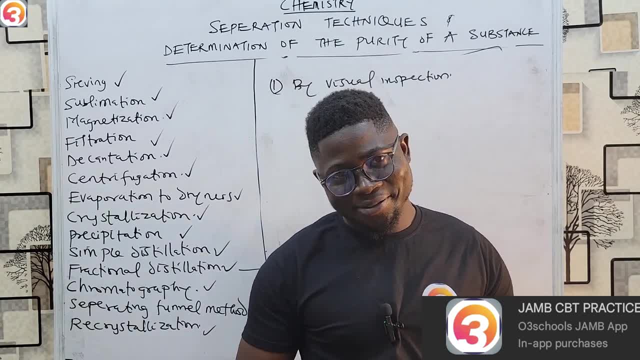 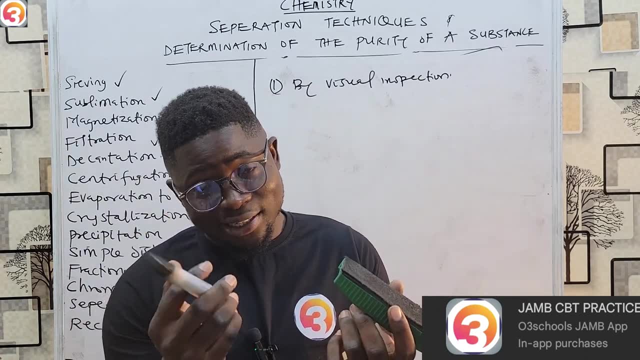 dirty. you say: ah, okay, how do you know that somebody's wearing a dirty cloth? answer: right. so you're learning from your eyes so that, ah, this, this is supposed to be white, but you don't. they turn to brown even that. he, that's all, yeah. if you go to a mechanical shop, you see different. 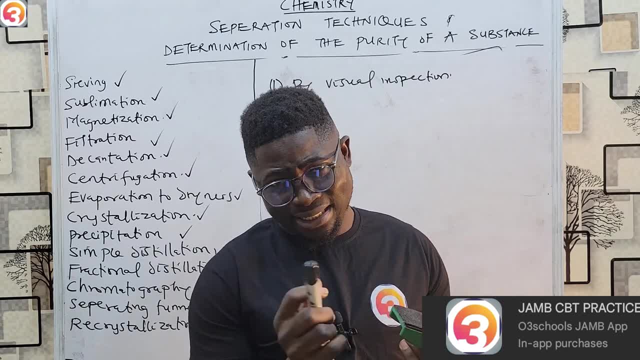 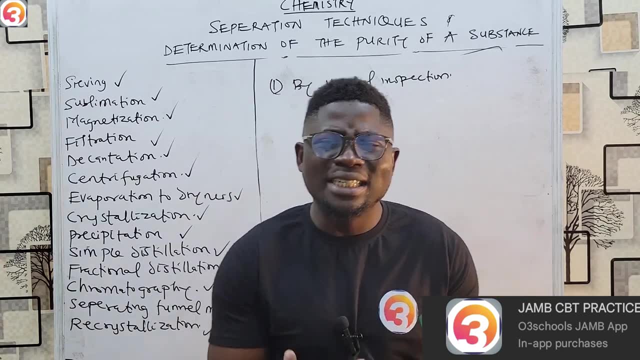 things on the body. you know that. that's that man is wearing. his death is very, very dead. of course that is the nature of his job, and so i'm just trying to raise that by inspection. so you look at what the color, look at the appearance of what of the substance of interest, and you know that. 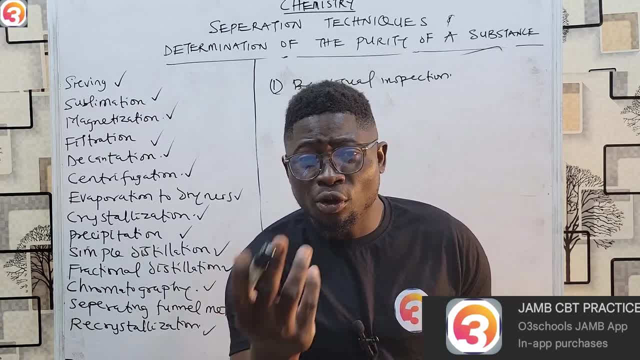 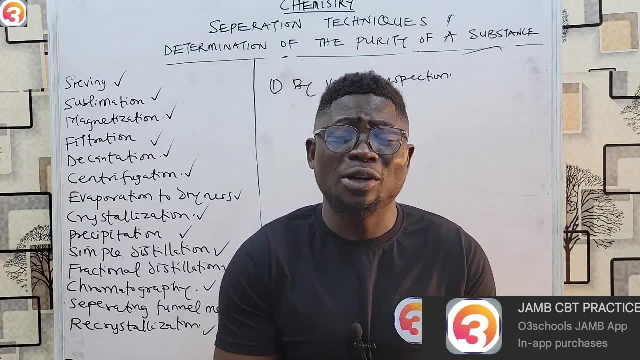 what this material is clean, whether it's pure or it's not pure. so if you look at the substance by the, by the color, by the, by the, by the appearance, you can know that what it is, what it is, pure or not right. so that's by. 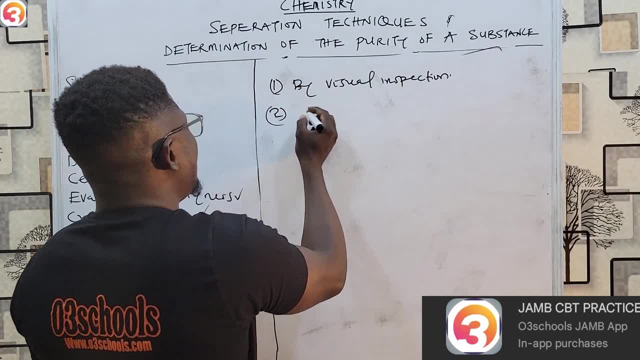 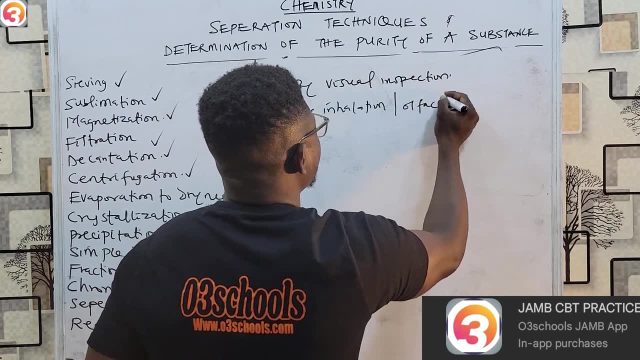 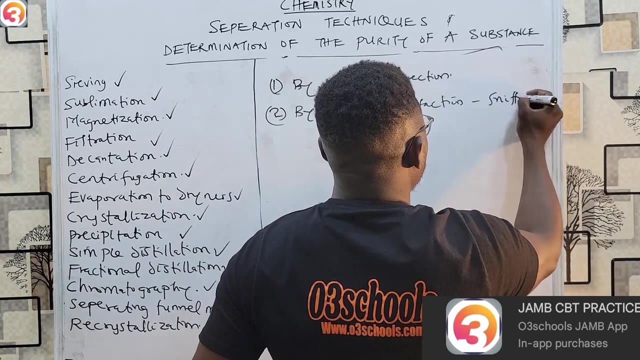 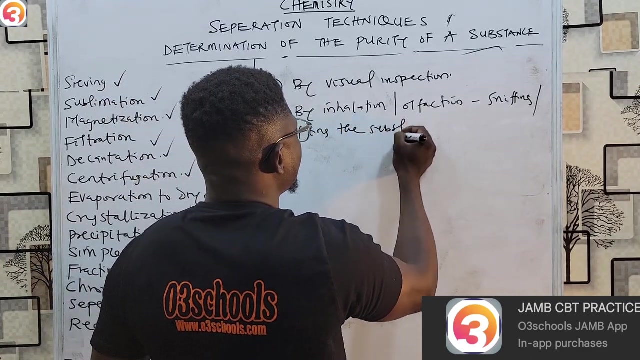 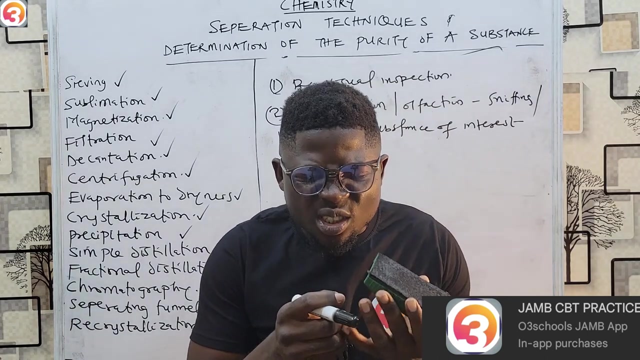 what? by visual inspection. then number two, we have what? by inhalation. inhalation or olfaction, right. so this is what done by what? by sniffing. by sniffing or wafting, watching the word: the substance of interest. so you take all the substance of interest close to you, you sniff it. 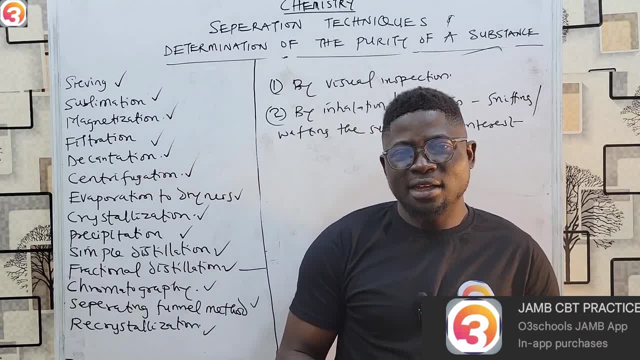 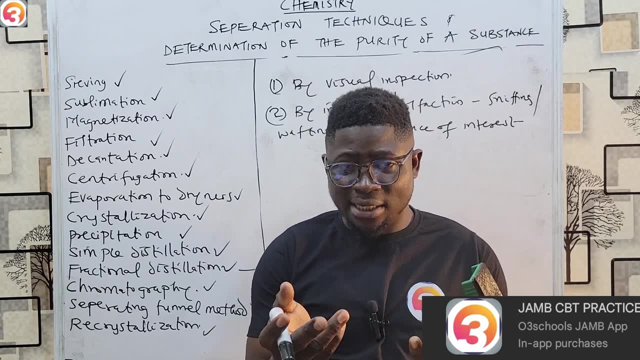 ah, no, no, no, no. you think that they spoil, right. so you have a substance. if you sniff it by the smell that comes from it, you know that what it is, what pure or not, it's getting bad or not right. so sometimes they may what they may be odorless when pure, why some may have characteristic what? 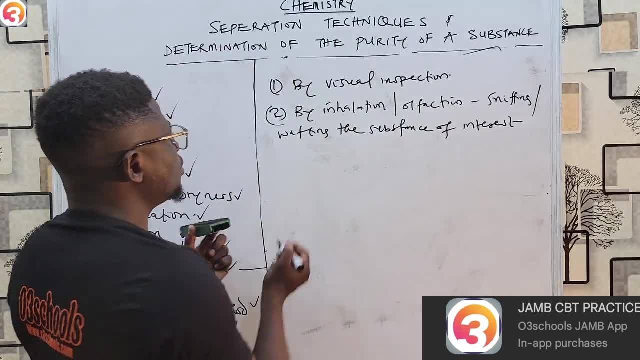 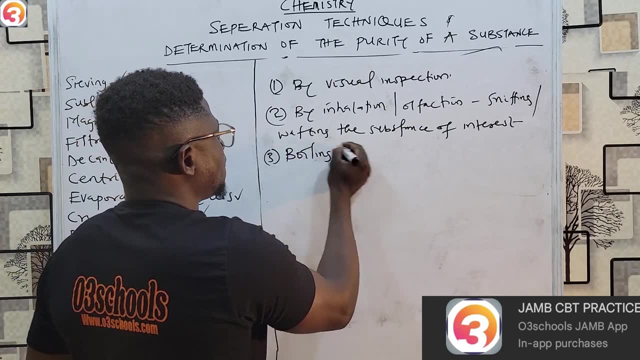 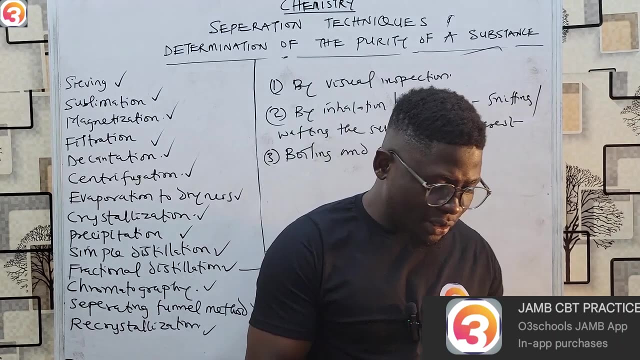 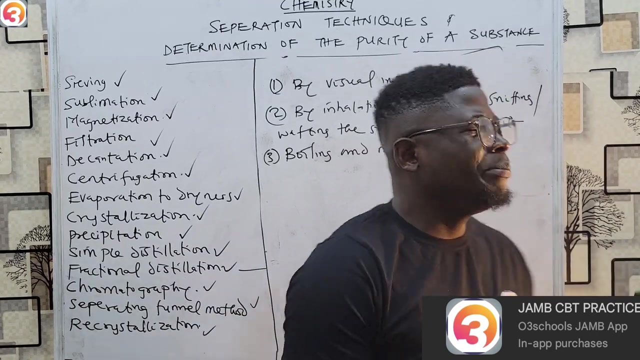 would also. you have to take note of what of that. then, number three, we have what uh uh, boiling and melting points and melting points determination. so for boiling and melting point determination is it is by far the most used right for the determination of the purity of a substance. 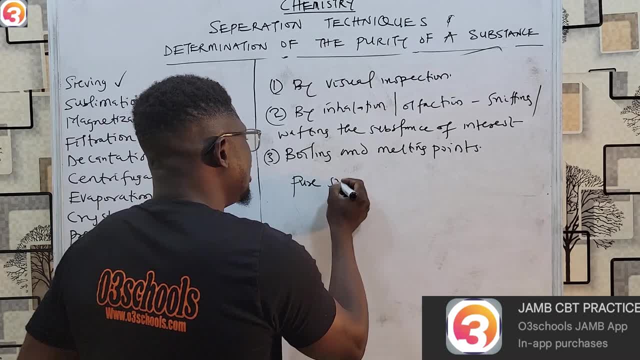 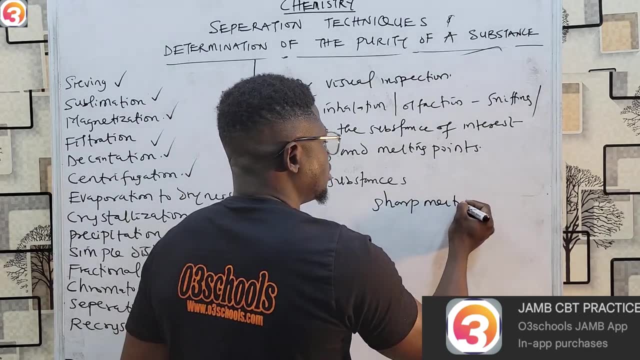 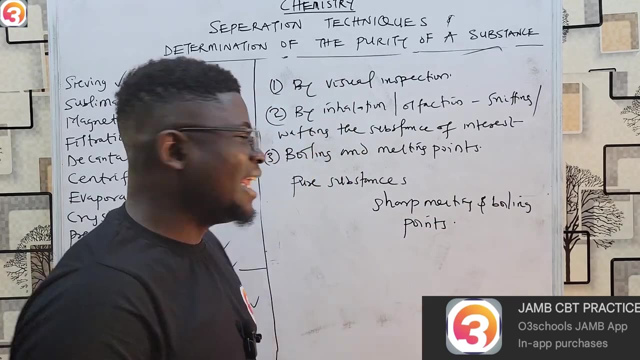 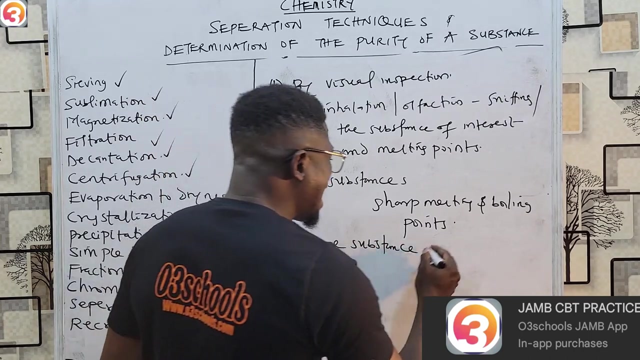 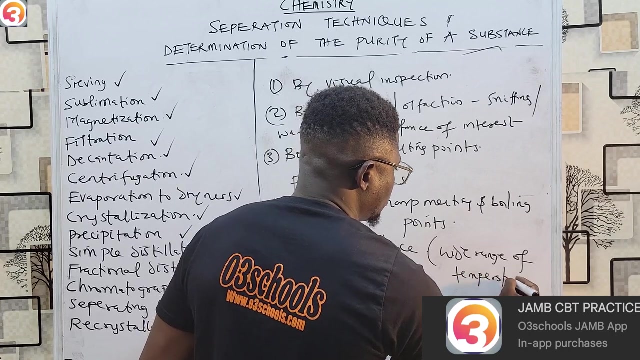 pure substances have sharp melting and boiling points. pure substances have what? sharp melting, melting and boiling points. and boiling points: right. why impure substances? impure substances boil at a wide range. wide range of what? of temperature? right? so of course pure substances have sharp. we have to take note that pure substances have sharp. 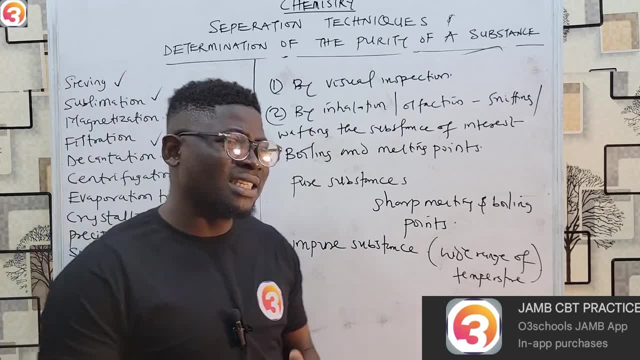 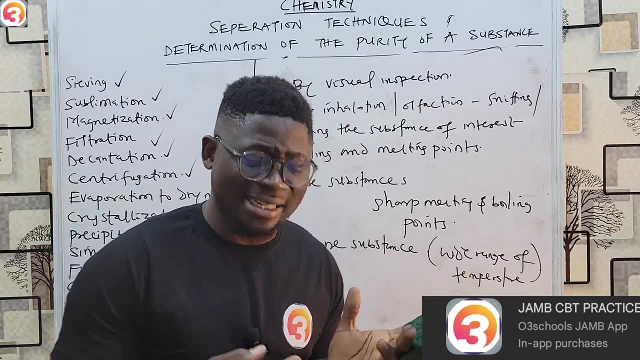 melting and boiling points right, and then impure substances may boil over a wide range of what of temperature. so if you sometimes have a sharp metal body point, you can tell that what this substance is, what is pure? but of course it has. it starts boiling over a wide range of temperature. 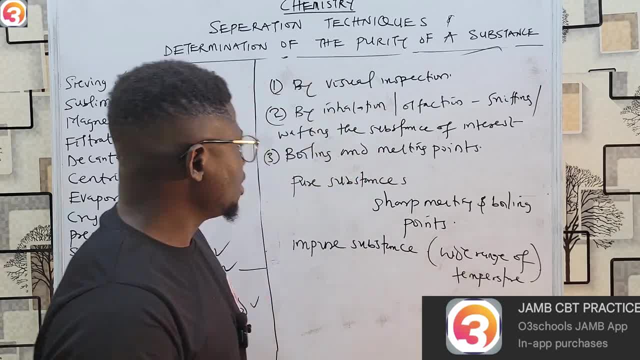 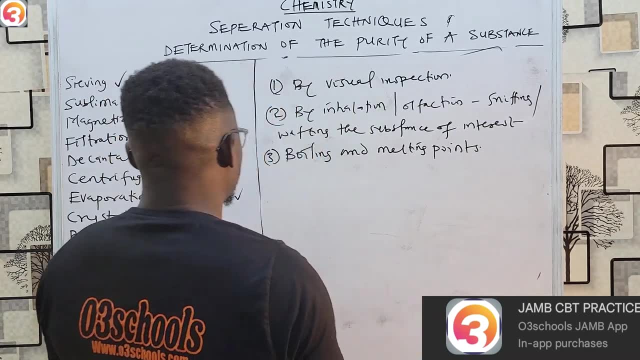 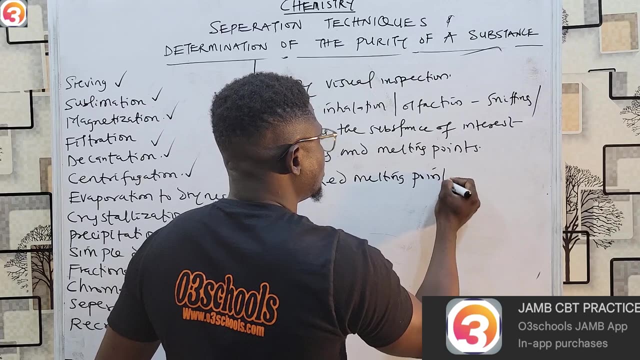 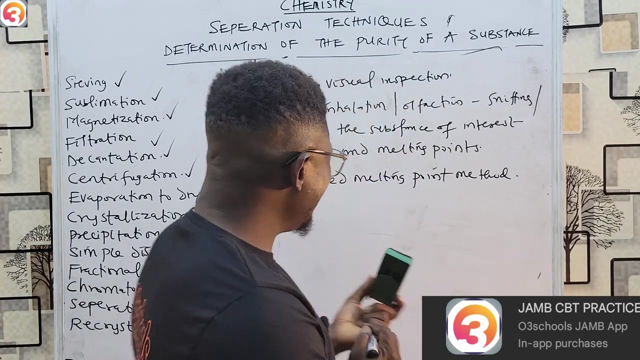 not that, what that it is impure, all right, so take note of that. that is number three, then number four: we have what you call the mixed mixing point method. before we have the mixed medicine point method, the mixed methane point method. so in this one you are taking a sample. 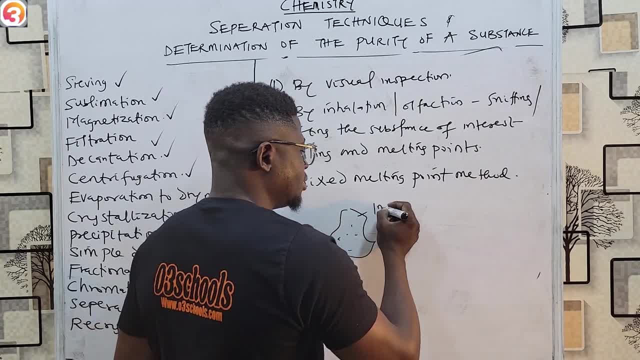 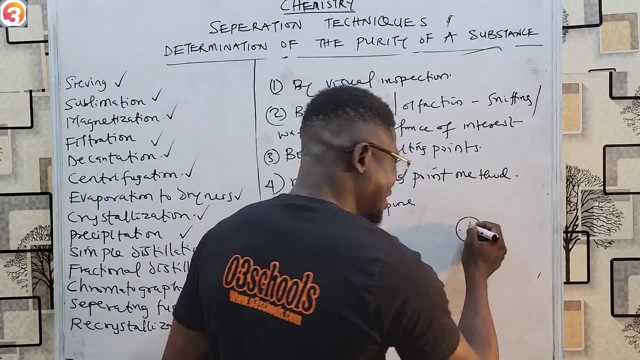 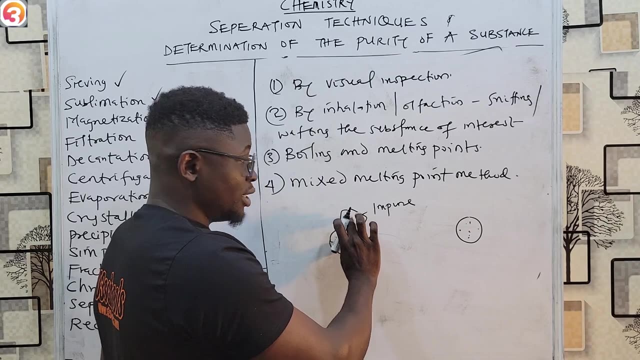 so let's say, with this sample now is what is the impure one? and then what you take? you take a pure sample. you take a pure sample of what that's a substance, of this, what this substance. we want to determine whether it is pure or not. so you take this, you don't know. you don't know about this one, you don't know whether 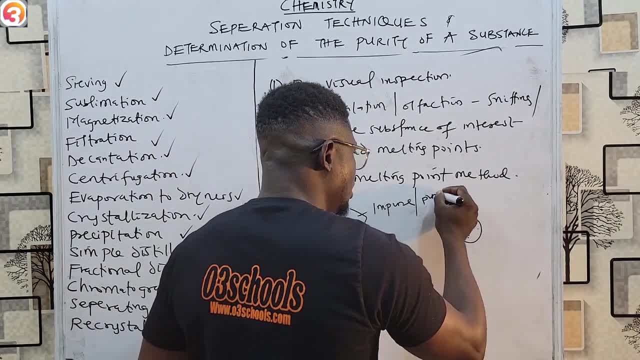 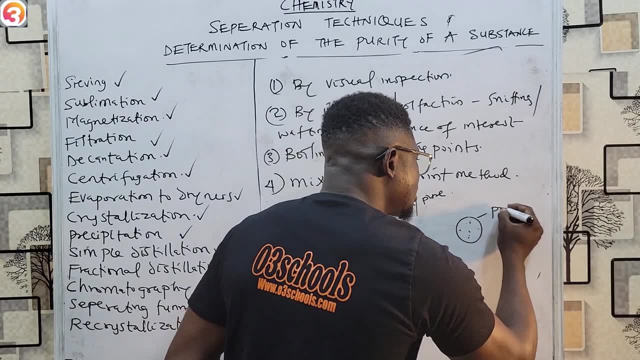 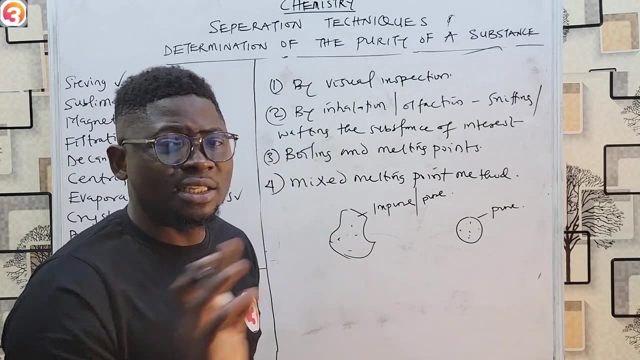 it is impure or not, right, impure or pure. so let me put it this way: this substance, we want to determine the purity. you don't know that it's pure or impure yet. so what you do? you take a pure sample of the same substance and what and mix them together. so if they have a sharp melting point, 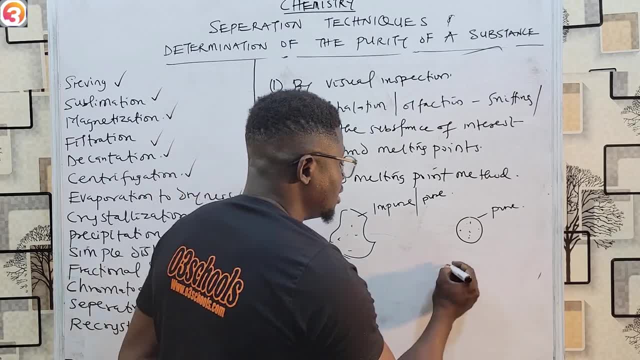 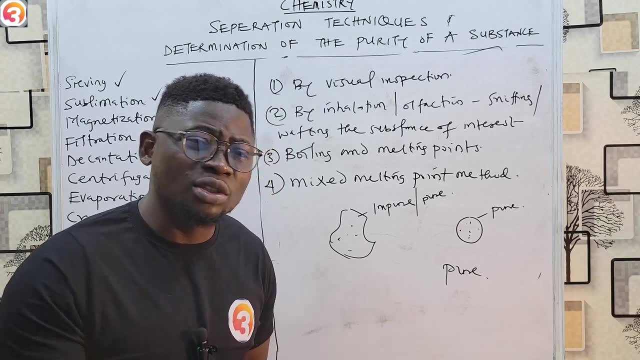 right. if they have a sharp melting point, you know that, what the substance is, what, what is pure. but once you mix them together and then you see that they have what, and they start having what a wide range of what temperatures, then you know that what it is, what it is impure. 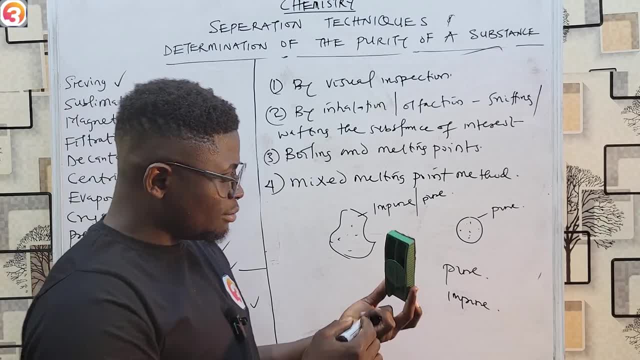 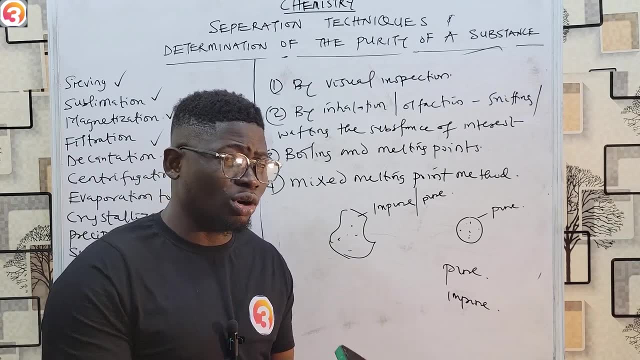 so that is what called the what the mixed melting point metal. you take a pure sample of the substance. you want to determine the purity and add it to the work example that you are not sure of whether it is pure or not, and then you use them to know whether it is pure or impure, whether, if 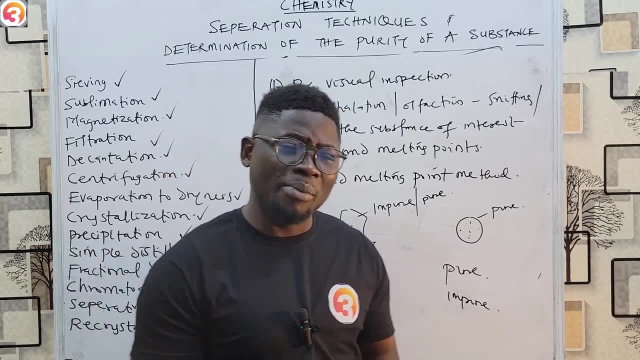 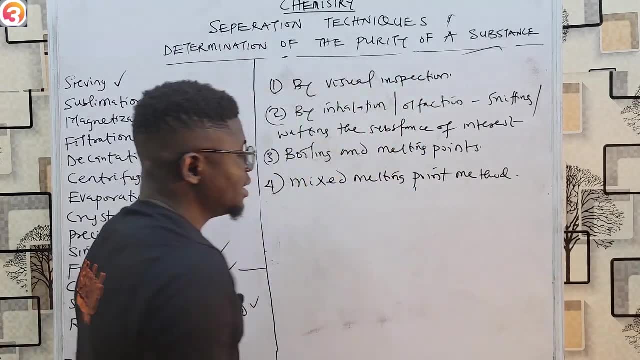 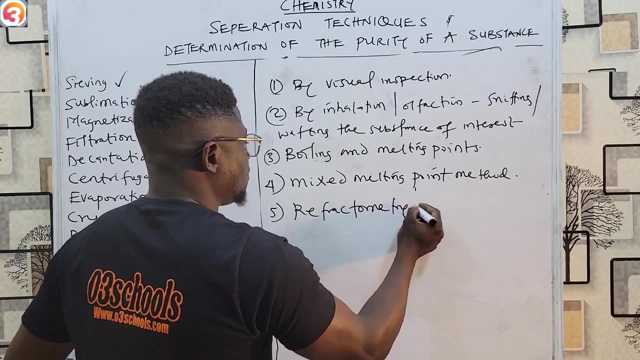 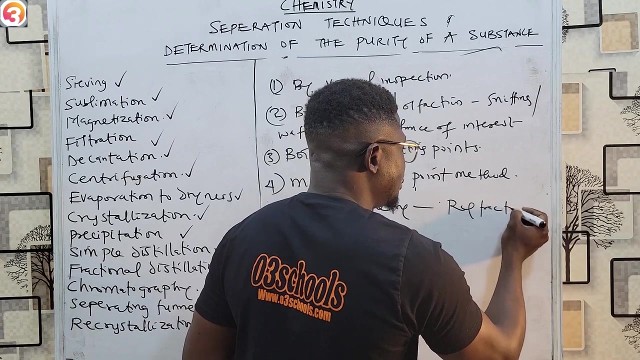 they have what sharp melting and boiling point, or if they would boil or melt over a wide temperature range. so that is that. for what mixed melting point metal? the last one. the last one is called refractometry. refractometry, in this case, you are using a refractometer. use a refractometer. 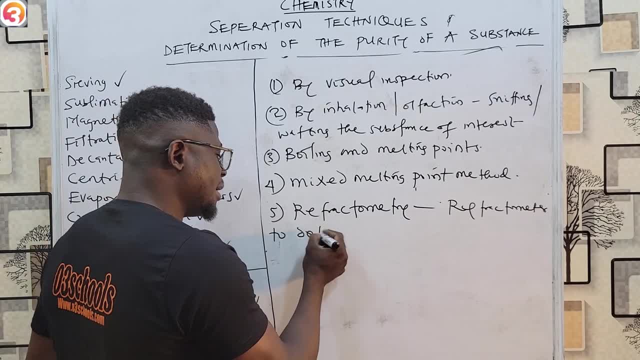 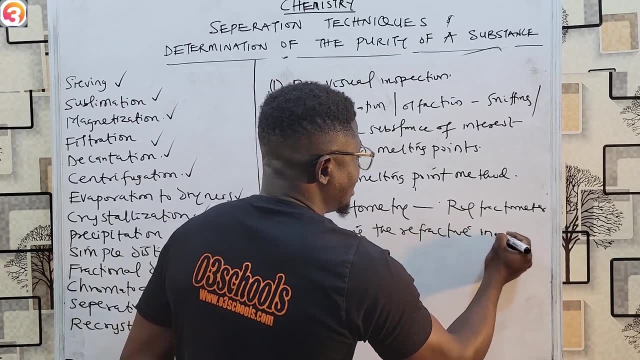 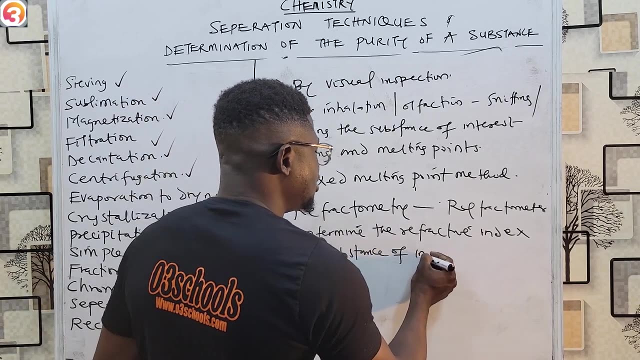 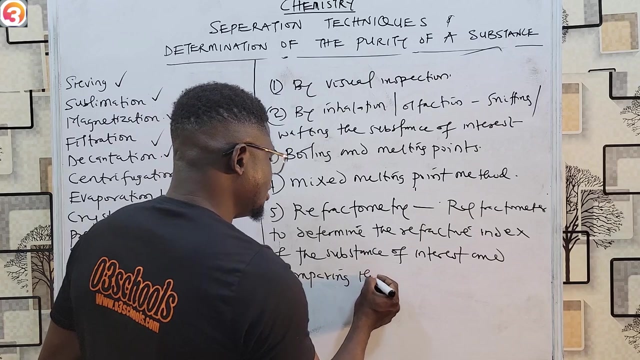 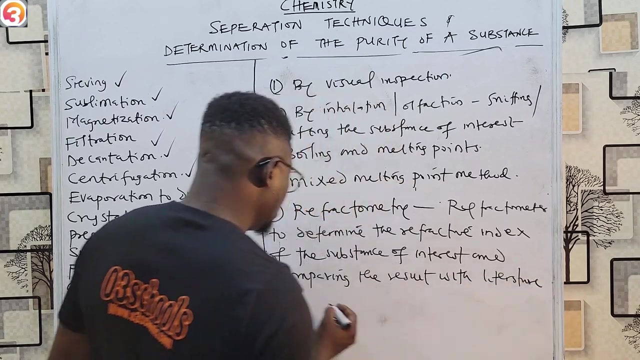 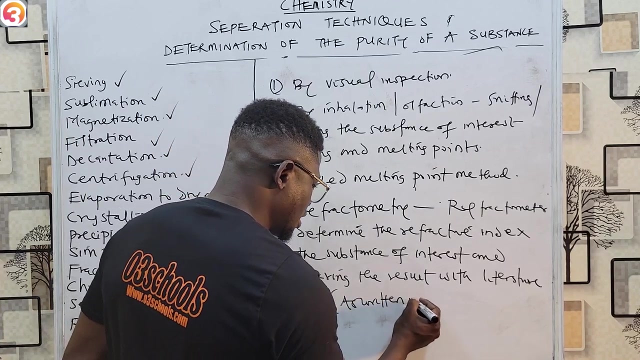 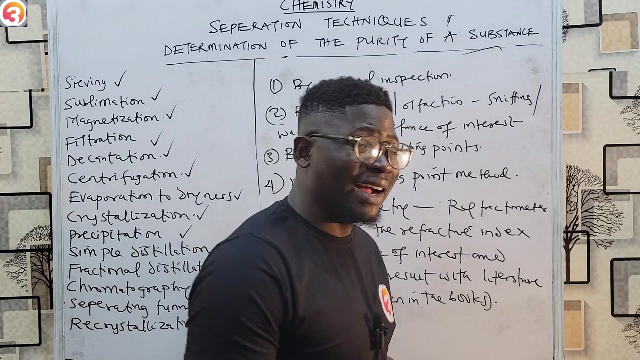 to determine the refractive, and that's to determine the refractive refractive index of the substance of what interest, and comparing the results. comparing the results with what? with literature, literature values. literature values are talking about as written in the books, so of course there are some books that have what they have. what values for what? for something that 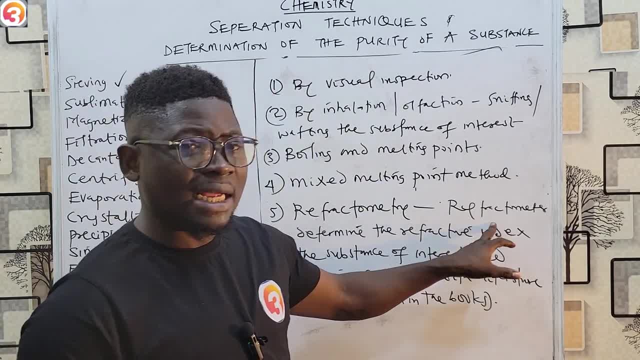 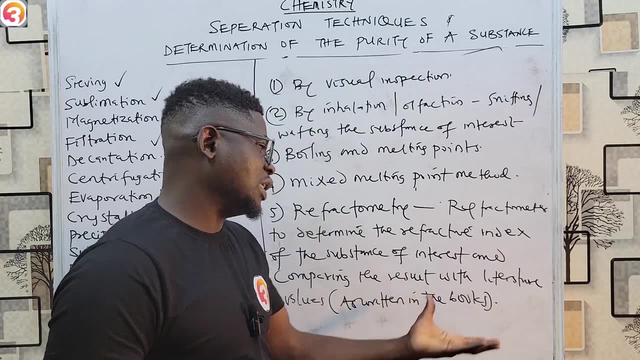 are pure right. so what you do? you take a refractometer to determine what the effective index of the substance of interest, and then you compare the results you are having with what? with the known literature values or as written down in the books. interesting class, you may say.